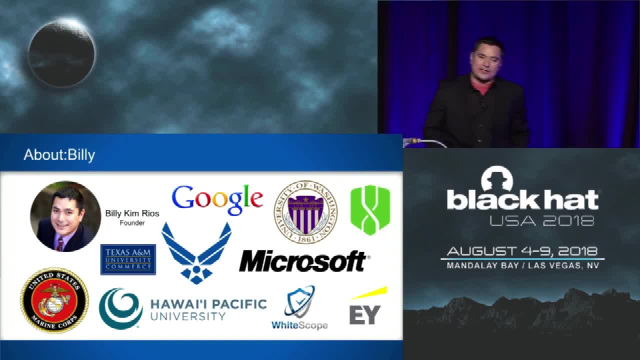 be on the engineering side. I was at Microsoft for a little while. I was at Microsoft for a little while, And I was at Microsoft for a little while. And I was at Microsoft for a little while. I ran security for Internet Explorer, So I definitely know what it's like to wake up. 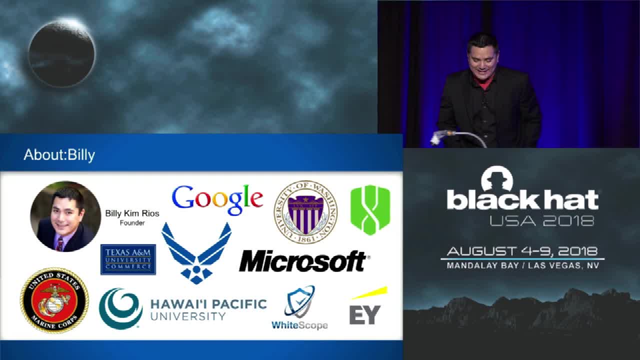 one day and find your product on CNN Not in a good way. But medical device is actually a passion of ours. We've done a lot of work in medical device in the medical device community And that's actually how we got started kind of working on systems together. 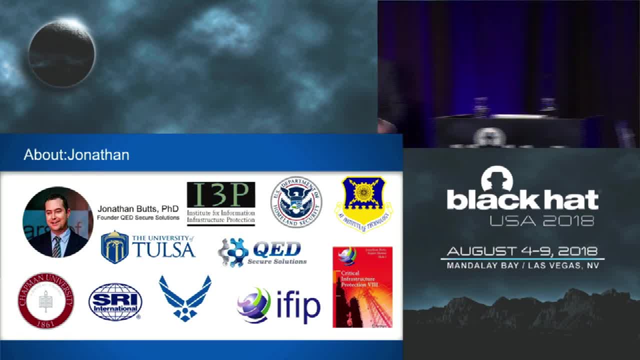 And, as I mentioned, I'm Jonathan Butts, And one of the things I'd like to highlight is I retired from the Air Force. I was a professor at their graduate school, And so when we talk about research- cybersecurity research- we actually make sure we put a lot of effort into 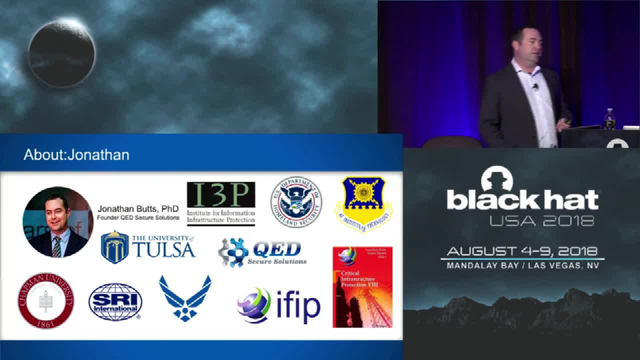 that We put that vigor, that academic background and vigor in it. So we're actually doing it from an experimental standpoint And so when we provide the results either to vendors or other folks, we want to make sure that it's sound and repeatable, to follow those research principles. 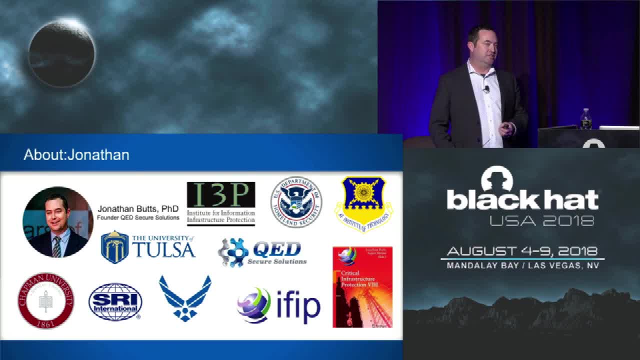 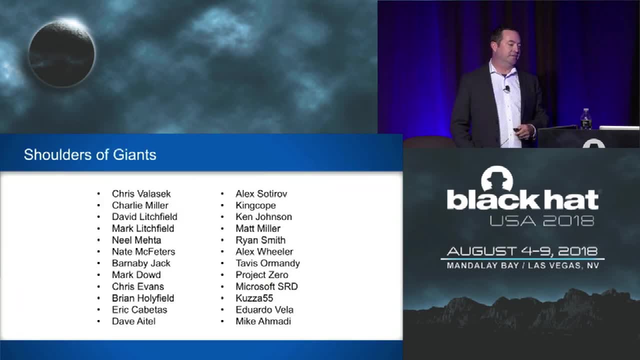 And I think that's important for what we go through here as we present today. These aren't just things we discovered and said, hey, this sounds interesting, We're going to draw these conclusions. These are actually. we follow a very strict methodology. 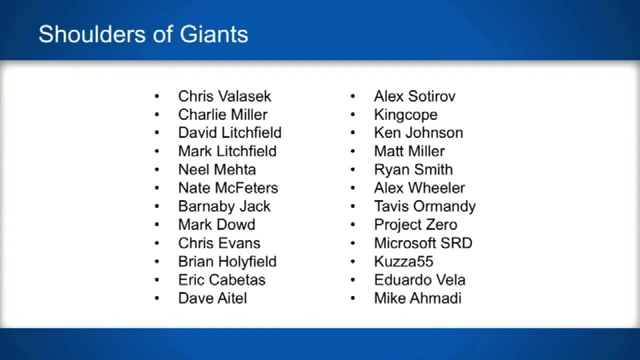 Yeah, Hey, there's a man been doing been doing cybersecurity for a long time, Even when everyone hated that word cyber, but it seems like everyone's using it now. But there's a lot of folks who may not do like device security or something like that, but have definitely 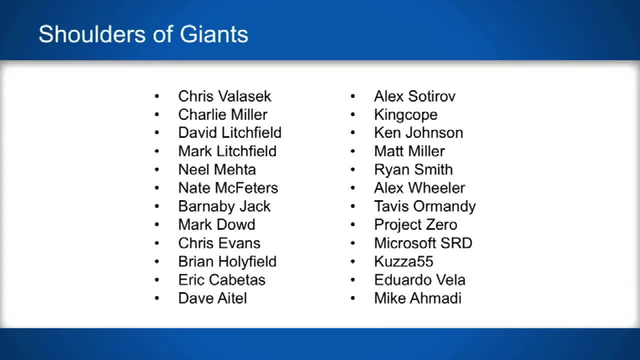 influenced the way that we look at problems, right. So I mean, I'm sure I'm forgetting someone here. If you think you should be on this slide, definitely let me know. But we definitely wanted to take some time to recognize a lot of different folks in the industry. And then the next slide. 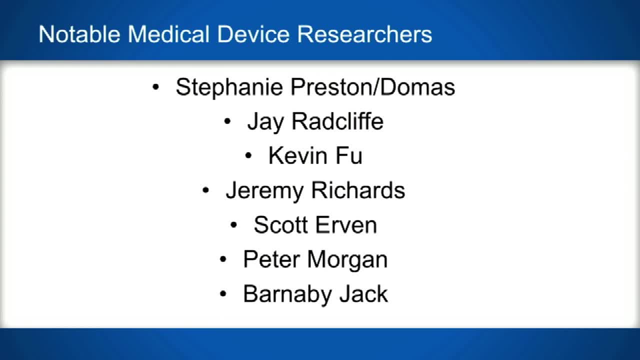 actually talks about, specifically like medical device researchers. So if this slide makes its way to the public and someone's interested in like, hey, I want to know some folks who are actually doing medical device stuff. This is a list of some really good folks on here. 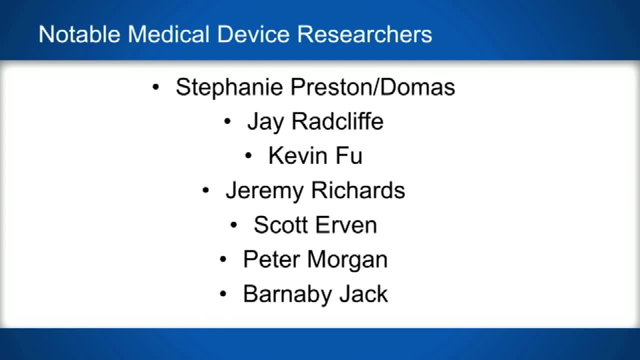 Stephanie, Jay, Kevin, Jeremy Richards, Scott, Peter Morgan and Barnaby Man. that guy was like light years ahead of his time, right. So I think some of this, some of the stuff that we're going to do today, may actually even overlap with some of the stuff he did in the past. We'll talk a little. 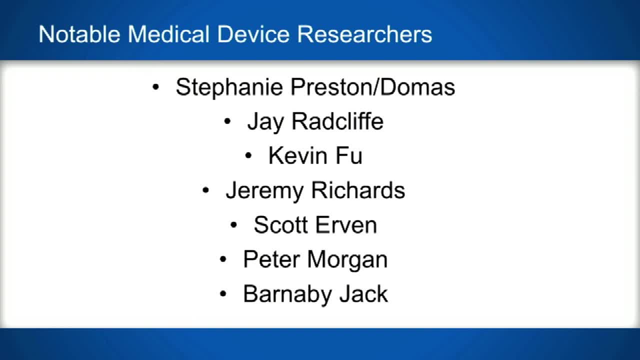 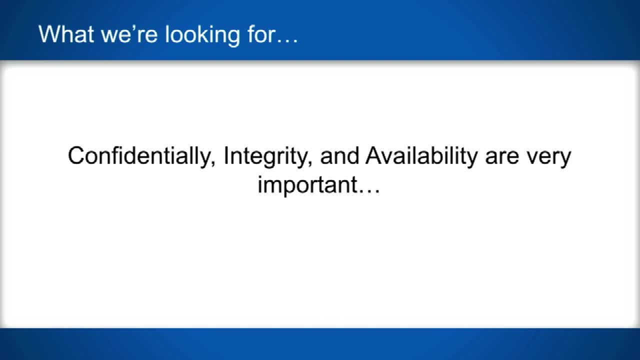 bit more about that here in a second, But the guy that that, the work that that guy's done is just amazing. So All right. So when we talk about vulnerability- so you know we talked about patient safety- We want to make sure that we call it a very important distinction between what we 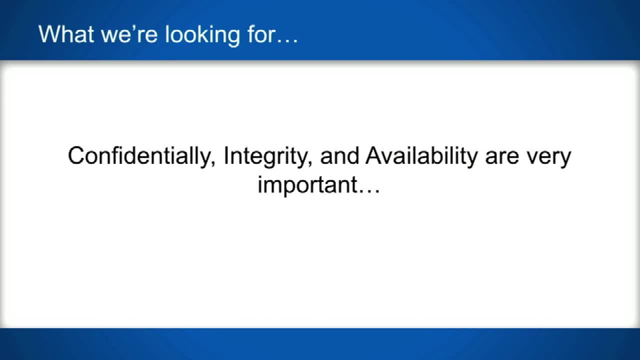 see on traditional information technology systems, your traditional IT systems. A lot of times you put that in the context of your information assurance principles. the triad- confidentiality, integrity, availability- That's all fine and dandy, But when we're talking about medical devices, 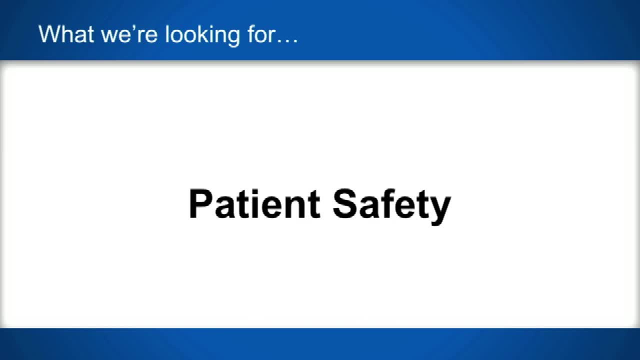 really what we're interested in is patient safety. How does this vulnerability that we find does that impact the delivery of patient therapy? And that's really the important question. That's the question we should be asking is: does this impact patient therapy at all? 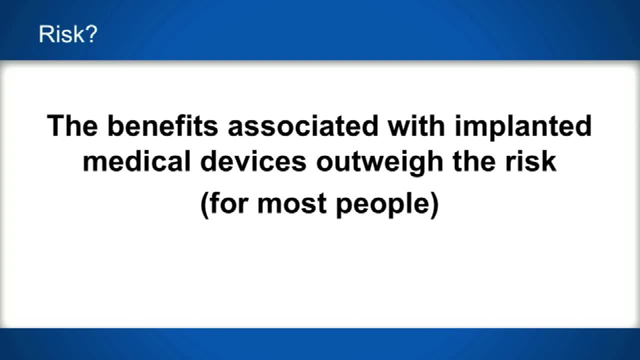 So, from this standpoint, one thing we do want to call out is: we're not physicians, We are cybersecurity researchers, And so our role is to present the findings from a device level and not to make the call on whether or not it's a risk to a patient, on whether or not they should or should. 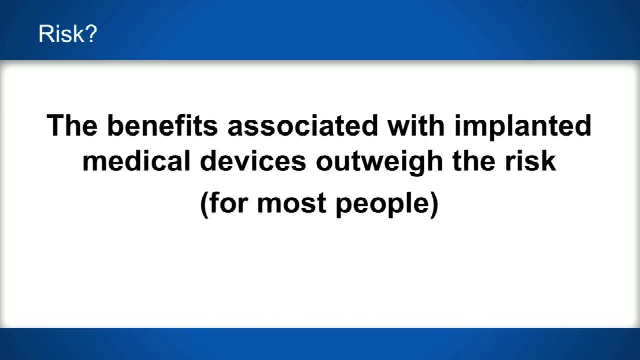 not be using this device. That's up to the physician and discussions with the physicians, as well as integration with FDA to start making those calls And I think too often you cyber researchers will kind of reach on that. So from this standpoint, our point of view is the benefits with implanted devices. 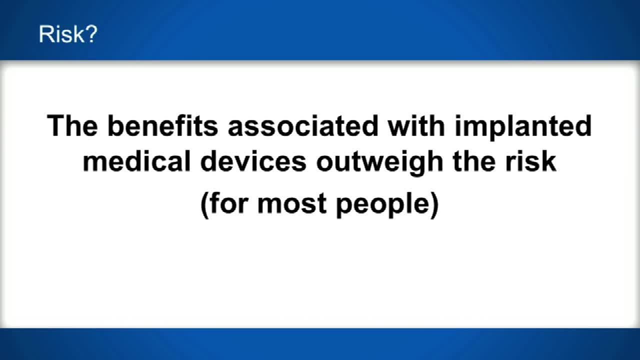 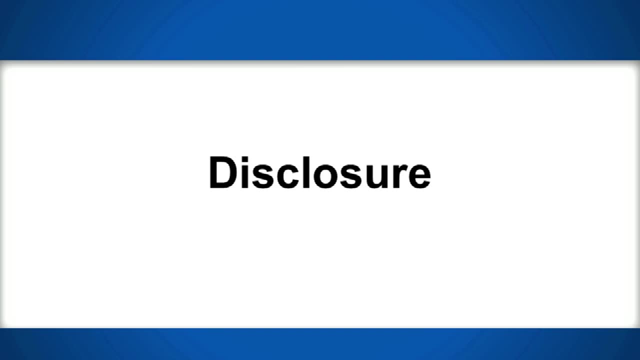 they're used to save lives, And so, at this point, we still believe that the risk of not having it is it's better to have the medical device, because it outweighs the risk of the cybersecurity aspect, Definitely. With that said, there are cybersecurity vulnerabilities in a lot of. 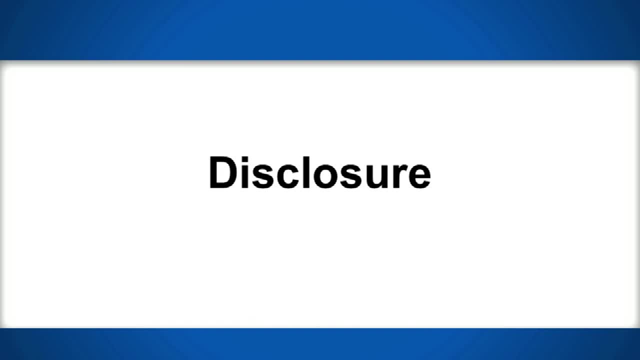 different products, right? So that's just a fact of life. We all have to deal with that, And so that's something that I think we can change anytime soon. However, the way that we deal with those issues is something that we can control, So we're going to spend the first part of this talk 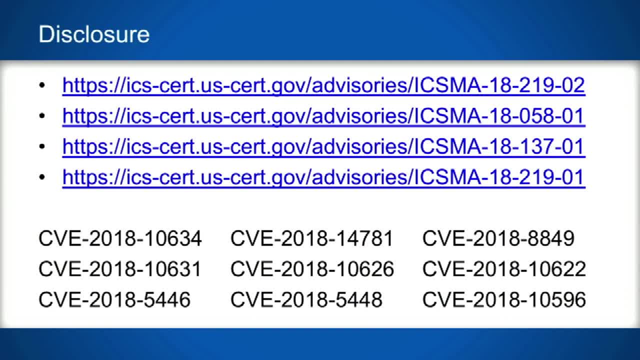 talking a little bit about disclosure. This is not something- this is not research- that we did yesterday, right? It's not like we just discovered this stuff yesterday and then just decided to come present here. This has been a long journey for us, A lot of this journey that we've been going. 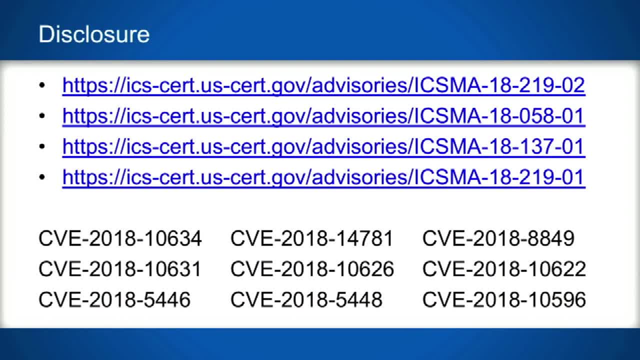 down over the last 18,, 20 months is captured in these four ICS cert advisories. Those are advisories from DHS. There's the links to them And then you know, we're going to have a lot of things that we're going to be talking about. So we're going to have a lot of things that we're going to. 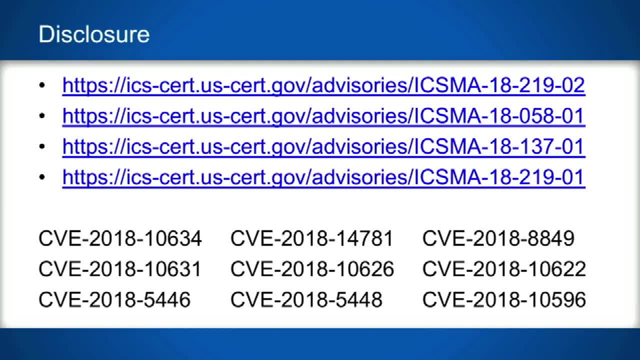 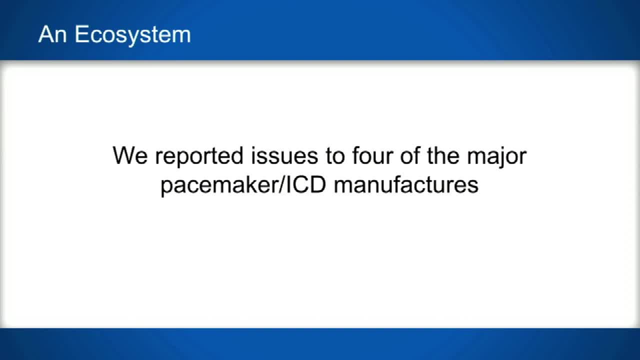 be talking about And then really are captured by these nine CVEs. So if you want to reference these or look up public information about this, it's captured in these documents, And so the research we've done: we found vulnerabilities or security concerns in four of the. 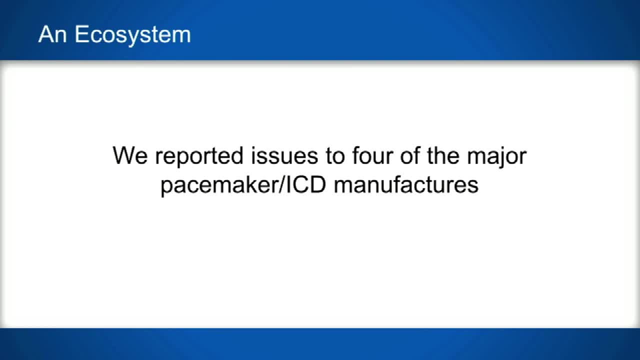 major manufacturers of ICD or pacemaker devices, implantable devices, And so we reported those to the major vendors. What was interesting for us is there was one manufacturer that actually was very difficult to work with. Now, Billy and I have been doing this for a long time. We've been 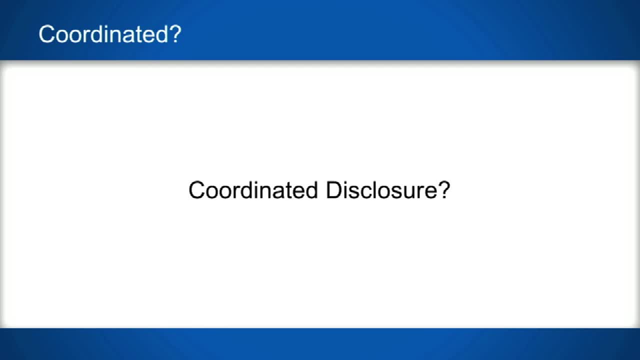 doing this for a long time. We have together probably over 500 advisories that we've reported through ICS, cert and worked with vendors And for the most part vendors are cooperative right. They see you as free QC QA And they'll work with you And we're patient with vendors from that. 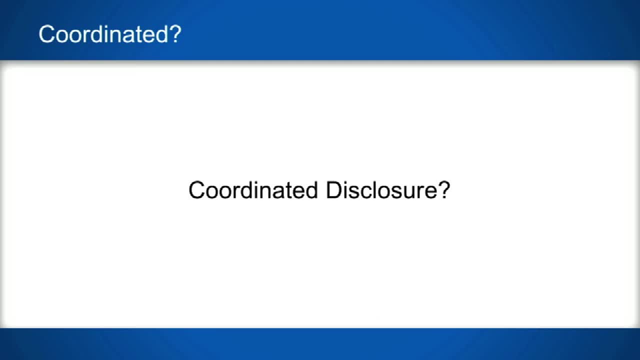 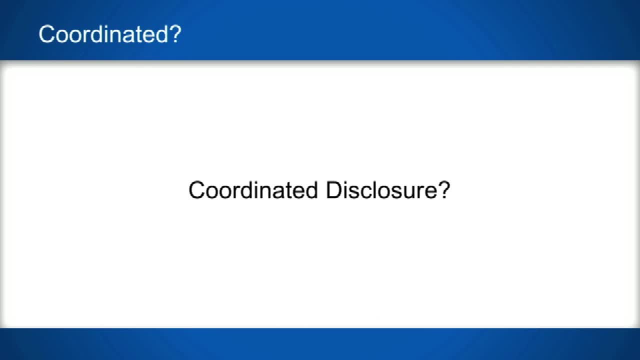 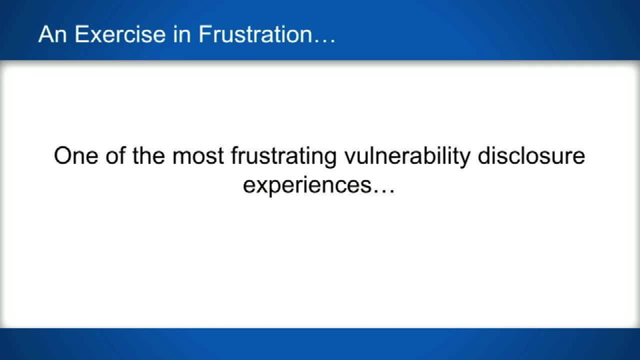 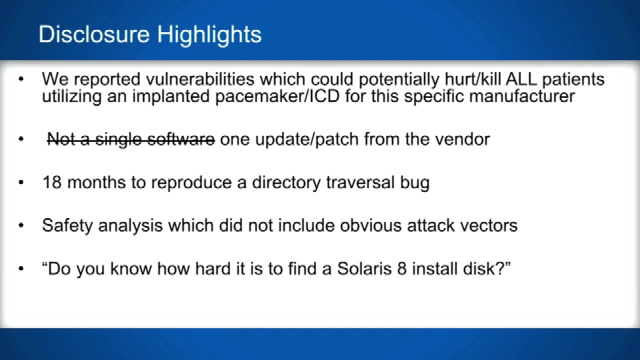 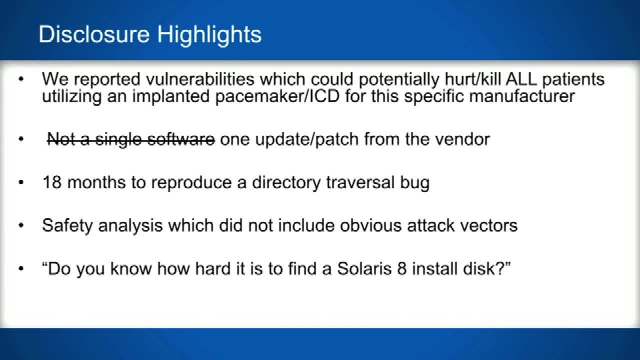 We- hopefully reasonably- would expect that a manufacturer that we give research to where the potential is that high, would probably take that seriously, right? I think they have a responsibility to take that seriously. As of this moment, we found out that there's actually one patch from the vendor. 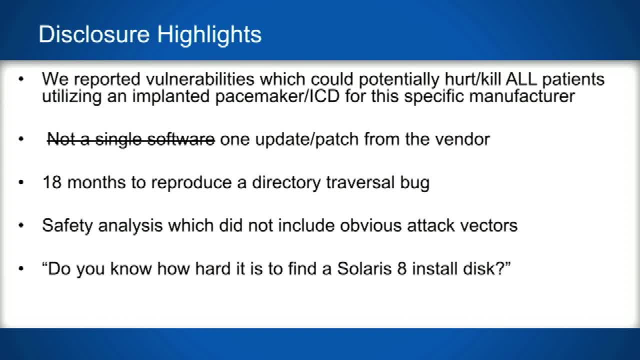 It actually has nothing to do with patient safety, which is kind of disappointing. More about data. We'll talk about that one here in a second. Some of the issues that we report to them, like a directory traversal bug in their update infrastructure, took 18 months to reproduce. 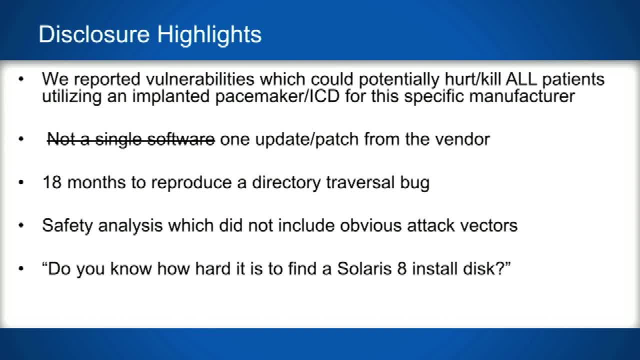 So we gave them a report that outlined a number of bugs, all kind of stemming on, like a web directory traversal vulnerability, like 18 months for them to say we finally reproduced it in our environment, right? So that's unacceptable. The safety analysis didn't include some pretty obvious vectors. 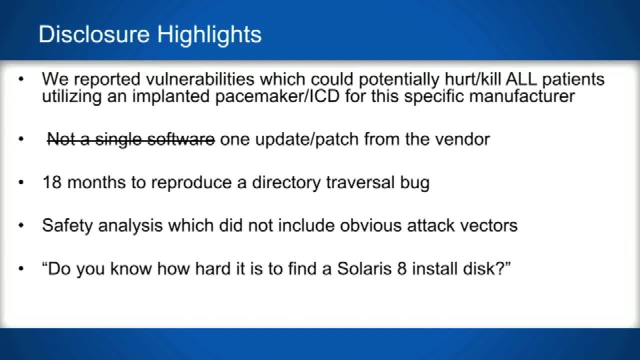 We're going to talk about that here in a second. And, you know, at some point in time we're encountering questions like: do you know how hard it is to find a Solaris 8 install disk? And we're like, oh man, it took 15 seconds on Google right to find an ISO. 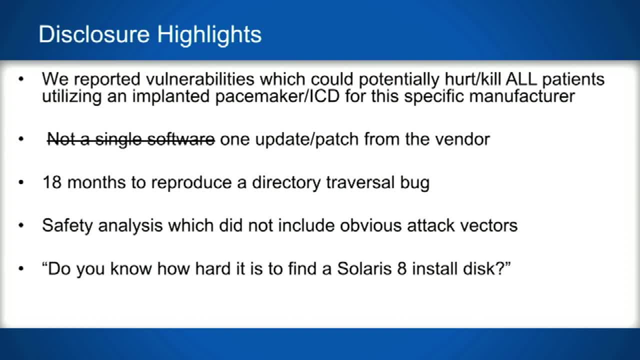 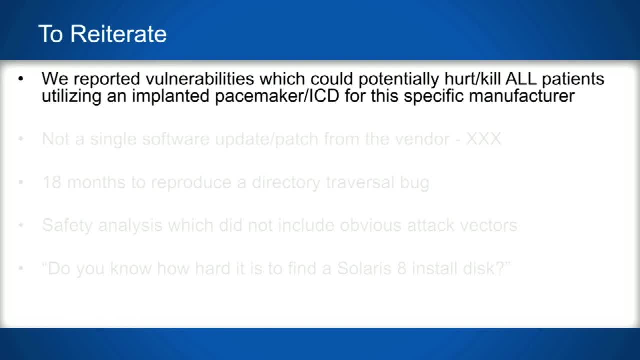 And then we're like, hey, you probably shouldn't be. We're running Solaris 8 on your update infrastructure anyway, right? So just kind of to reiterate: this is the takeaway for us, right? The rest of that stuff is interesting. 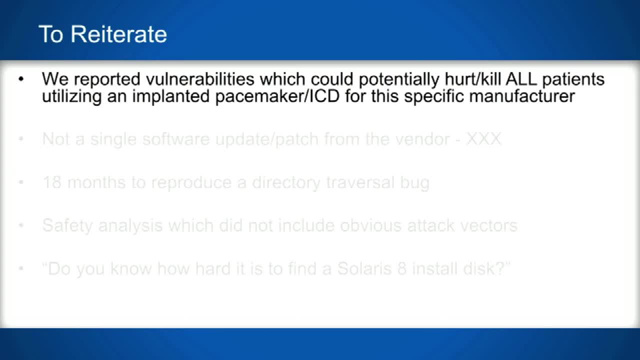 But from a vendor's perspective, we reported something that has the potential to hurt- kill- patients, So they've spent more time twisting the story or at least trying to put out a message from our perspective. instead of fixing this problem, We actually provided them how to fix it. 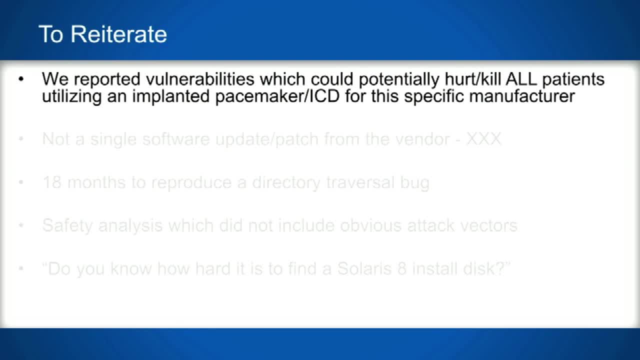 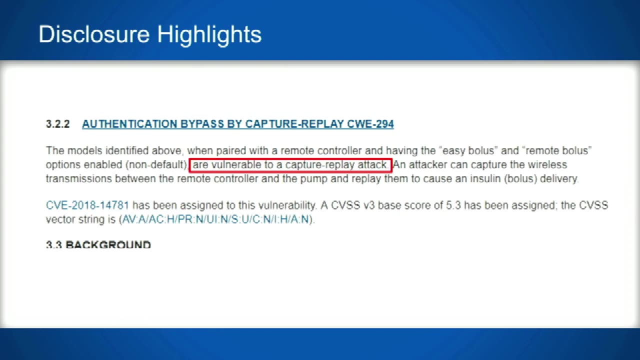 Their competitors have actually implemented security controls to protect, And probably for what? $20,000?. Yeah, engineer time, Engineer time, Probably all together. Instead, here we are today. So here's some of the trust issues we've gone through. 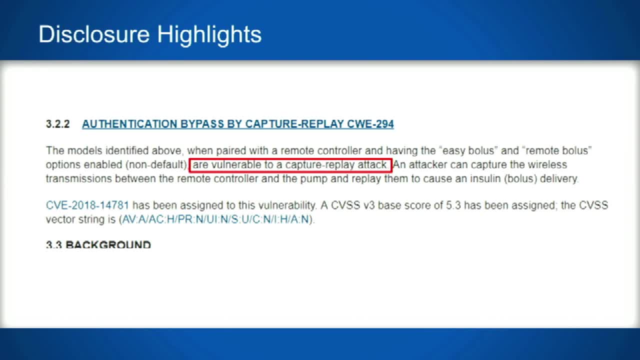 So this is one of the vulnerability highlights from the advisories from ICS cert. Yeah, this is a classic example of the lack of variant analysis, right? So we gave them a report that talked about some weaknesses in authentication mechanisms, And then the proof of concept that we had demonstrated a capture replay. 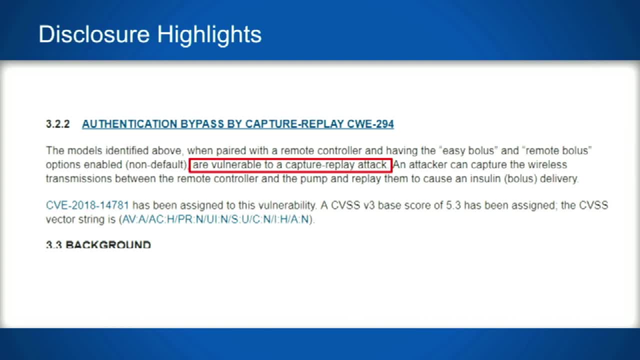 And so if you actually go to the advisory that's associated with this, if you look at the risk section it talks about, hey, the device is vulnerable to capture replay attack. That's actually not the full extent of it, right? We don't actually need to capture anything. 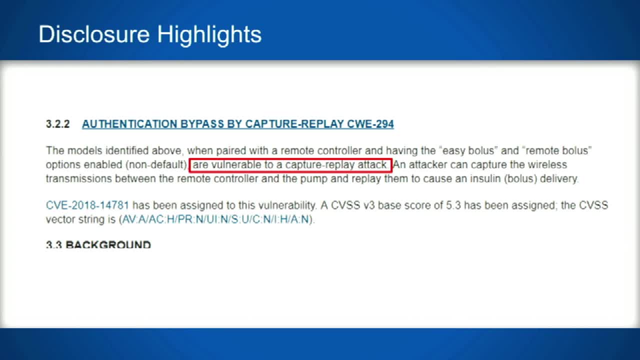 We know what the structure of the message looks like. We know how authentication occurs. Authentication occurs with a serial number. The serial number, the first couple digits of the serial numbers, are all the same from the programmers that we've seen, And so really you're just brute forcing like five numbers, right? 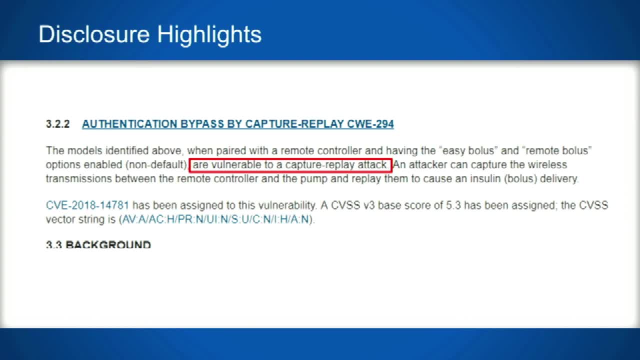 That's not a very good space, And so this is an example, though like hey, we shouldn't expect a researcher to literally develop a proof of concept for every feasible scenario. that's possible, right, We shouldn't have to do that. 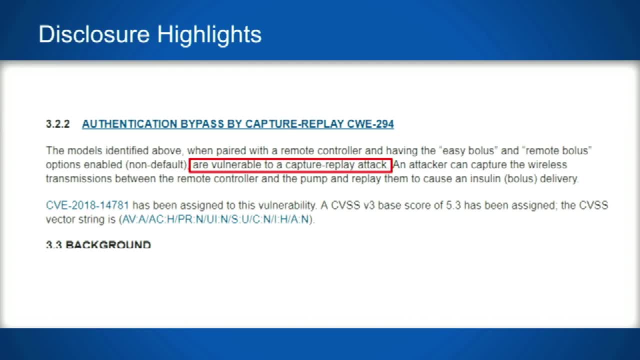 Instead, what we should do is say: hey look, these are the weaknesses that we discovered. Here's a proof of concept that we've developed that takes advantage of one of these vectors, And, as a manufacturer, you probably know your product better than anyone else. 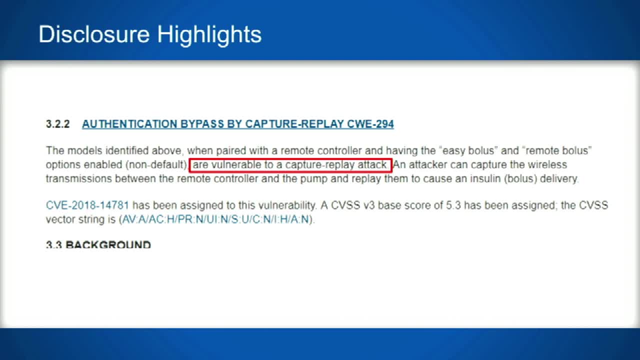 You should be able to understand what the variants are right And if you're going to publish an advisory, the advisory shouldn't be focused on the one specific scenario that the researcher reported to you. You probably have a responsibility to understand what the total impact of a vulnerability or weakness is. 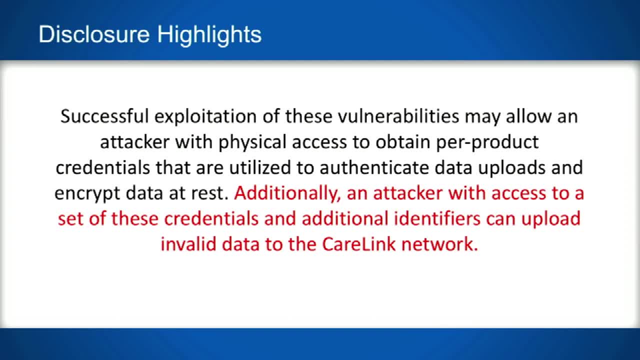 So this is an interesting one as well. Like we have this in red, highlighted in red. additionally, attacker with access to a set of these credentials and additional identifiers can upload invalid data to the CareLink network. Does anyone really understand what that means? 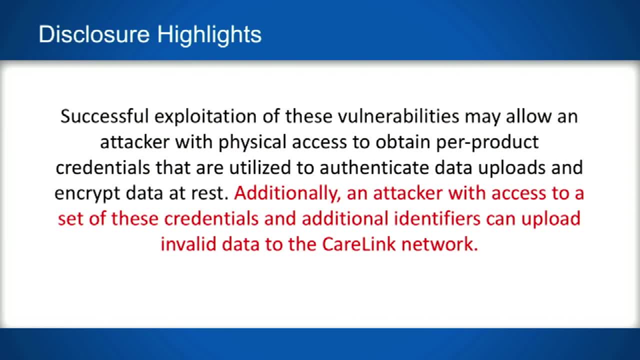 Probably not, because it's worded that way intentionally. How about I just break it down for you very simply? We had a vulnerability where we could literally upload data on behalf of another patient, right. So you're in bed, You have a patient monitor on your home, your bed stand. 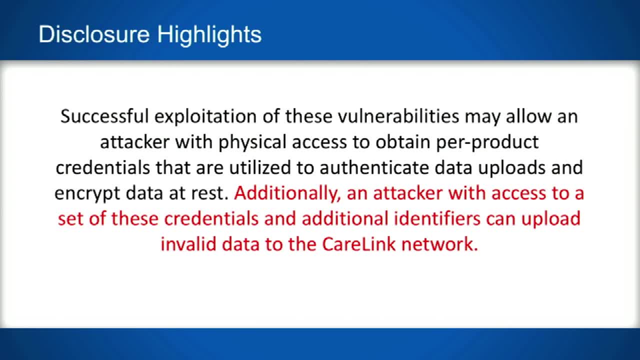 That thing's reporting information back to the doctor about what's going on inside of you, And we could just join a network and upload data, say, hey, you're not doing so well, Or maybe you're doing fine, right, And so this is another example of hey, if you're expecting folks to make a risk-based decision on the vulnerabilities that are affecting your product, you should probably give them the right data. 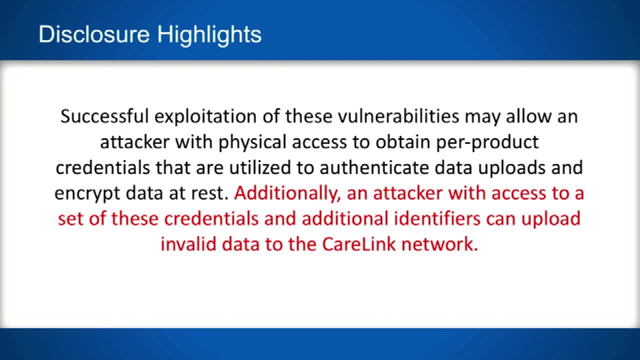 Right, I understand there's a brand piece to this. I understand that there's other things, other factors, political decisions and things that you have to understand, But at the end of the day, it's all really about your patients and the physicians that are taking care of them. 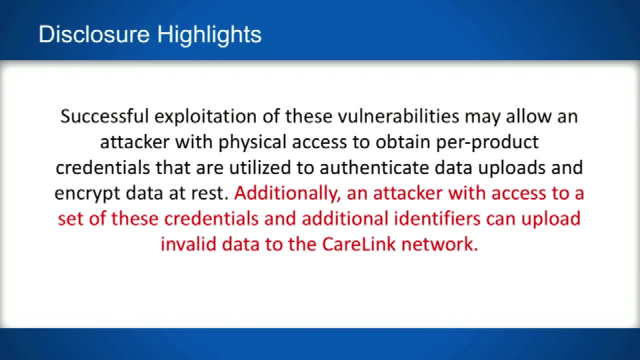 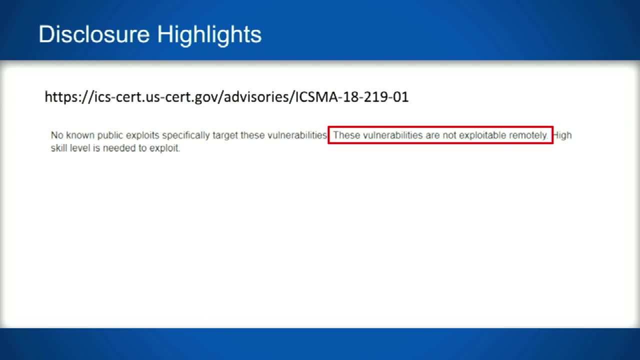 And we want the physicians to be able to understand what the real risks are so they can make an informed decision. right, Here's more examples. So I mean, we just read how a vulnerability is exploited on the last slide here. Every single advisory contains this statement. 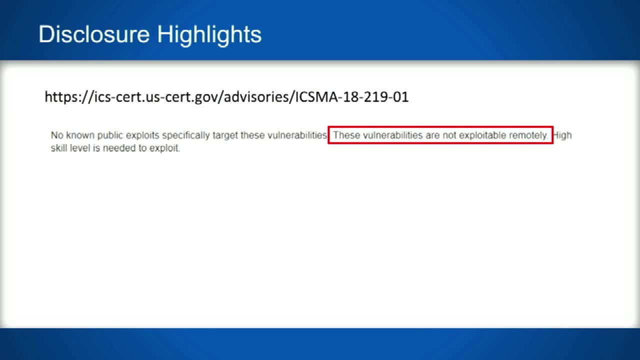 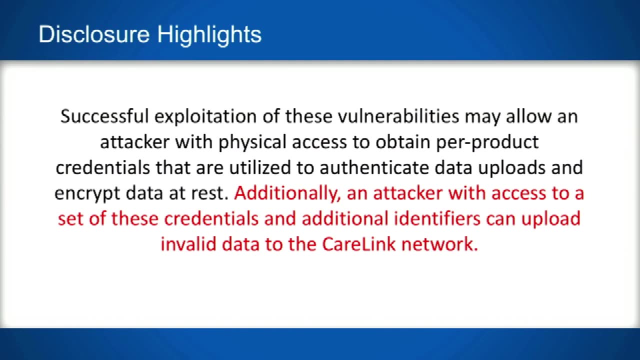 Sentence in there. These vulnerabilities are not exploitable remotely. So go back to the last slide. It's like: but somehow, even though it's not exploitable remotely, someone can upload data somewhere to a network. right, It doesn't make any sense. 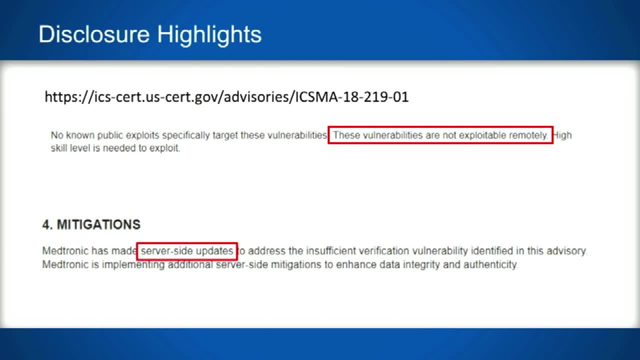 And so what we went through was a couple months of essentially just dissection of like, hey, yeah, we did server-side updates And we're like: how is this not remotely exploitable? One of the things we're going to show you is via radio. 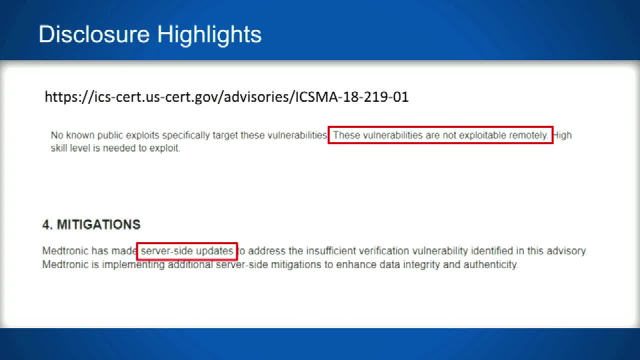 They're like: oh, that's not exploitable remotely, You've got to be close right, You've got to have some. It's like Like, look man, if it's a network-based exploit, it's a radio-based exploit. I think most reasonable people would call it remote right. 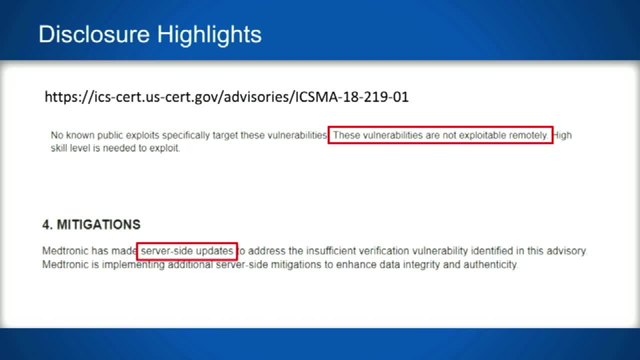 If I can do it from Starbucks, I would call it. If you can upload invalid data, like via Starbucks, to their network, it's probably remote right. But I don't know why this is in every single advisory right And then at some point you just get tired of fighting the PR spin right. 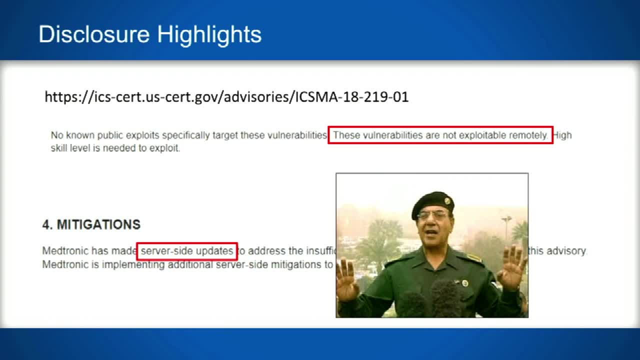 It's just like man. it's just not worth it anymore. Say whatever you want to say and we're going to come to a place, thankfully, like Black Hat. Yeah, Just show what we've discovered And then you can decide with your own eyes whether it's remote right or low risk. 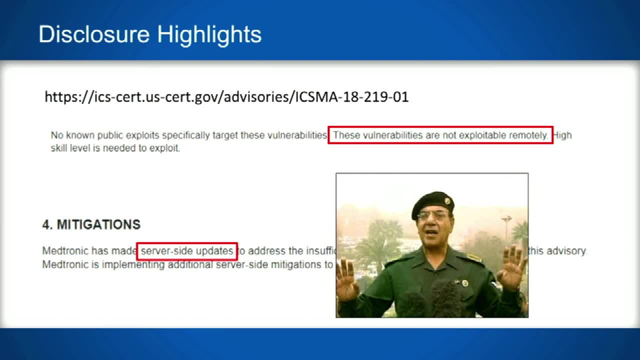 And I think the other piece of frustration for us is it buries the message. We're so wrapped around- remote not remote, It's like there's potential impact to patient safety out there And that message is lost because we're too busy focusing on characterizing these correctly. 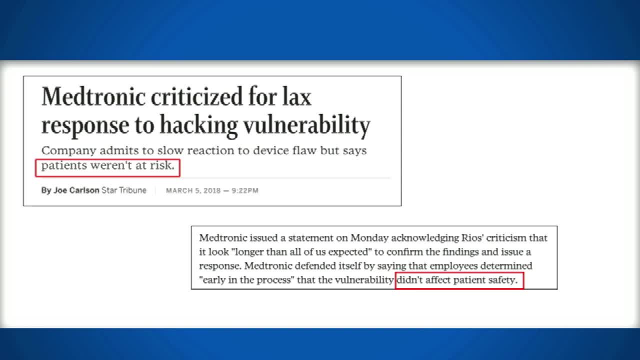 So here's another article that came out, And the company actually said that in the article that, hey, the patients weren't at risk, And even quoted that said: you know it did not affect patient safety. Well, fast forward up to right before this talk, yesterday, when news started leaking about what we were going to be presenting on. 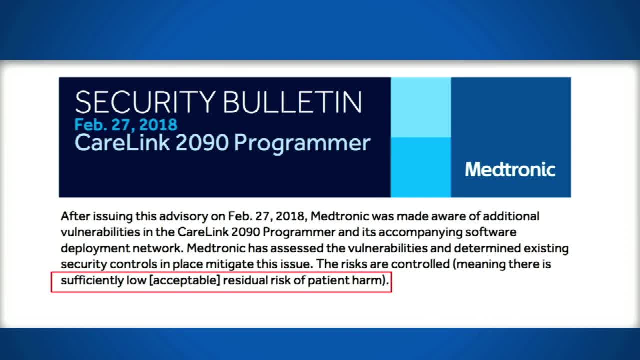 And now they said yesterday they released it yesterday, The security bulletin was dated 27th, But there's sufficiently low residual risk to patients' harm. Where does it matter, right? Is it none, or is it low? We're not talking about something that doesn't really matter. 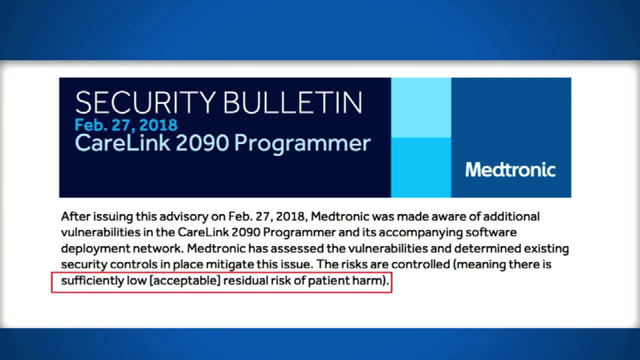 We're talking about risk to patient safety. Is it low or is it none? It matters to me If I'm a physician and have to make decisions off this. that should matter. And this is what we went through. It's like the verbiage changed almost every phone call we tried to have with them, every messaging. 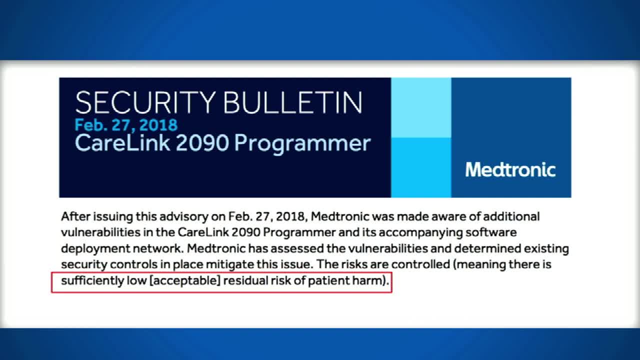 And it basically led us to believe is they don't really care about the impacts of what these devices have. That's what they showed to us Now. I find that hard to believe and I don't want to label everybody at a single company that way. 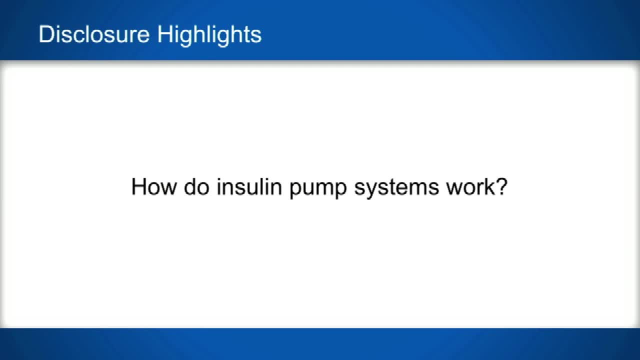 But that was just the message that was portrayed to us. So, yeah, we're going to get into now A couple of the different devices themselves. We have two devices that we're going to demo here. We, due to time constraints, we decided to stick to two. 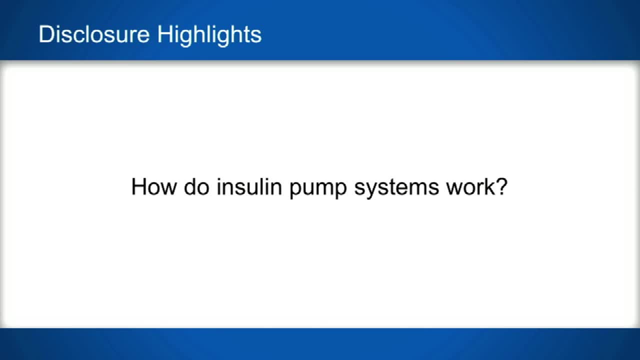 So go ahead. Yeah, hey, so I want to talk to you about how these insulin pump systems work. I think there's been some research on this in the past, But I just want to do a quick primer. So, essentially, what you have is what's called a meter, right? 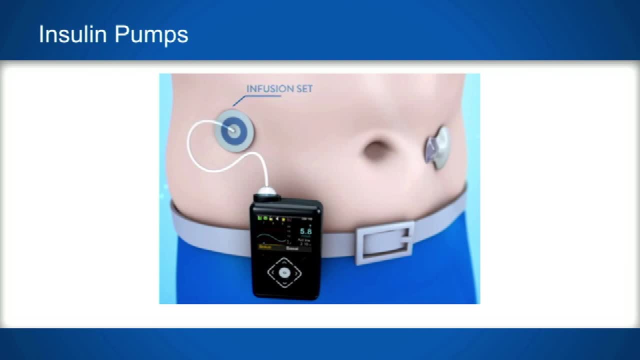 And that's this thing right here, And that meter, as you can see in the screenshot here, would actually be connected to something that could actually be implanted inside your body, right? So a little bit difficult to take apart, right? And then, at some point, what you would do is you would take a little bit of this: 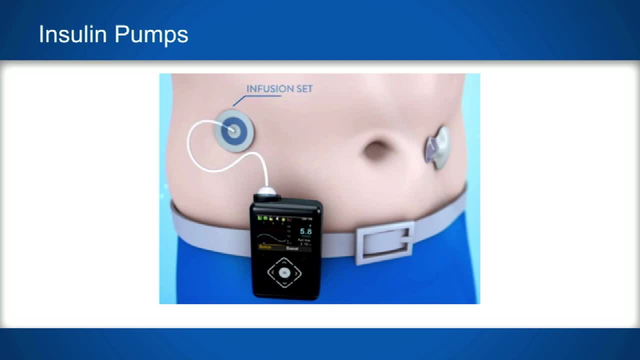 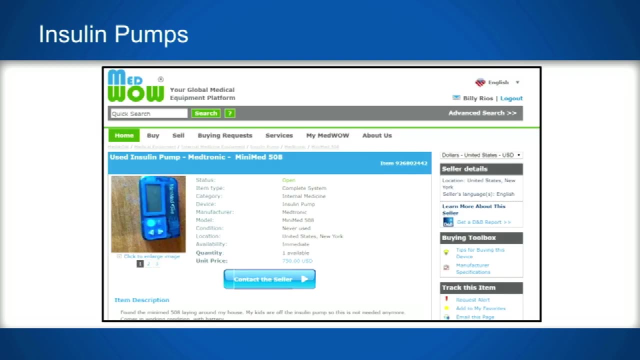 And what you would need is, this thing would actually control the amount of medicine that you're getting in a controlled way, right? That's what the meter is there for In some instances. what you might be able to do is actually control that yourself and deliver medicine when you need it. 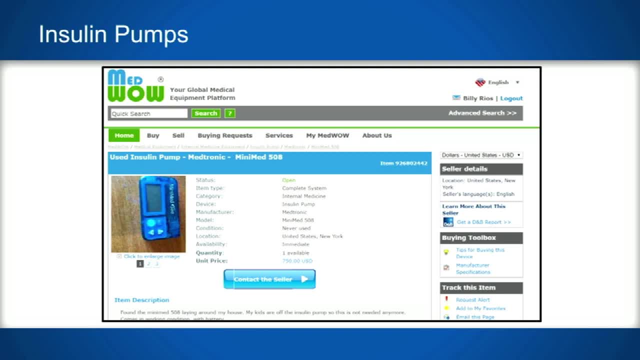 So how do we get one of these things? There's actually a lot of auction websites out there where you can actually buy these things right. In some cases you might need a prescription. It might be good to have a friend who can say: yeah, get it, give it to them. 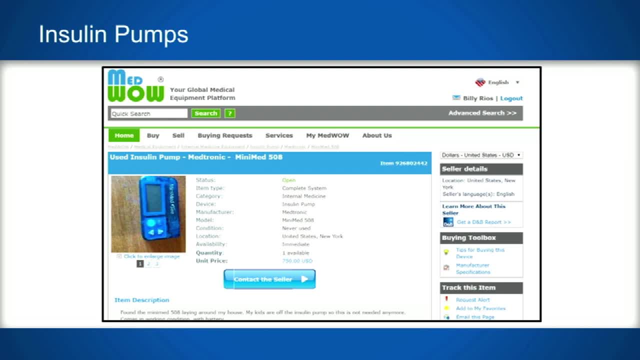 But in most cases when someone asks, hey, what are you using this for, What do you need this for, Or whatever, We just respond either over e-mail. It's like, hey, we just want to take a look at this. 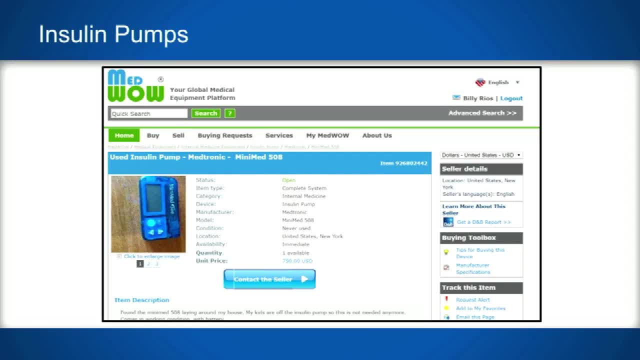 We think they're cool. They asked if I was a doctor. They didn't ask if I was a medical doctor, So it's like, yeah, I'm a doctor, Right? I think my favorite response was: like: whatever Billy wants, I approve. 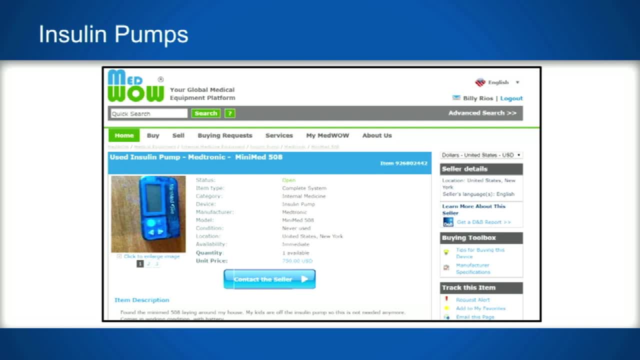 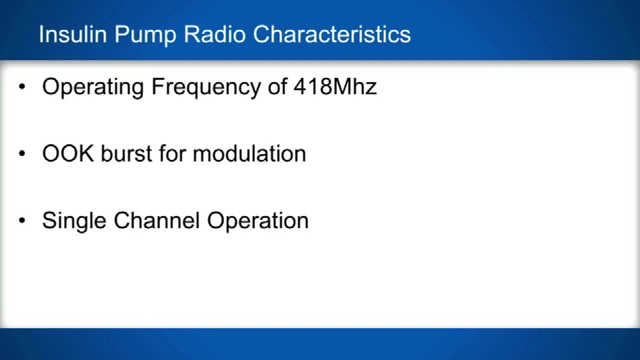 And the manufacturer was like it kind of doesn't work that way, But it is possible to get these things. obviously, This is the one that we have, And so some of the radio considerations. This thing broadcasts on 418 megahertz. 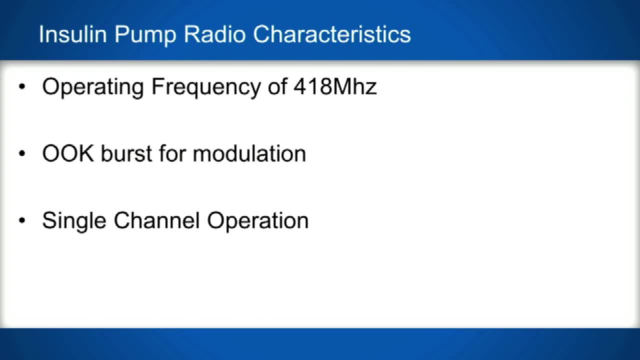 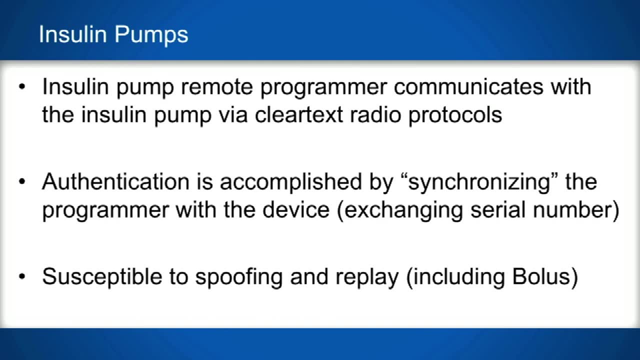 It uses on-off keying For essentially transmitting data from the little programmer to the actual meter Right, And then it's a single-channel operation. Essentially, what happens is there's an insulin pump remote programmer that you can actually turn on and say: hey look, if I push a button on this little programmer, it can actually deliver medicine or insulin, a bolus, what they call- into someone's body. 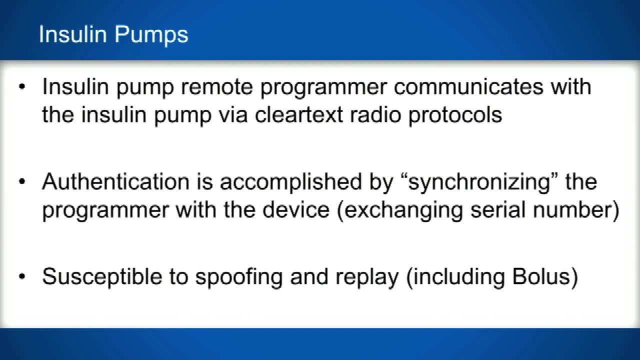 Right, That's pretty important. That's done via clear text protocol. Right, Authentication is accomplished by what we call synchronizing. There's a button that's like called synchronize Right And then you have to synchronize Right And then you have to actually program the serial number into the device itself. 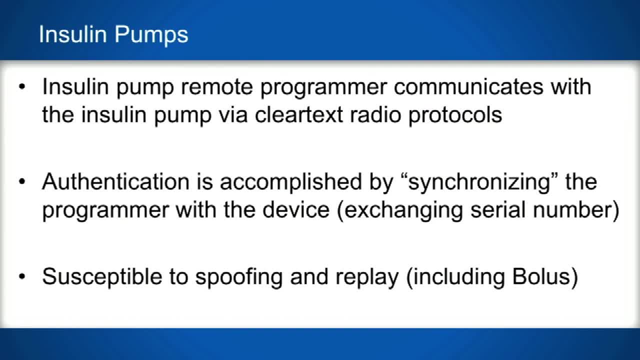 And so the device, when the radio piece is turned on, it just loosens for signals, And if it has the right serial number at the header of the message, it just takes that message and processes it Almost like a serial bus. 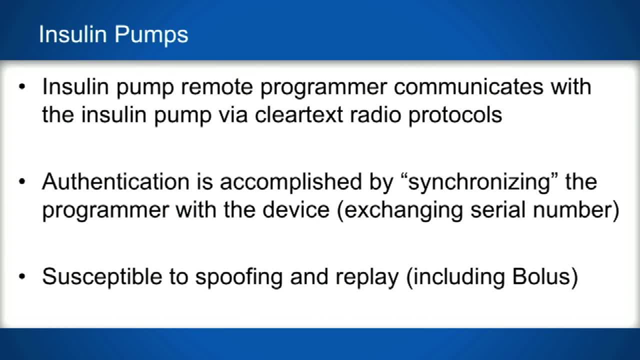 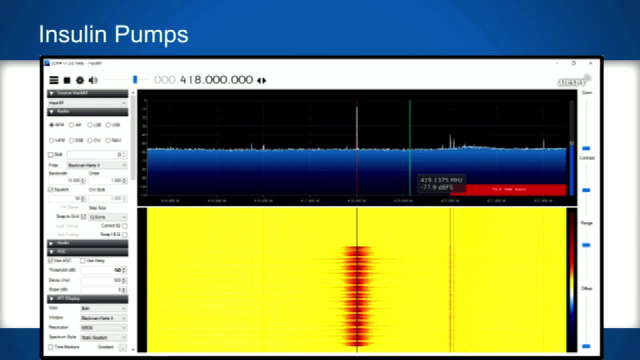 Right And then. so this is obviously susceptible to spoofing and replay. Right, That includes bolus, And so if you capture the signals in the air, this is what it looks like, Right? So this is what a captured synchronization message would look like. 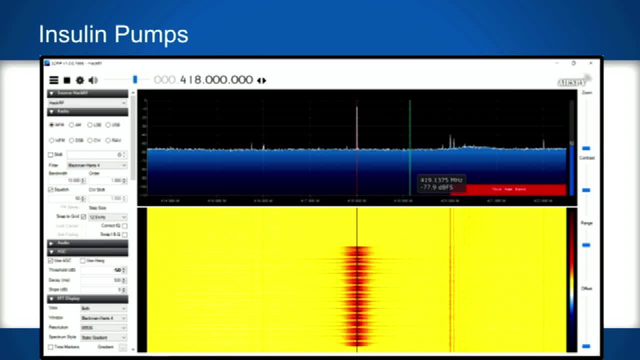 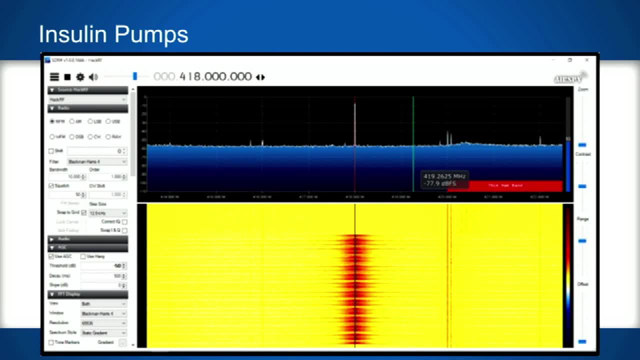 Right, And this is what you would have to essentially Do: to initiate the pump in order to take some kind of message, to do some action, And then, if you take another message for the actual bolus, this is what it would look like as well. 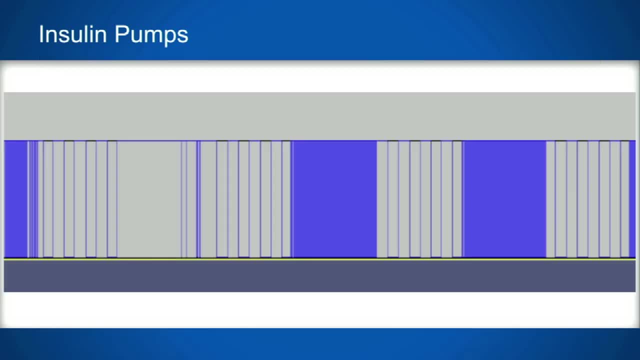 And then if you actually break that down into the bits and bytes, like demodulate it, you'll see that it's a very simple message that gets passed And the way the authentication is done is via serial number at the very front. 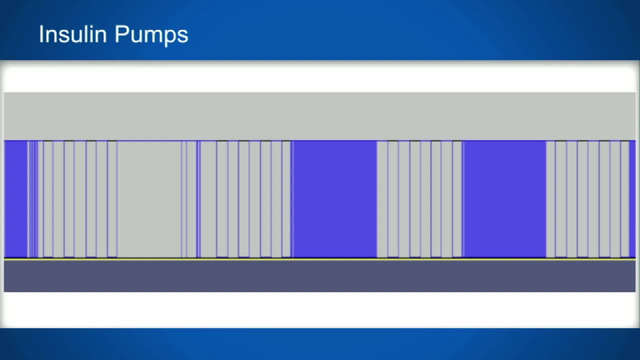 So if someone is able to guess your serial number, if someone listens in the air and captures your serial number, or if someone just brute forces the five digits that change for the different programmers, they will be able to guess what the serial number is and they will be able to initiate synchronization and bolus or the stopping of delivery of medicine on a pump if you have the radio mechanisms turned on. 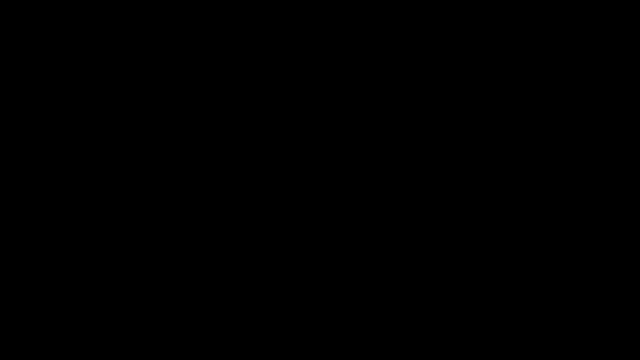 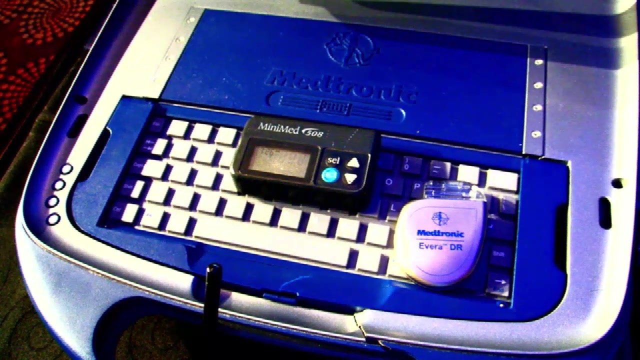 So we're going to demo this for you here. Can you turn this guy on here? I'll show you what this thing looks like. So we have this meter right here, We have a program around here somewhere, but, more importantly, I have a hack RF like sitting right next to it. 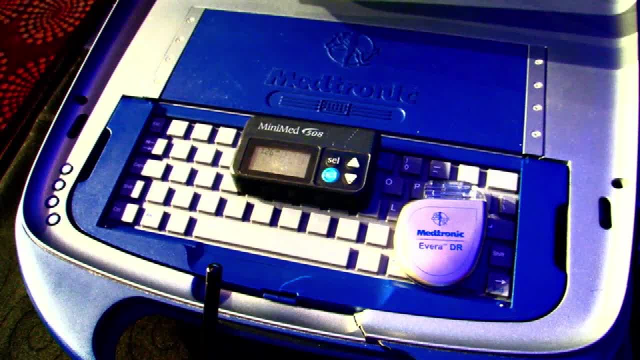 So we're going to be broadcasting over low power And, to be honest, the message that we're going to broadcast Has this device's serial number or the programmer that's programmed to hear the serial number, so it shouldn't affect anyone else. 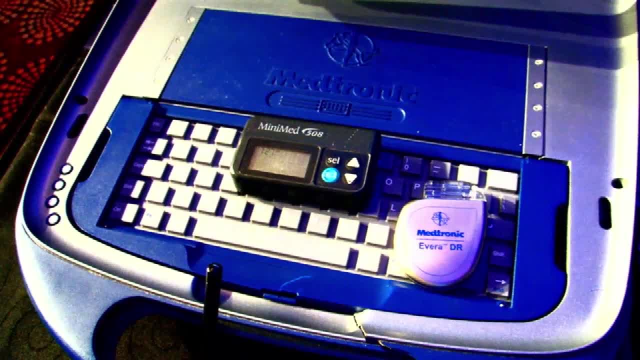 But, man, if you have a radio device, that's especially one of these, I would back away. I'd probably leave, man, because these things do some weird stuff, right, And some stuff that we can't explain. So again back to the point, as Billy sets, this up is remote, not remote. 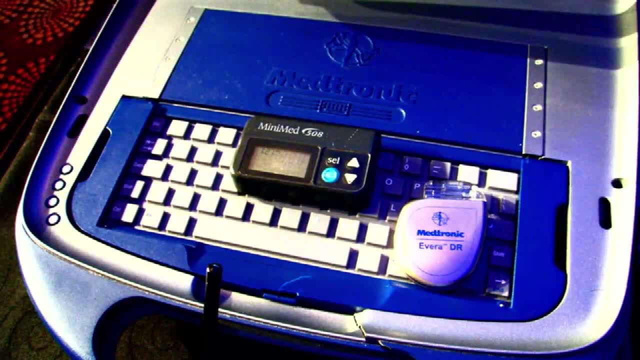 This is his laptop connected to an RF device. We're not connected through any physical cabling at all to that device. Again, definition by me is remote from that standpoint. Yeah, And then Let's see. You might be able to see this. 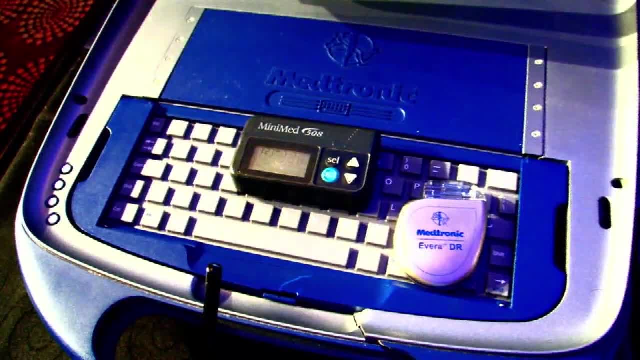 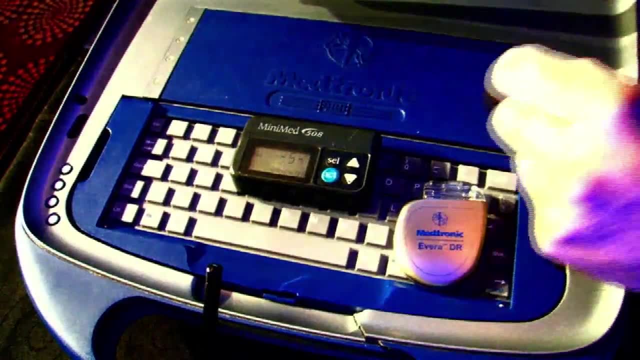 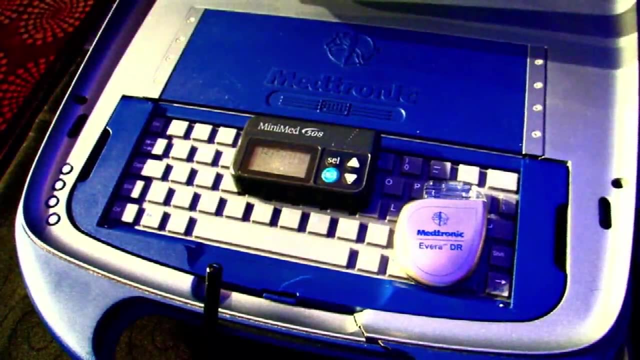 Yeah, just give it a second. We'll start going about now here. I mean I wouldn't classify this as remote. I mean look how close it is, right. I mean come on right. But I think the important thing here is that we actually changed this demo last night. 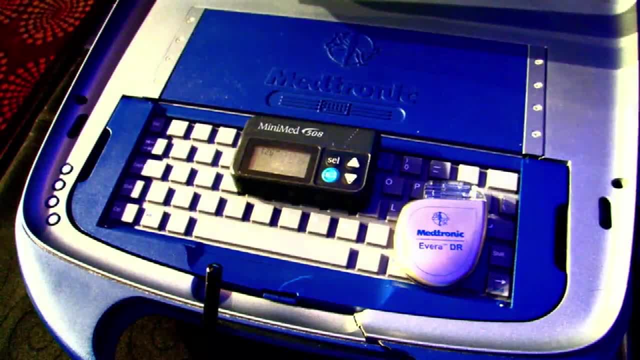 We stayed up pretty late last night to change this demo. The original demo that we had delivered bolus, right like dumped insulin in someone. This one actually stops the delivery of insulin. Does anyone know why we did that? Because if you read the advisory the risk is like hey, this attack could be used to deliver bolus. 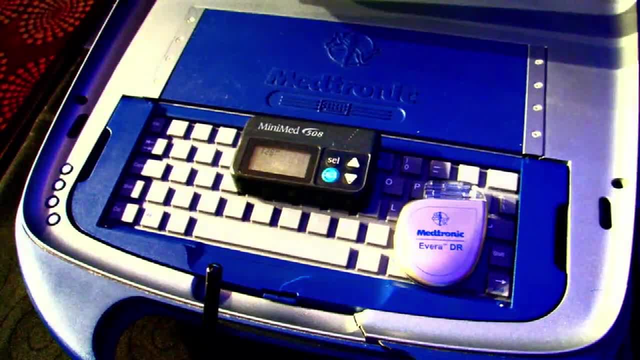 It just talks about the one scenario that we showed in the proof of concept We're like it goes well beyond that right. Whatever the remote programmer can do, we can do that. So if the remote programmer can stop the delivery of medicine, we can do that too. 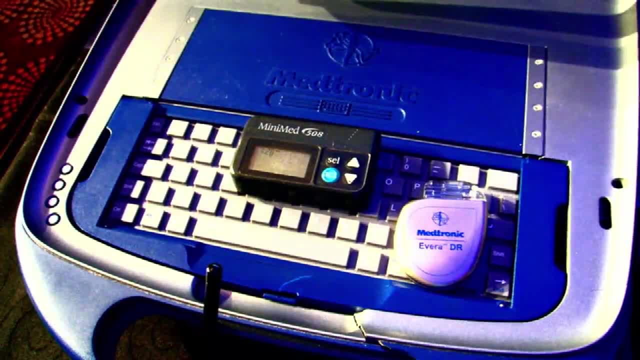 If the remote programmer. If the remote programmer can update settings on the device, we can do that too. If the remote programmer can deliver bolus insulin to someone when it's not supposed to, we can do that too, right. 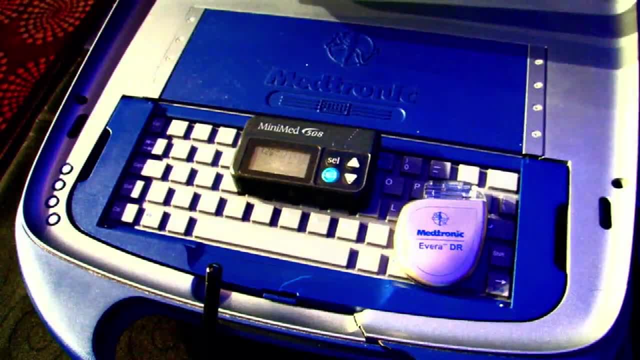 And so if you go read the advisory, it just talks about one scenario. right, Go read the advisory, See, that's why we changed this right, Because when we see things like that, it's frustrating, right? It's like: do we really have to do proof of concepts for every single scenario? that's possible. 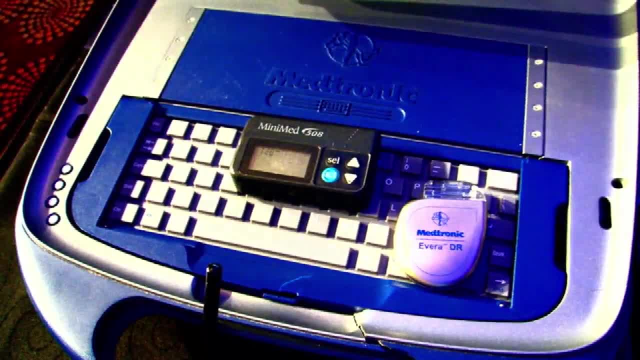 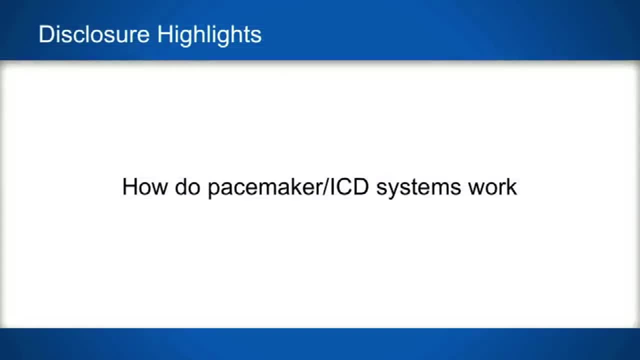 I don't think that's reasonable right. Want to go to the next one? So the next. We can switch back Back to the slides. Yeah, Or do you want to? No? All right, So that's the one piece of it. 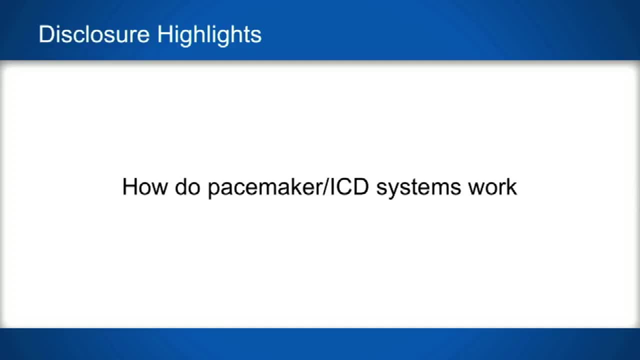 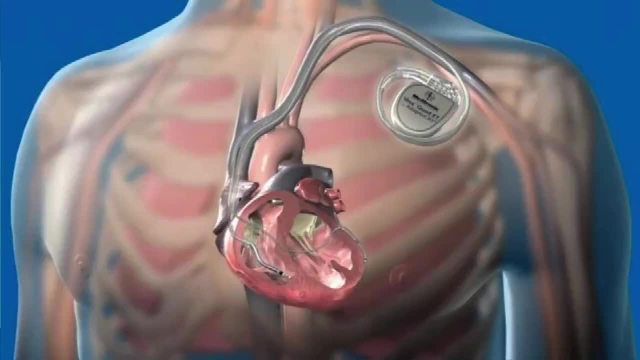 The second device that we talked about, which actually probably gets more attention, just because it seems a little bit more nefarious, I guess, or impactful, is the pacemaker and ICD systems And so kind of just how these things work. They're actually implanted underneath your skin. 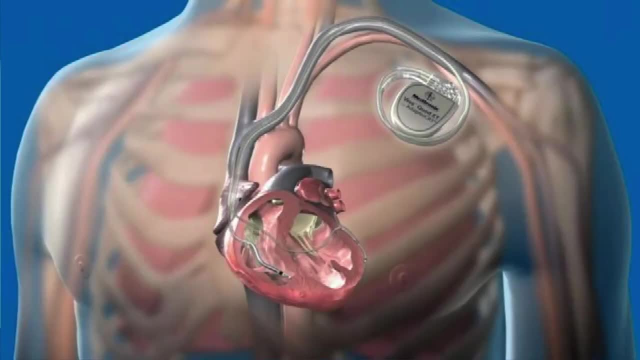 There's some leads that are put into- Yeah, and there's one right there And there's some leads that are put in- And it'll actually control the pacing of the heart. The ICDs will actually, if certain circumstances are met or parameters are met, will actually initiate a shock to regenerate the heart beating. 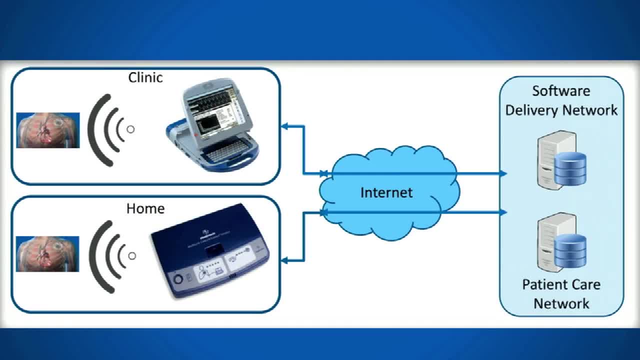 But the important part of this is this whole thing is an ecosystem. It's a system of systems, ecosystem And so the way these are set up within the patient's home on the bottom left, there you actually have a patient monitoring system And most of these they sit at the nightstand. 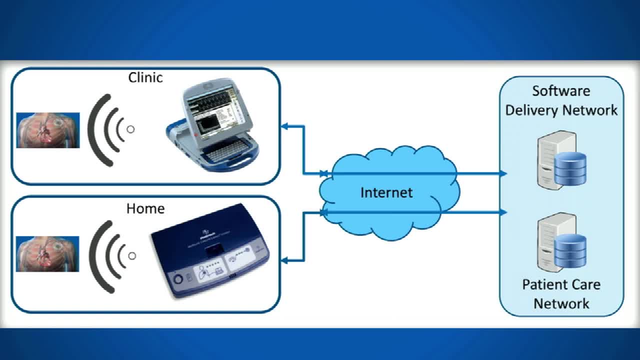 The device communicates. It communicates to that, usually at night when the patient's sleeping, because it's gathering data and sending it up through the network over to a patient care network. That way the manufacturer can monitor it But, more importantly, the physician can get indicators for that patient. 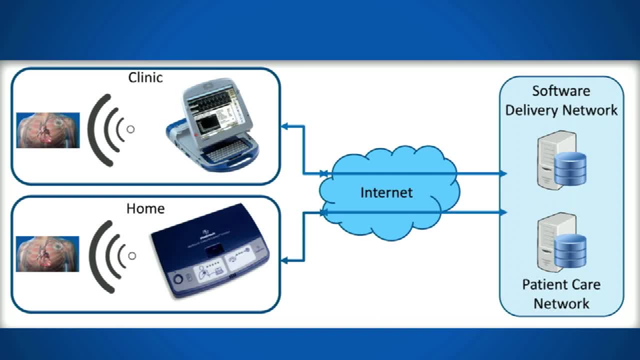 Another part of the ecosystem is the actual programmer itself, And that's sitting at the clinic And that's what the physicians will use to actually program the therapy that goes into the pacemakers, And so it's done over an RF communication. They will program when it's supposed to shock, what the pacing 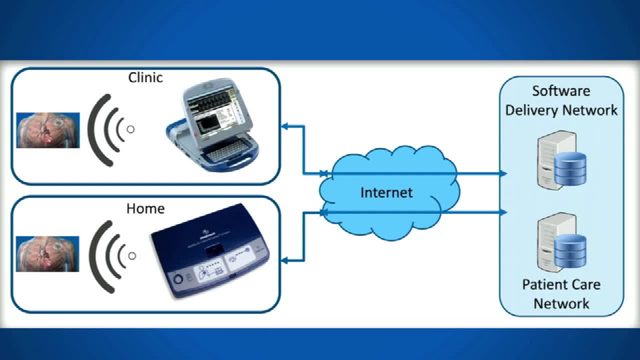 What the algorithm is and a whole set of parameters for that patient. then the back end piece of it, which is also part of this ecosystem, is the SDN, or the software delivery network. So this is where updates are actually pushed down to these devices, or from the perspective of the patient care network, which is also back in the manufacturer where that data is brought in. 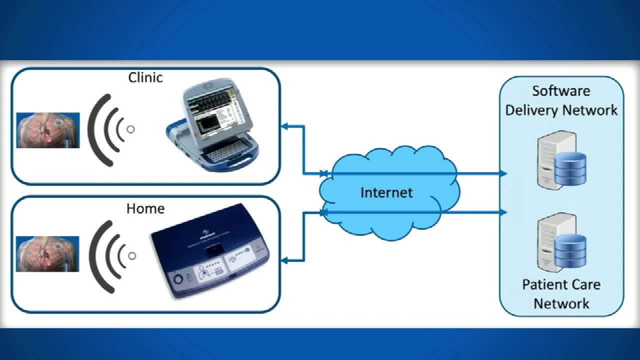 Yeah, Another important thing to understand is that these programmers are what you're looking at right here. So what you see in the top left hand corner on the slides, that's this right, This is a physician, This is a physician programmer. 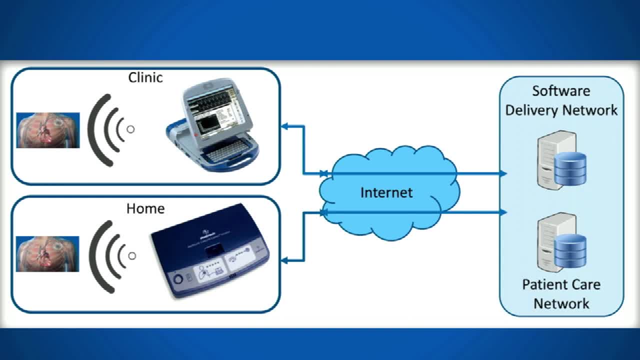 These things also have the by design capability to update the firmware on the device itself. So not only is there a program on the pacemaker or ICD that says this is what the pacing cadence should be, This is the criteria to deliver a shock, to get someone's heart started. 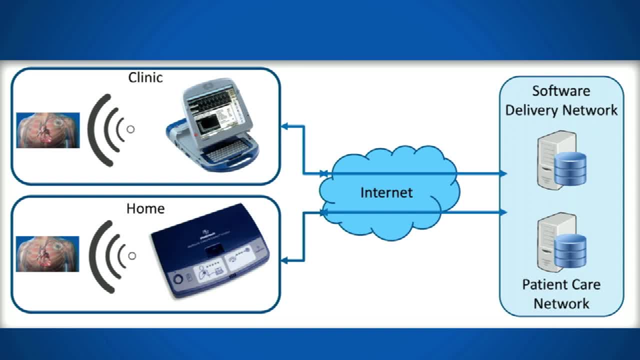 This thing also has software on it as well, Right? And not only can this programmer adjust the therapy that you're getting, it can also change the software on the device by design. That's by design, Right. So when we look at these, 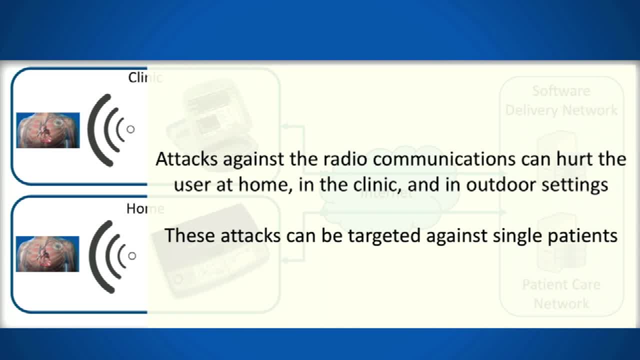 The actual programmer themselves, the various devices. So if you look at the radio communications- and this is what some of the past research has alluded to- you can target a single patient And that's almost like the demo we just gave here is, you can target a single patient using RF. 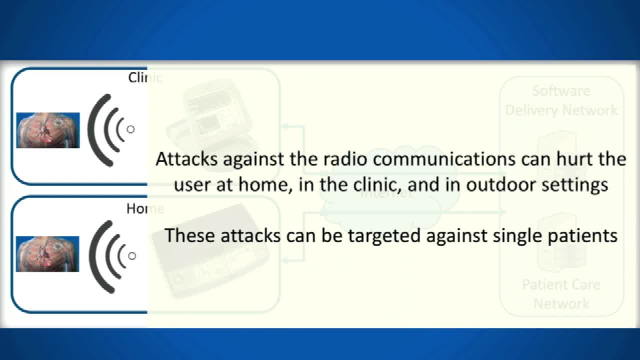 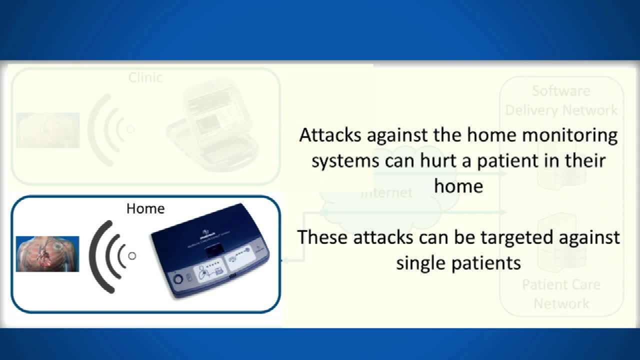 And so that's kind of the one to one scenario as we would cause it is, I can launch an attack against one specific individual. So if we look at the home monitoring station, if I go to someone's house or I target that specific home monitoring system, I can do a one to one attack. 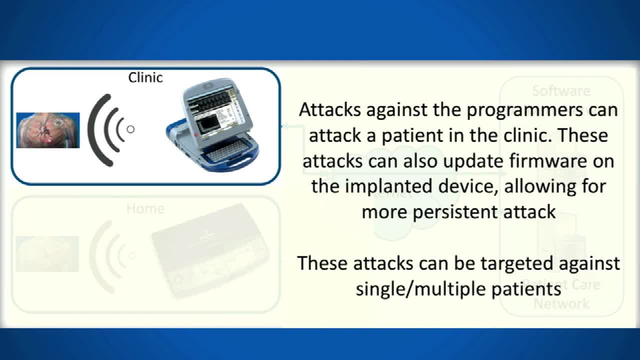 The programming is a little different. It's kind of one to multiple, just because that programmer sits in a physician's office or operating room or clinical setting, And those devices will program multiple ICDs. So those programmers might be responsible for a dozen, a hundred more. 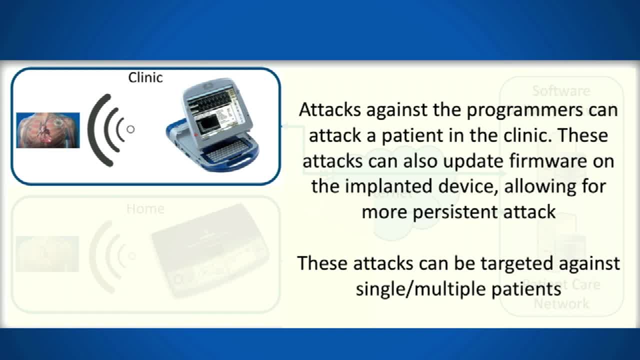 And there's about what? 10,000 of these, I believe There's tens of thousands across the world- This specific programmer That are actually used to program the devices And this is for this vendor. this is the model they have right now. 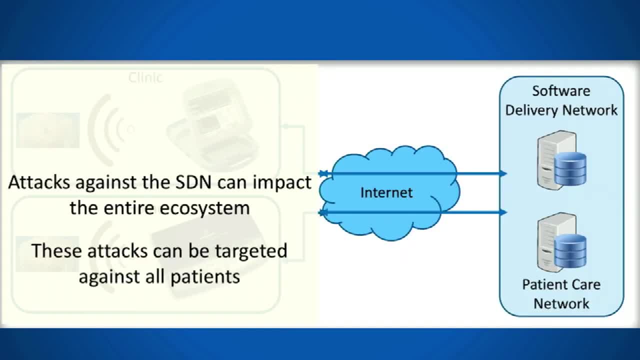 There's not a new one. This is a newer model. The software is up to date, Current patch to patch level. Yeah, these are the most interesting attacks, though. So there's a mechanism, a communications path from these devices through the Internet to servers that are basically Internet facing. 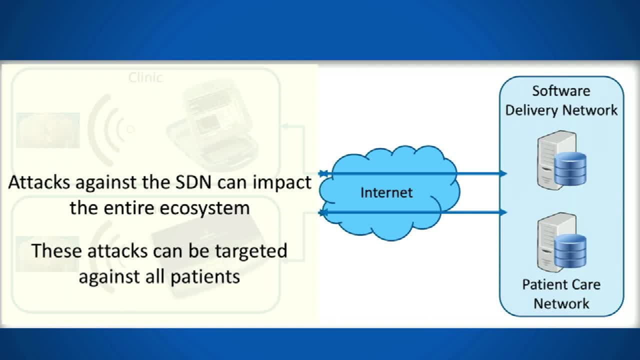 We'll show you how that works exactly. And there's a software delivery network and a patient care network. If someone were to exploit these components in its current situation, this is where you can attack every patient right, Because you would have access to update software on a home monitor. 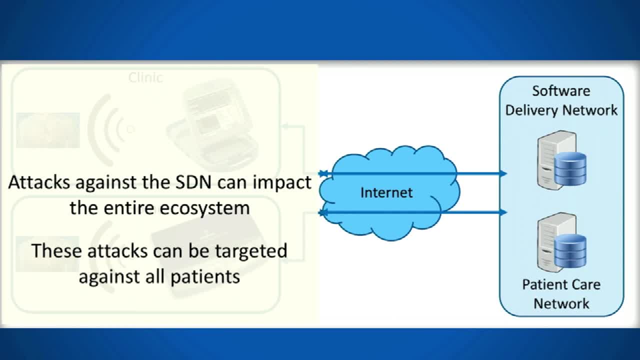 You would have access to update software on a home monitor. You would have access to update software on the programmer And if you have access to a programmer, you can influence the software on the programmer. What can you do? You can buy design change therapy and you can buy design change software on the actual pacemaker, ICD right. 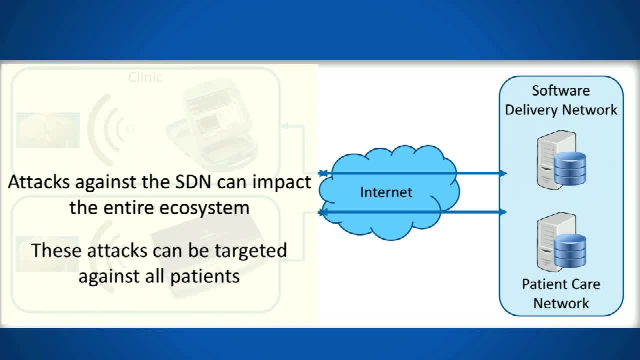 So when you look at the threat model, you know the radio-based exploits are really cool, We love doing them. The attacks against the actual programmer itself and the attacks against the actual home monitors- really cool, We love doing that too. 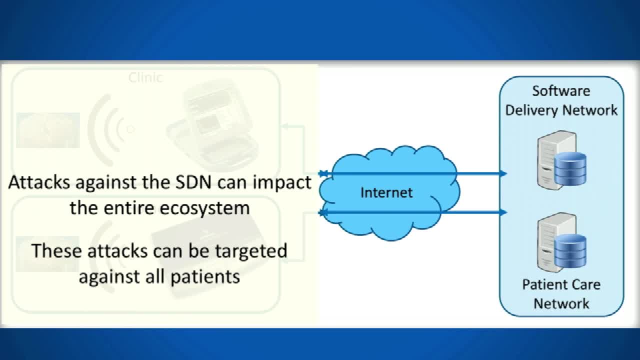 We have lots of phones and those things, But the communications path between these devices and this infrastructure over here, This infrastructure over here, is the most important piece, Because if any part of this gets compromised, the potential for every single one of your patients to get hurt or killed is present, right, 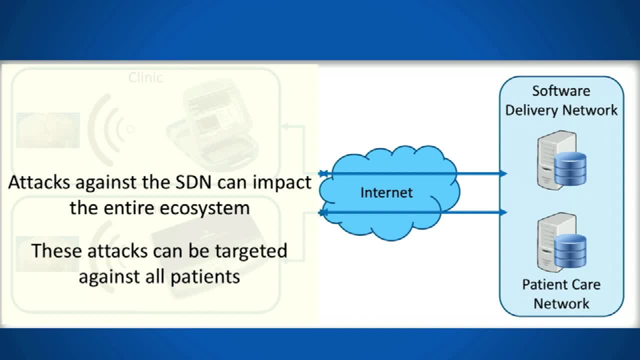 I'm not saying every vulnerability allows that, But if someone compromises your software delivery network and you don't have the right mechanisms in play, they will be able to leverage that to influence every single programmer in the field right. And if they can influence every programmer in the field, they can reprogram the therapy and the software on every single device in the field right. 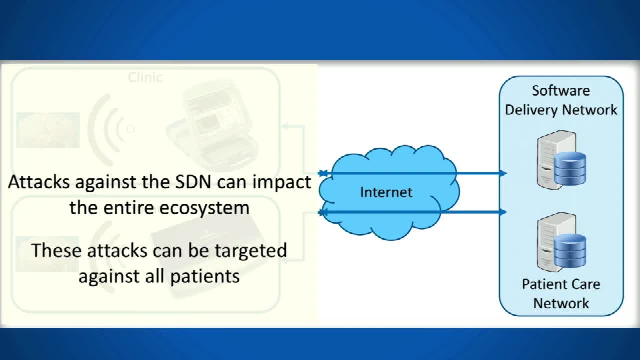 So these parts are the most risky parts of the threat model, Right? So if you're a vendor and you develop these things and someone starts reporting vulnerabilities in your software delivery network, you should probably take it pretty seriously, right? And so what we're going to do is just kind of give you an example of how this works, right? 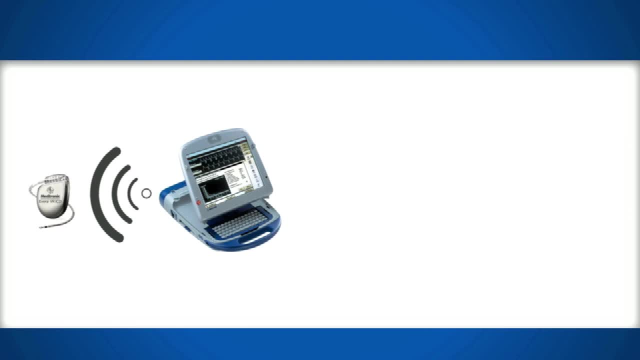 So we have a programmer like this. The programmer uses RF to actually interact with the ICD or the CRT, because this is inside someone's body, right? You can't hook up a USB port to it or anything like that, So that's done by radio. 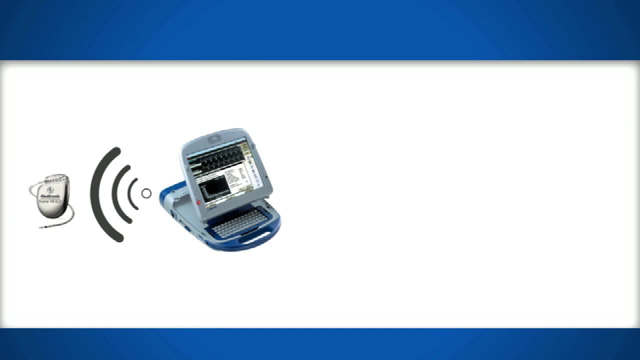 So you have to be in pretty close proximity to get access to that communication stream. Next slide, And then there's this Internet component and there's a software delivery network. So actually, how does this work in the real world? So go one more. 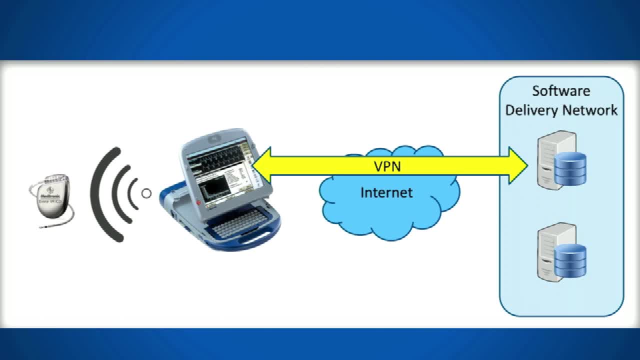 What this programmer will actually do is, when it's ready to download software updates, it will actually establish a VPN to the software delivery network And then, once that's done, it will actually pull software updates down right. So at a high level, that's essentially how the updates occur. 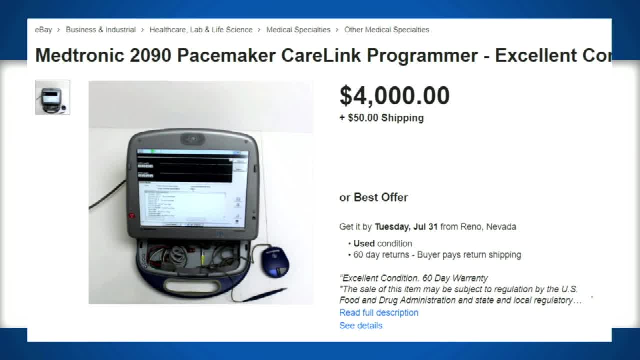 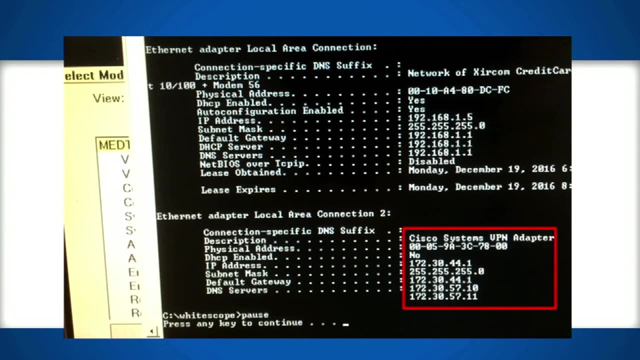 So the next slide. And so if you really want to take a look at one of these, you can go to various auction websites and just buy one, Right, This one's in excellent condition. And then if you manage to, let's say, get a shell on a device and kind of monitor what happens after the VPN is established, this is what you'll see. 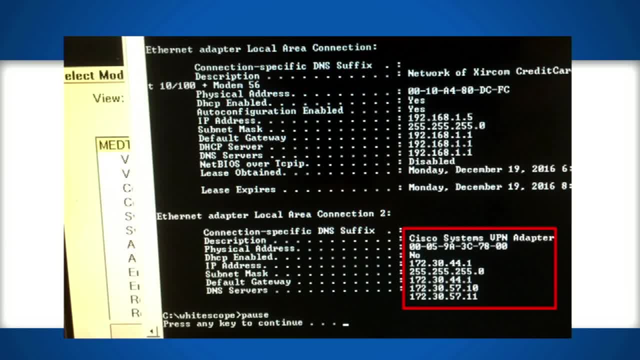 You'll see two network adapters. One network adapter will be on your local network or wherever it's connected to, And the second network adapter, which is a traditional commercial off-the-shelf VPN client, establishes a connection to an internal software delivery network belonging to the manufacturer, with its own IPs and own gateways, and so on. 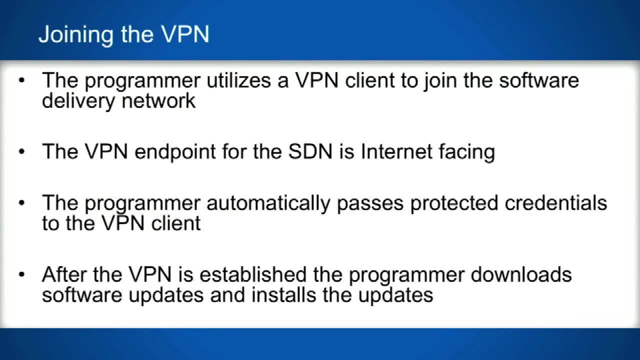 All right, So the next slide. And so, like I said before, a programmer utilizes a VPN client to join the software delivery network. The endpoint for the software delivery network is actually on the Internet, That is, an Internet-facing server, Right. 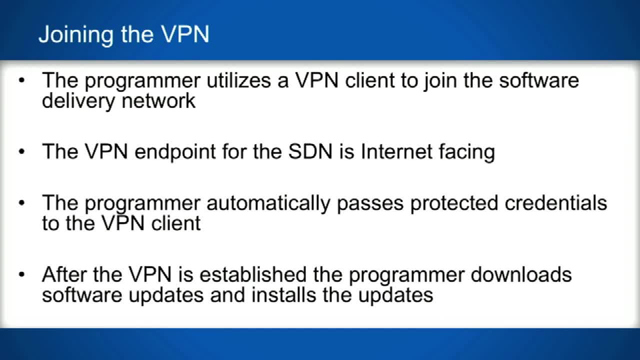 So when this thing downloads software updates, it is connecting to an Internet-facing server to establish a VPN and then downloading the update. once it's on the other internal software delivery network, The programmer automatically passes credentials from the programmer to the VPN client in order to join the VPN. 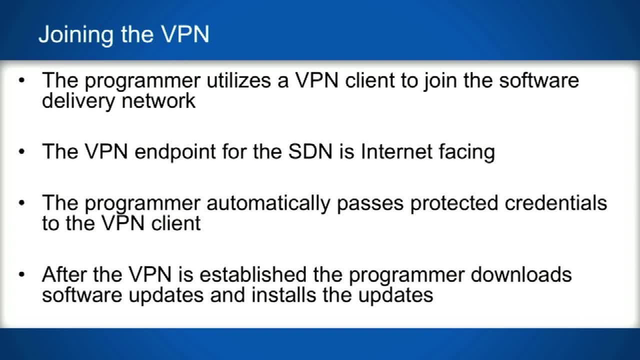 So the doctor doesn't type in a password, nothing like that. It automatically does that Right, And then, after the VPN is established, the programmer will download the software update, And then what does it do? It executes it Right, And so there's some interesting observations here. 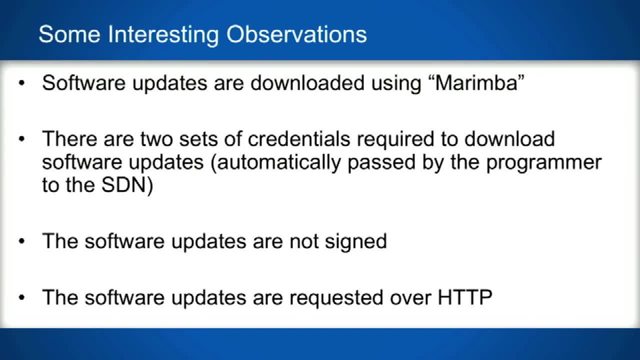 And this is what we actually reported to the manufacturer 550 days ago- More than 550.. Yeah, We said hey, we know how your software update mechanism works. Right, There's this VPN thing. It's kind of interesting. There's this really- I don't want to say ghetto- really interesting software called Marimba. 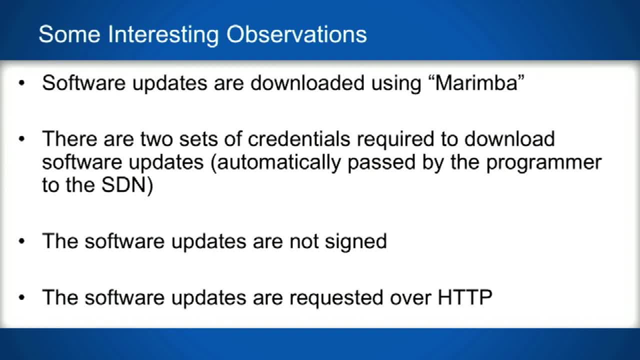 Right. So it's actually end of life. It's not supported anymore. There's two sets of credentials that are used to essentially initiate this download process: One set of credentials to join the VPN. One set of credentials to authenticate to the update server. 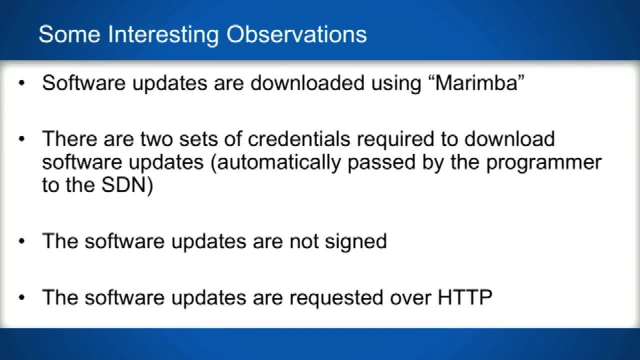 We've got both of those. The software updates are not signed, So if anything ever happens to the update server and they serve back an update, the programmer is going to run it Right And the software updates are actually requested over HTTP. So I mean, is it HTTP that's secure or HTTPS? 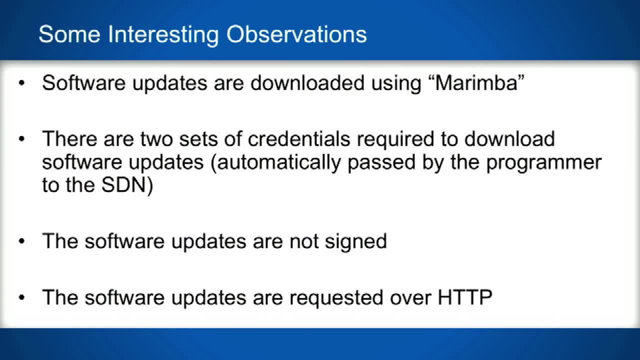 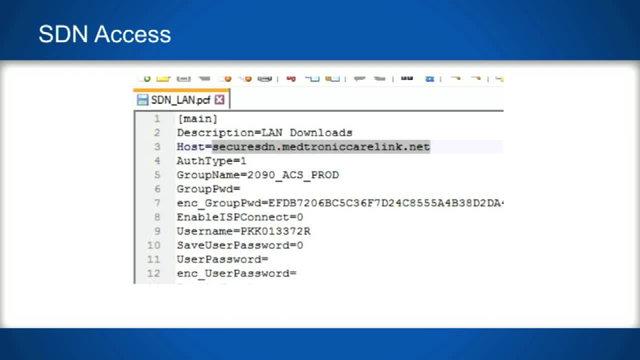 I can't remember, I don't know. One of those S has an extra letter. I always forget. Right, Yeah, So And so this is what we're looking at. Right, This would be the endpoint for the VPN on the Internet. 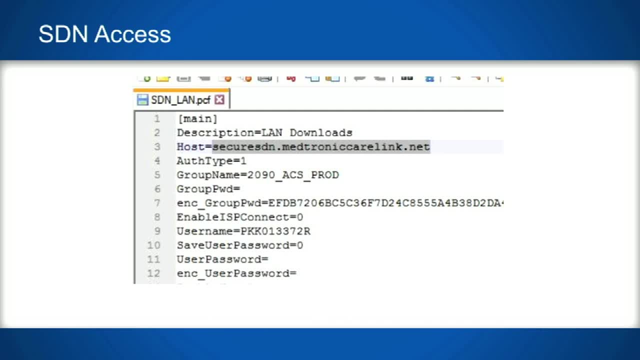 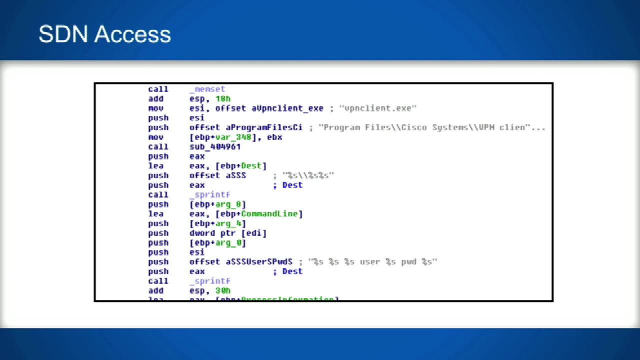 Right, Pretty interesting, And since we can see the actual configuration for the VPN client, we can figure out how to connect to it. One problem: The password is not in the VPN client configuration. The password for this is actually stored in non-volatile memory on the programmer. 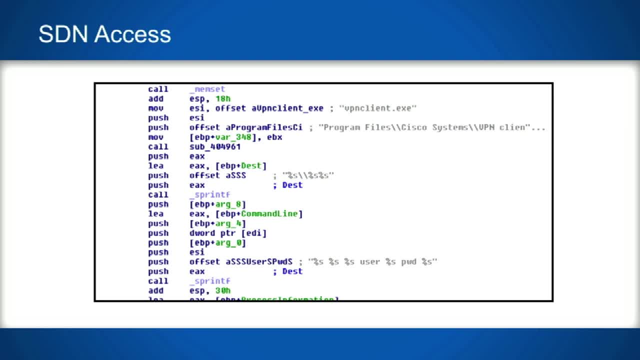 Ah, kind of a neat trick. No one would ever look there. Right, Clear text, Yeah. So we start to reverse engineer some of the way that this works And we realize, if you take a look at this IDA disassembly, at some point in time the username and password get passed to the VPN client via the command line. 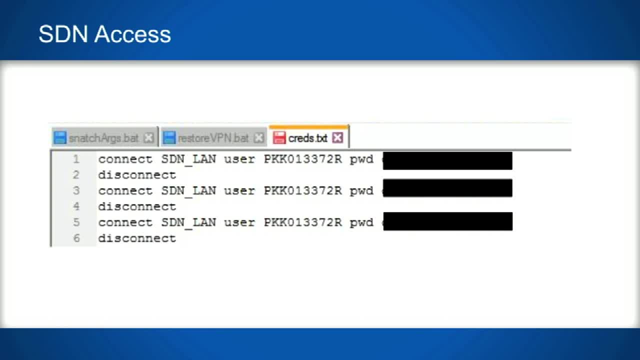 Pretty interesting, Right? So what we ended up doing is writing our own VPN client saying: hey, you know what, instead of just logging into the VPN, why don't you just log this password to a text file? which is what we did. 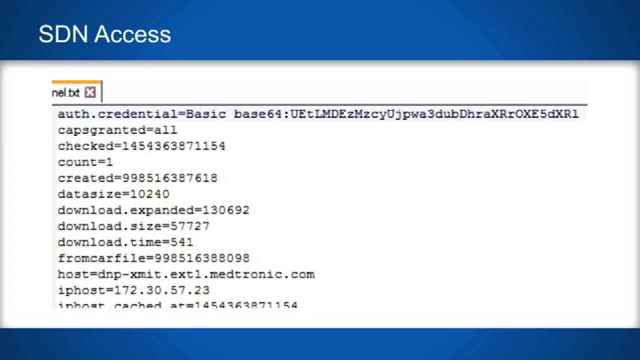 And so now we can authenticate to the software delivery network. Once we're inside the software delivery network, we need another set of credentials. We need another set of credentials to actually authenticate to the update server Right, Base 64.. There's the credentials, right there. 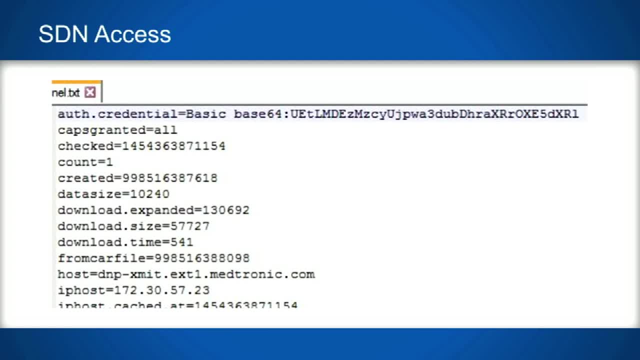 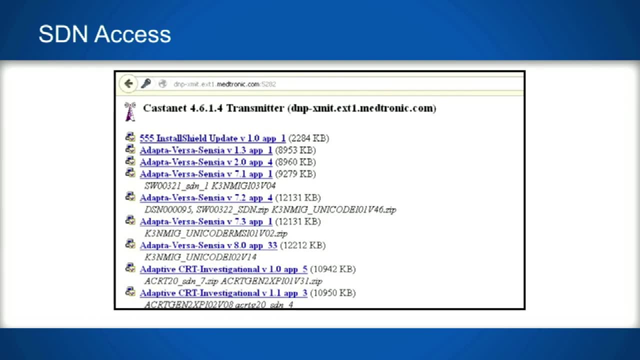 Right So, base 64. No one would ever guess that. Right, It's uncrackable, Right So? and then also, what's in there is the actual host name for the update server on the internal network, Right So? and that's what the internal software delivery network server looks like. 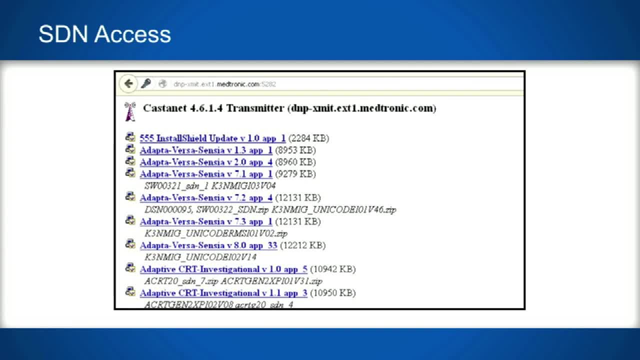 And so not only did we get access to it, we could see all the updates. If you take a really close look, we can actually see updates that are not even supposed to be in the public. Right, There's someone- There's a lot of updates in there called investigational. 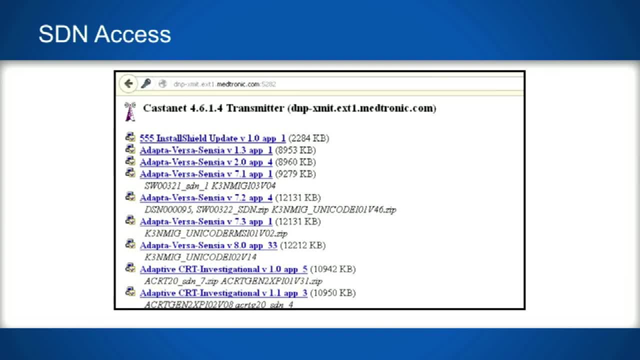 Right, Those are parts of trials, Clinical trials, Right. So there's a lot of stuff there. What are these files? Does anyone know what these files are? They're executables and MSIs. The operating system for this programmer is x86.. 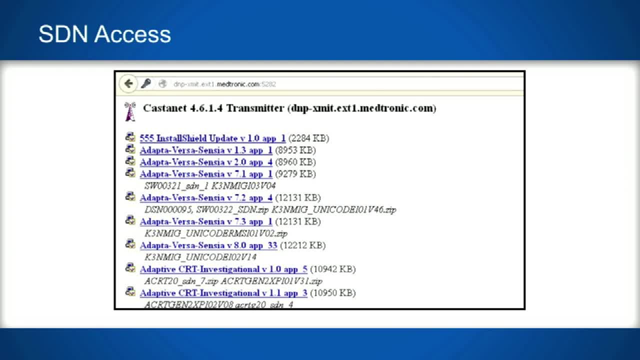 It's a really modern operating system- Windows XP, It just came out last year, or something like that- So developing malware for this program is pretty straightforward: Right x86, Windows XP, And so we're in the SDN. We can see the update infrastructure. 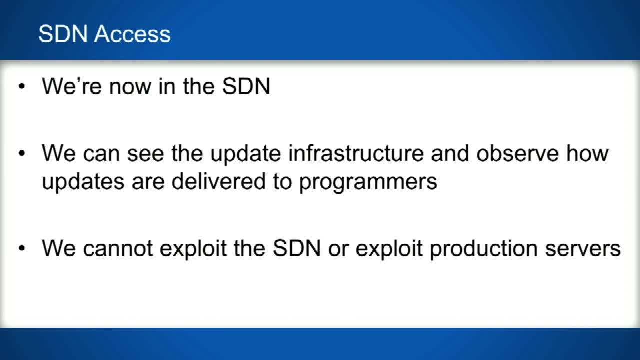 We can observe how the updates are delivered to the program. Right, We can see how the updates are delivered to the programmers, But you know what It's not like. we can just start going and attacking their production servers Because it's so protected. 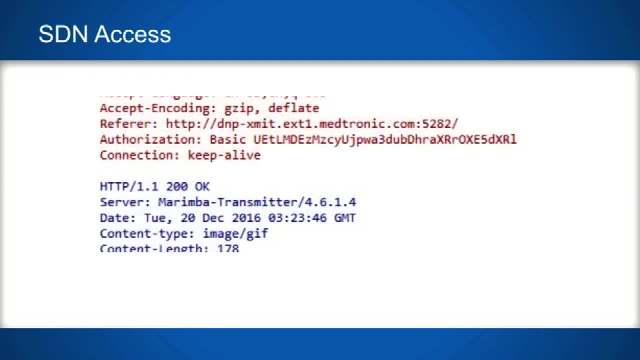 I mean, it's super secure. No, because we don't want to cross that legal boundary, Right Right. So now we can't get into their system and hack it, because then we become obvious criminals. What you can do, though, is see how the requests are done and see what the server header that gets returned is, and see exactly what version of software they're running on their server. 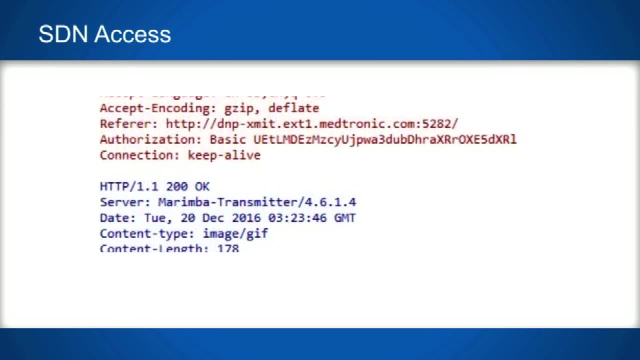 Right, This is the exact version of Marimba. they were running in 2016 when we actually did this research. Right, Like right before Christmas. I'm sure the wives were happy, Yeah, But so now we know the exact version that's running the server side software. 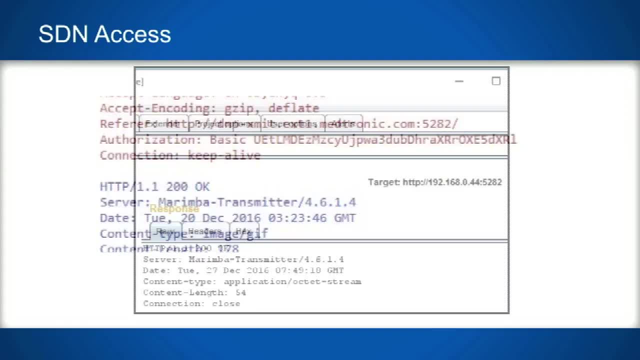 Right, And so what do we do? We go get the software and install it in our own lab, Right? And so now what you're seeing here is like burp requests that are being sent to a 192 address, which is actually our internal lab. 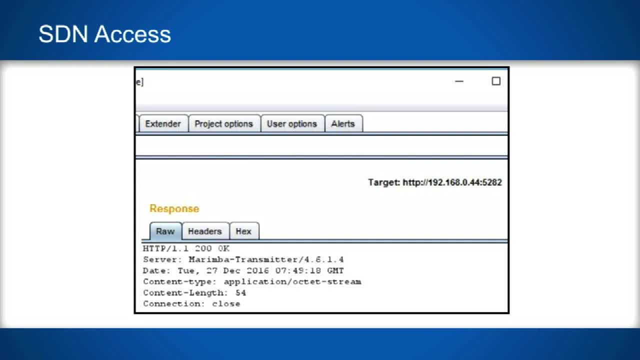 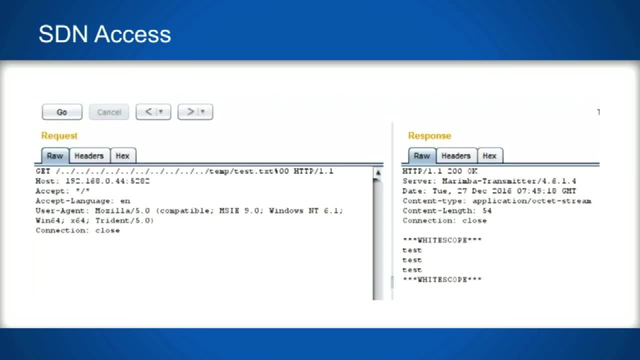 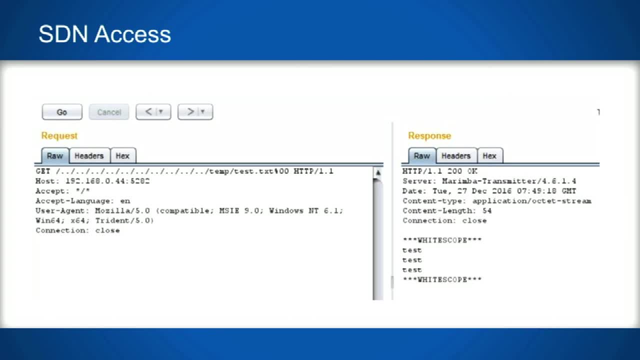 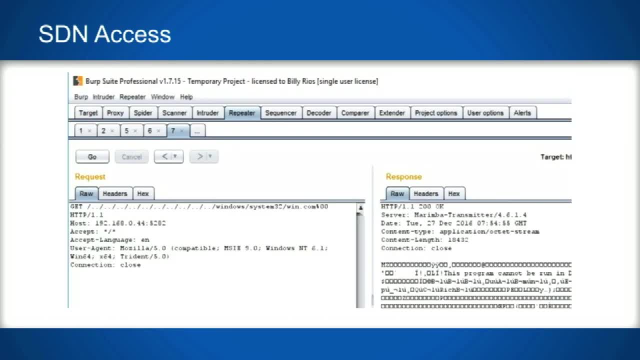 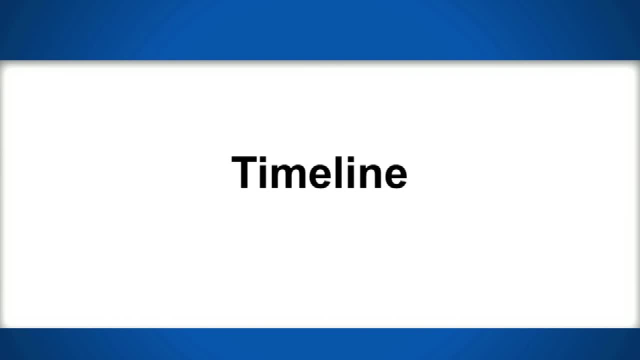 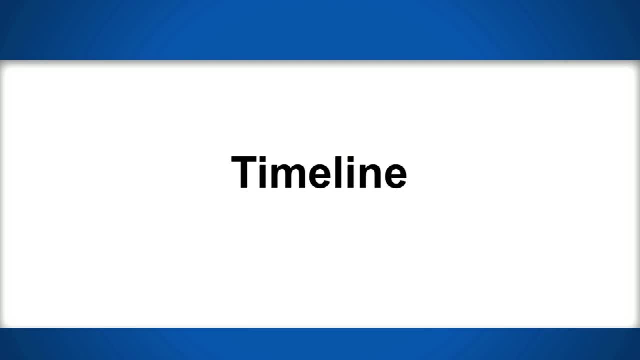 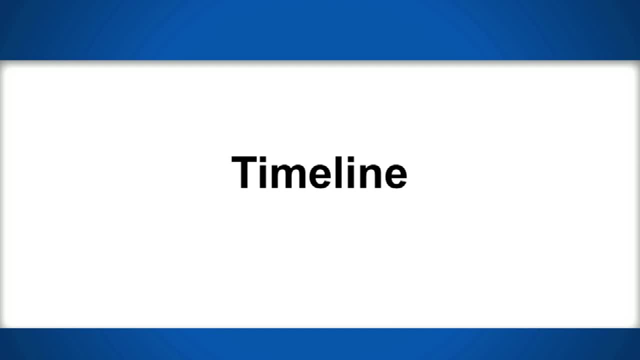 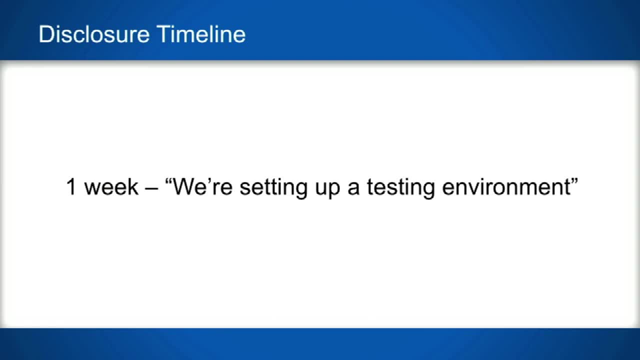 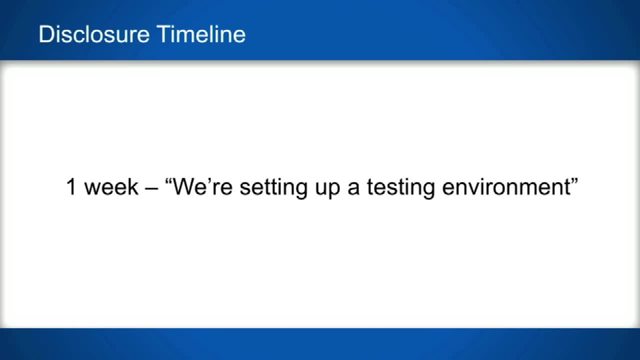 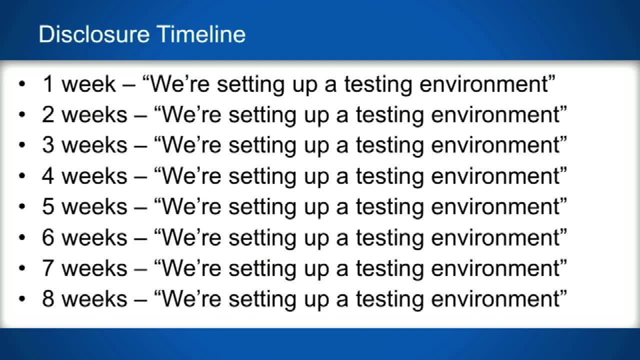 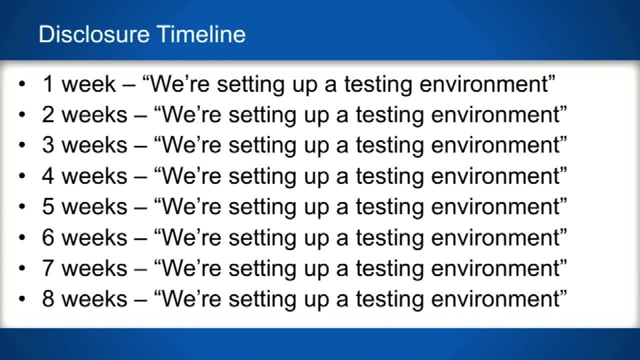 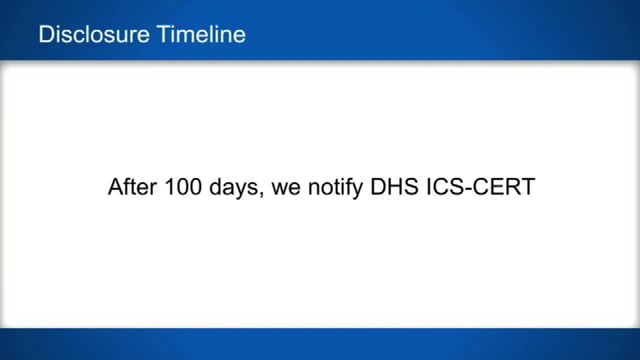 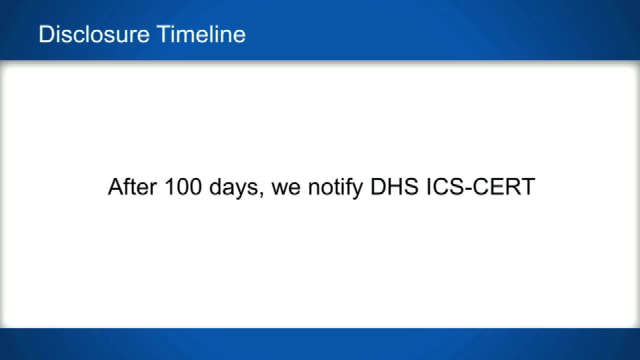 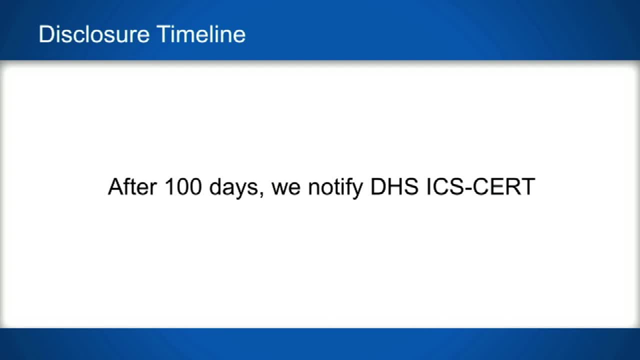 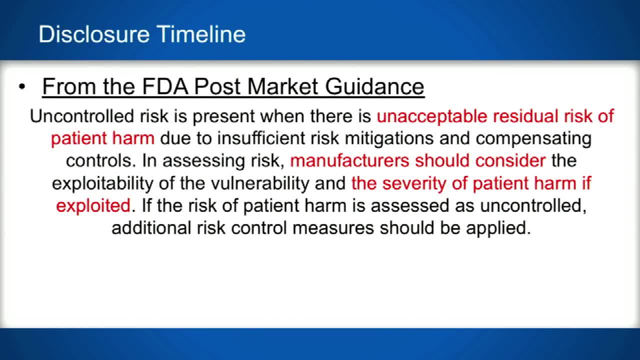 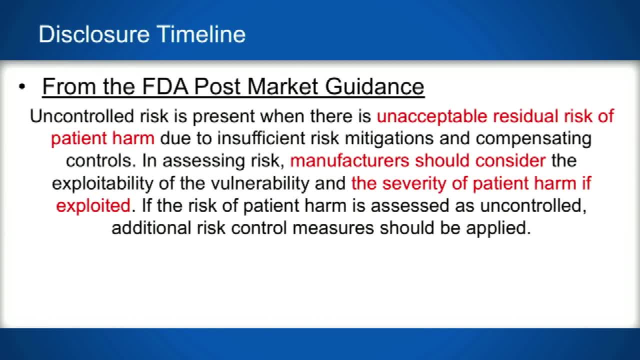 Right, It's got some pretty obvious issues. It's got some pretty obvious issues. OK, We're going to go ahead and get a couple more questions, Please, Please, One. some of the comments are that MongoDB is havering If there's unacceptable residual risk to patient. 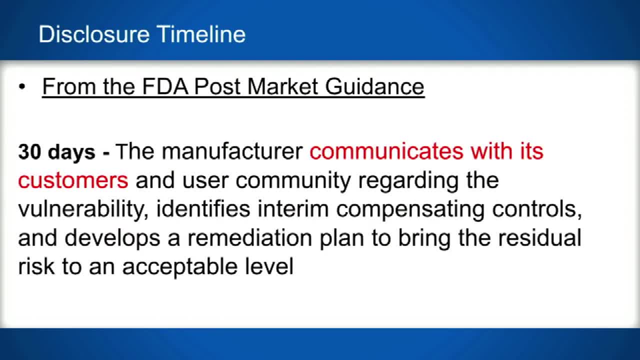 harm. what manufacturers should do is they should consider the exploitability of the vulnerability and the severity of patient harm, if exploited. So that's when we talk about the disclosure timeline of how vendors are supposed to responsibly Act, to tell their patients: You've got more to add. 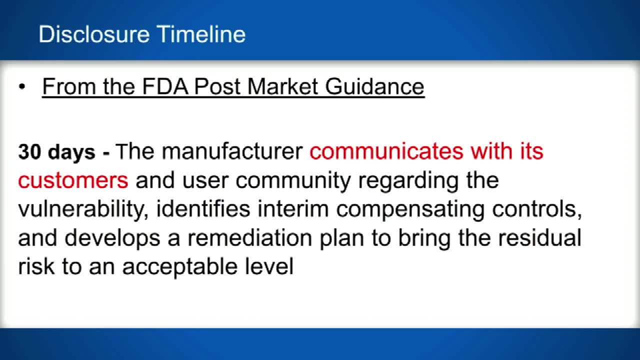 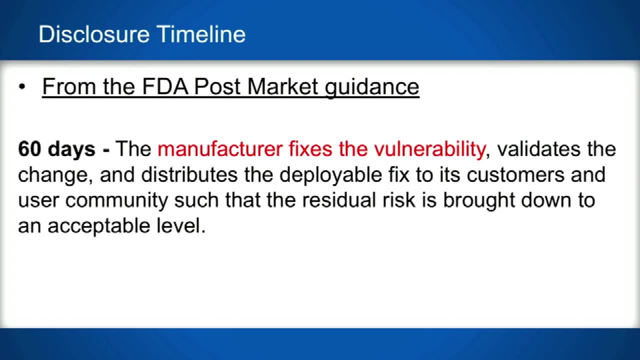 No, I think it's good. OK, So with this, at 30 days the manufacturer notification- and actually in reality there was no notification at all until we started talking about presenting a black hat. funny thing: 60 days: the manufacturer is supposed to help fit by, then fix the vulnerability if there's a. 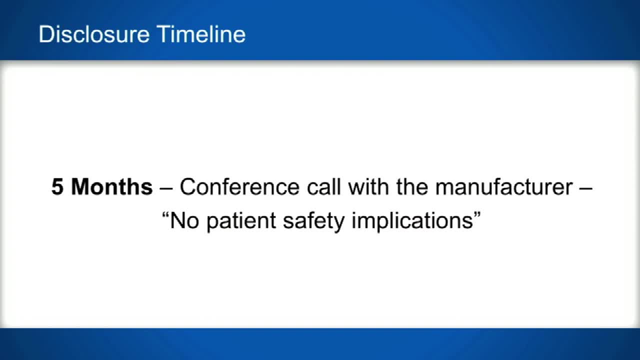 potential impact of patient safety. so at the five month mark for us now, we had another conference call with the manufacturer. this time the regulator was on the phone and they at this one this was: do you, I'm sorry, yes. so at five months they said there are no patient safety implications. so they said we 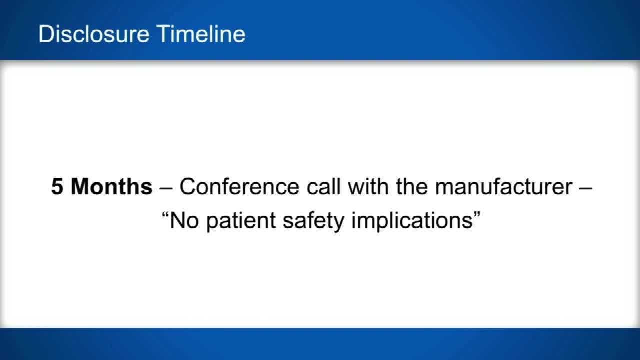 actually reproduced your research and there's no patient safety implications. yeah, yeah, so we were like man. that's kind of interesting. we have some questions about what your analysis looked like, right, and so one of the things they said is: hey, the directory that serves the software is read-only. 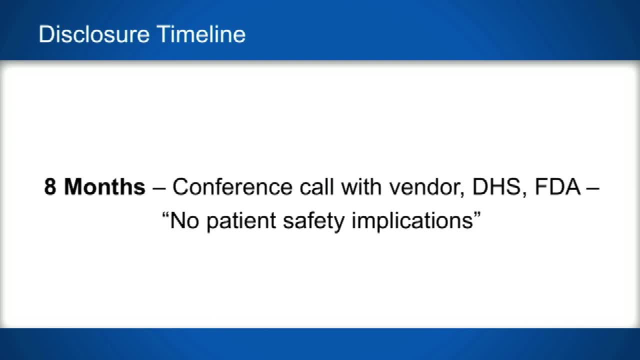 right. no one could ever write to that directory like, okay, that's pretty interesting, right, so you're the next one, it's. we're like: okay, that's, that's, that's cool. so we're like: okay, if that's what you say. that's, that's what you say. and. 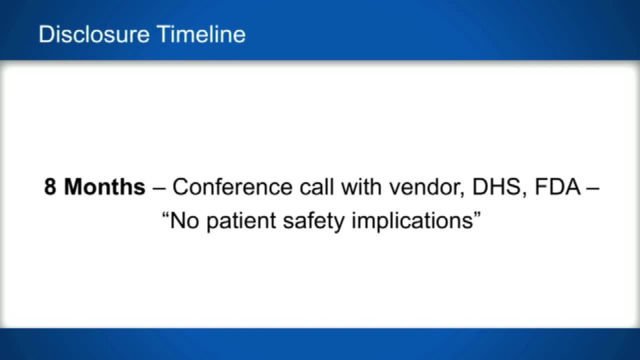 then, three months later, we had another call, and this call was with us, the vendor, you and DHS and FDA, right. So the regulator's on there and the US government's on there And basically they're telling the company like, hey, no patient safety implications, no patient safety. 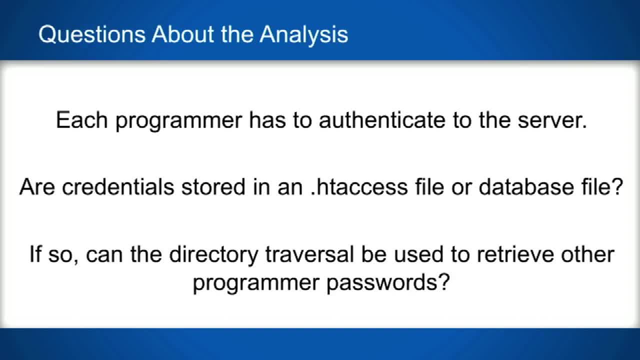 implications here, right, And so we thought that was kind of interesting. So go to the next slide here. So we started asking some questions, right, We're like, hey look, we reported directory server directory traversal vulnerability, kind of interesting vulnerability. Understand how, maybe? 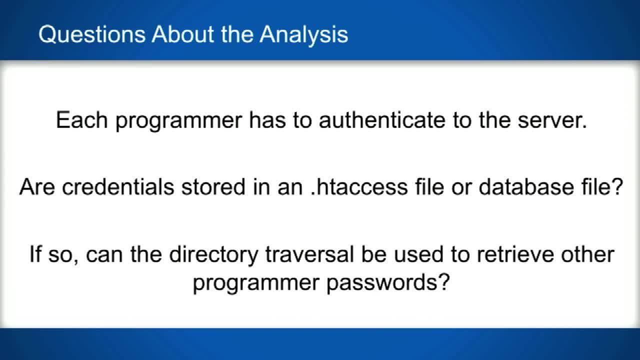 someone couldn't use this to own the server. But we're wondering if you went through these test cases Like, for example, each program authenticates to the server. right, They all have a set of VPN credentials and a web server credential. Where are those credentials stored? 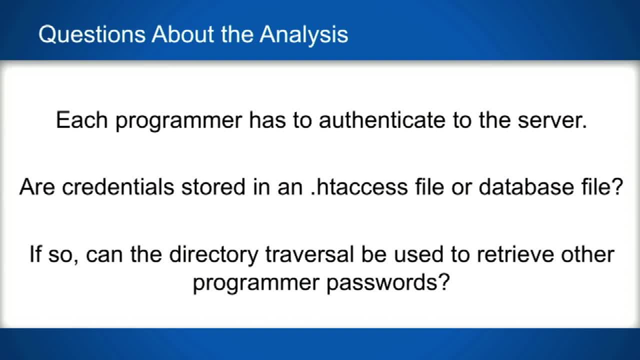 Are they stored in a file? Can this directory traversal vulnerability be used to access that file? Is it an HD access file? Is it a database file? Could we download that file right? So could we get passwords for other programmers? Legitimate questions. you would expect the. 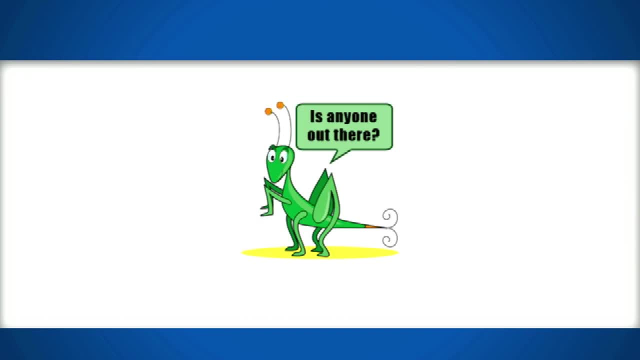 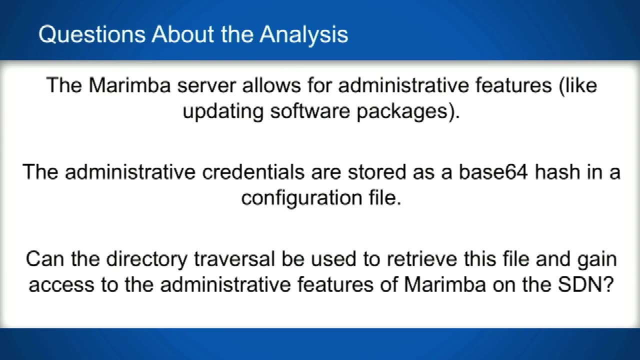 vendor engineer team and the vendor to ask themselves: Right, definitely Yeah. And this is their answer: like crickets, right, Like man, nothing right. And then so we said, hey, you know, we have this Marumba server. It's got administrative features. That's kind of neat. 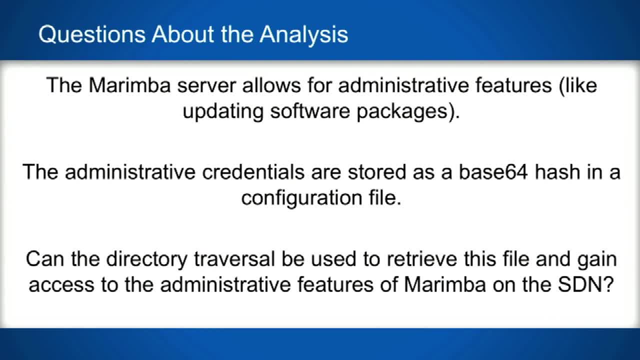 right. The administrator credentials actually store in a base 64 hash in a configuration file. We know where that configuration file is. If you have a directory server or directory traversal vulnerability, could you retrieve that Marumba configuration file and actually get the admin password and then get access to the administrative? 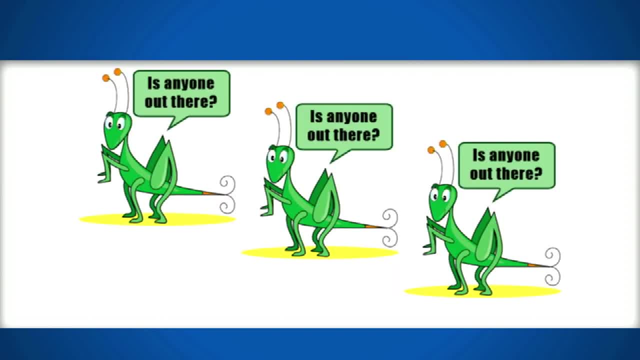 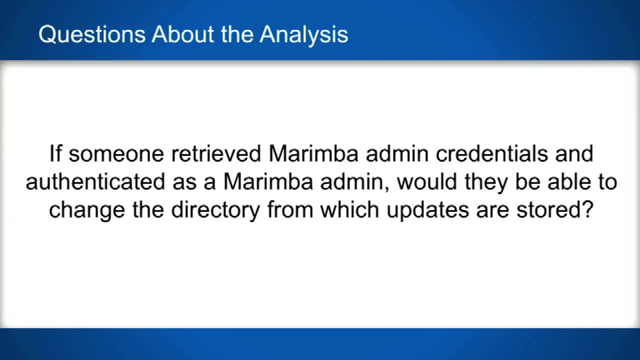 features on Marumba. Yeah, nothing, Well, crickets right. It's like: wow, okay, All right then If someone did retrieve the admin credentials from Marumba, would they be able to authenticate as an admin, And if so, could they just simply change the directory where the files? 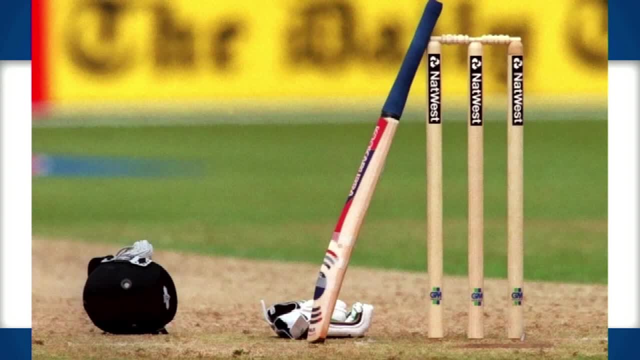 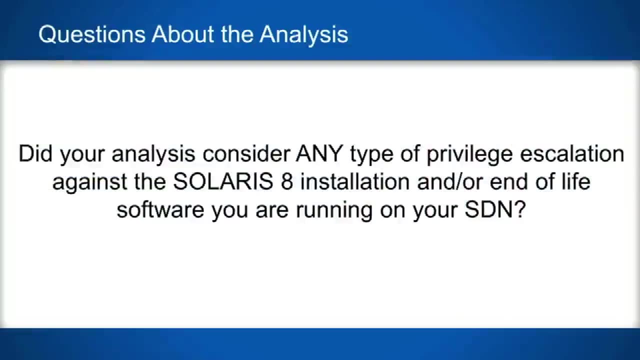 are being served from right Crickets, right. So I love cricket, by the way, But I mean, man, this is tough, right, And so, at some point though, the truth was revealed, right, So we said hey, also given that you're. 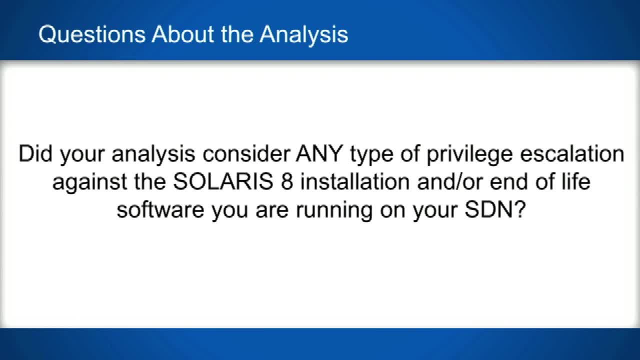 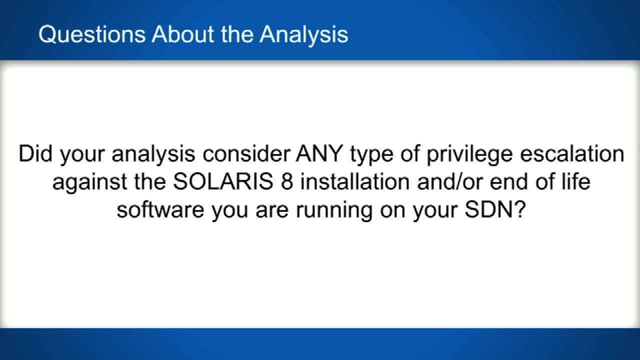 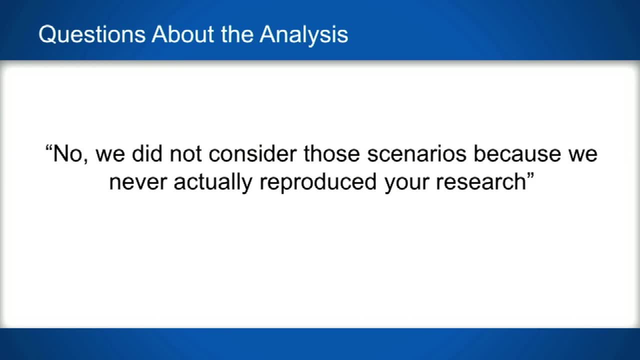 software and someone might be able to run a privilege escalation exploit against a Solaris 8 installation. And the answer was no, we didn't. And we said why not? And they said: because we actually didn't ever reproduce any of your research, right. This is eight months later. 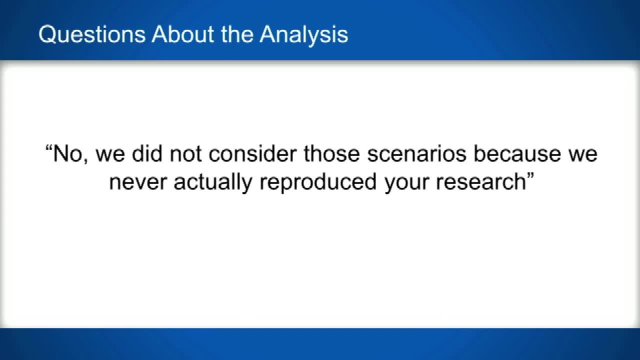 Eight months After we had a call with the regulators and DHS to where they told them there are no patient safety research. So our frustrations again. I know we're a little frustrated up here, but this is ridiculous. Come on, Yeah, You know. Crazy, right. 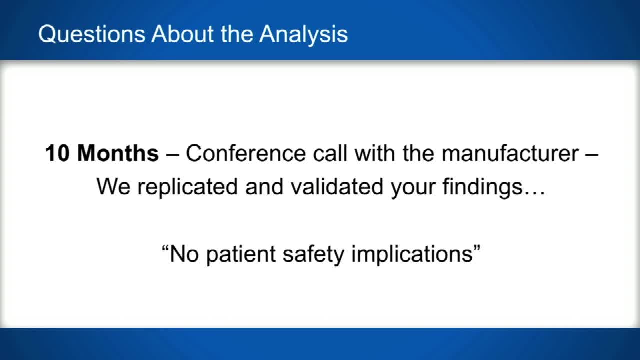 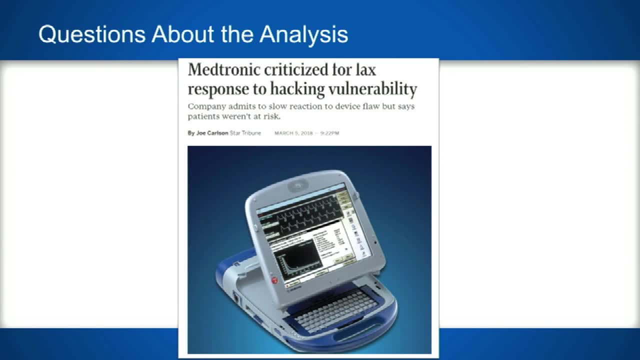 So two months later they're like: oh hey, you know what, We did actually replicate your findings, but hey, there's no patient safety implications, right? So there is actually an advisory that went out for some of these bugs And when that advisory went out, someone actually 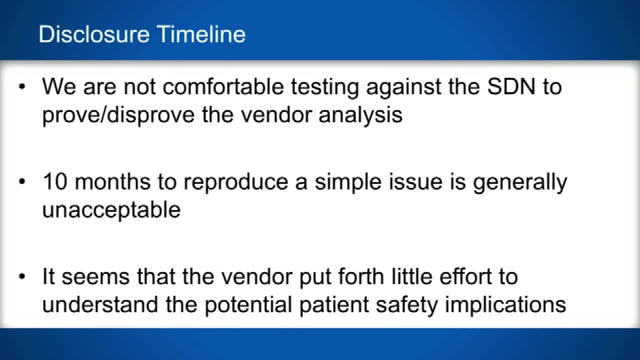 wrote this article, right. We'll come back to this article here in a second. So not comfortable testing interest, right? So we can't really prove or disprove that specific attack scenario. But to be honest, even if their analysis is true, ten months of analysis time is probably two. 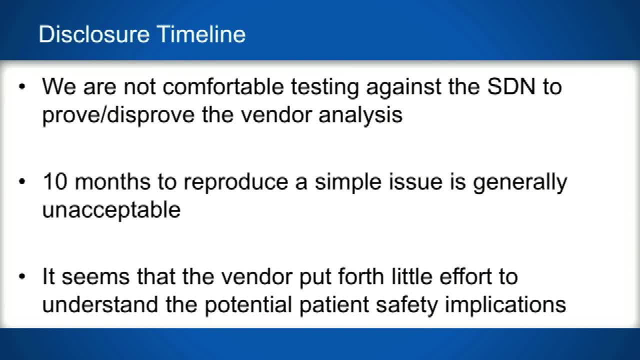 long, especially considering that the impact if that server does get compromised is what Every patient could have their therapy altered, right So, and it seems like they put forth little effort to kind of understand all the various implications, So want to talk about this. 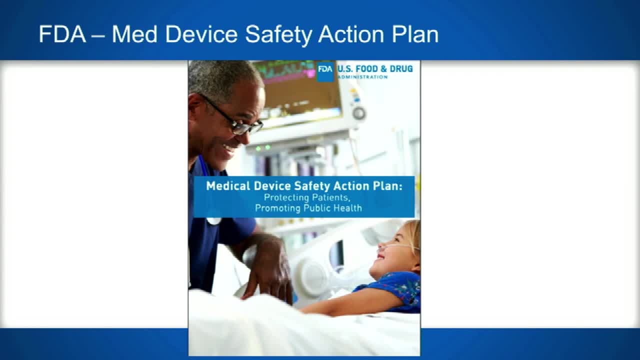 one, Yeah, And so one of the things that again we were working with FDA on this and we've reported, as we mentioned, plenty of vulnerabilities before. Working with the vendors is something we actually enjoy. This has just been so painful, But working with the FDA kind of one. 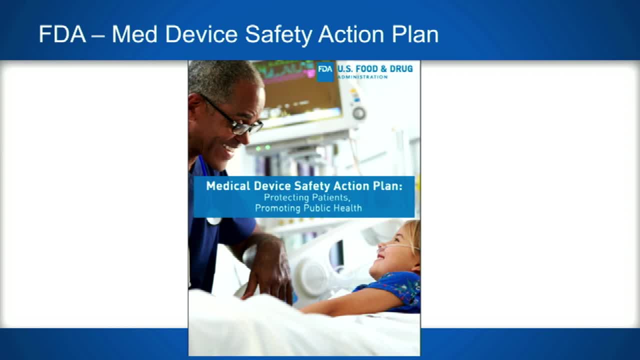 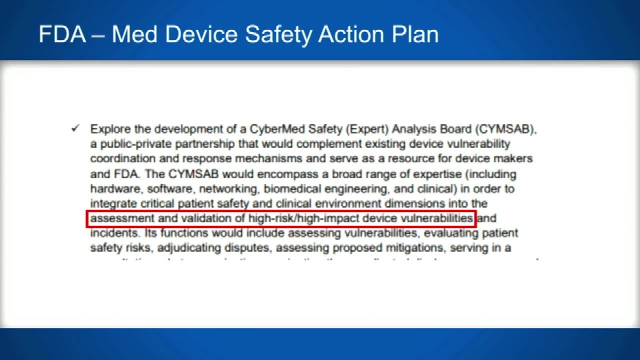 of the things that they've done is: they've done a lot of work on this. They've done a lot of work on this. What they have for leaning forward with is this analysis board that they're standing up, And so part of this is to help avoid issues like this, And this is going to be the part where they 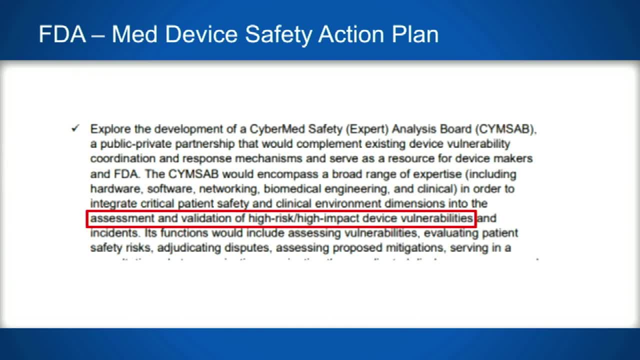 actually have researchers and physicians, clinicians across the industry that will help vet these problems. Because that's one of the issues is, you have the vendor saying one thing, you have the researcher saying another. We're both vested. We're both vested in one way or another, And so 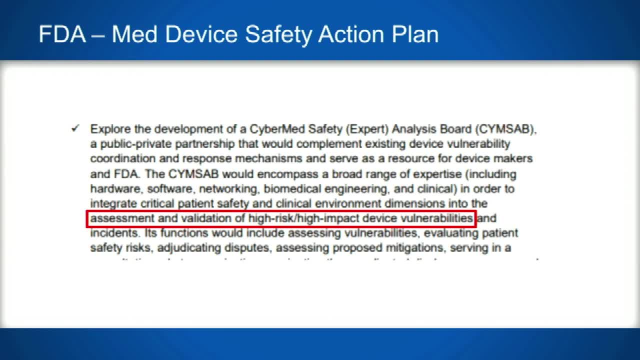 how does the regulator weed through this to actually make sure they're making smart decisions And, more importantly, the way that they're doing it is they're doing it in a way that they're one thing missing out of all this whole thing we did. There's no physicians ever involved in the 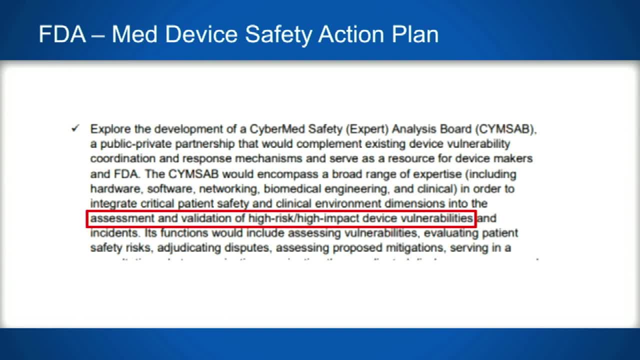 discussions right, There's no doctors, There's no cyber researchers in the vendor, And so how do we pull that together to where? if you're a physician and you see those ICS certs that go out or the advisories that go out, how do you react to that? How are you supposed to react? It doesn't. 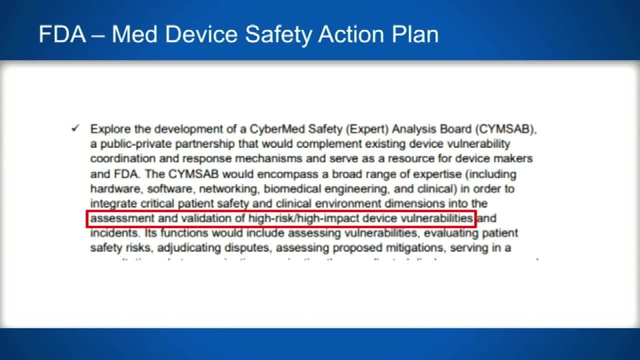 mean anything, And so how do we get that messaging more clear and better to the physicians so that they can make informed decisions? And people ask us. the number one question we've gotten since we've been here is: um, you know what's your motivation behind this and, simply put, is as: 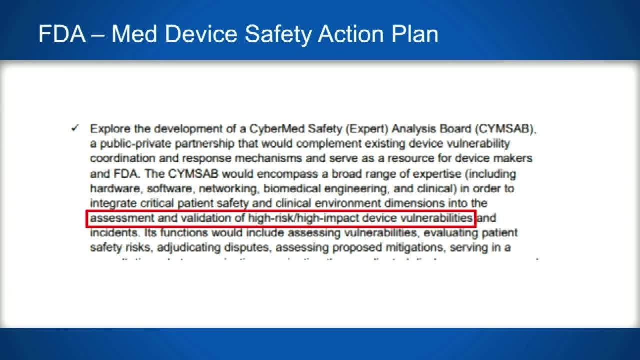 i mentioned, we're not financially invested. we don't. nobody's paying us to do this. um, man, we've. when we first started this, i remember reading an article about a father talking about his son. and what do i? what am i supposed to do? because he's relying on this for care for life. 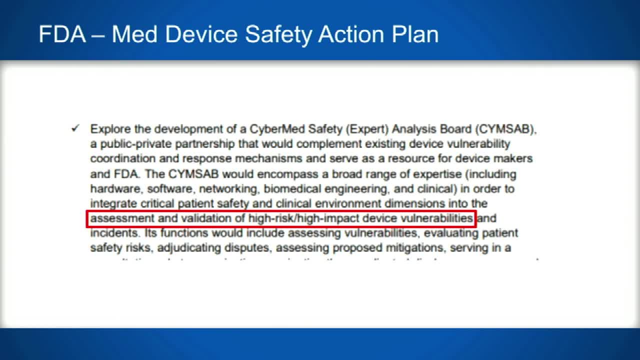 support. you know, and this it really just frustrates us when a vendor has the ability to spend a little bit of money to fix this and do the right thing and instead they spend more time, you know, trying to control the message. and it's an easy fix and it's and we proved, we demonstrated the security. 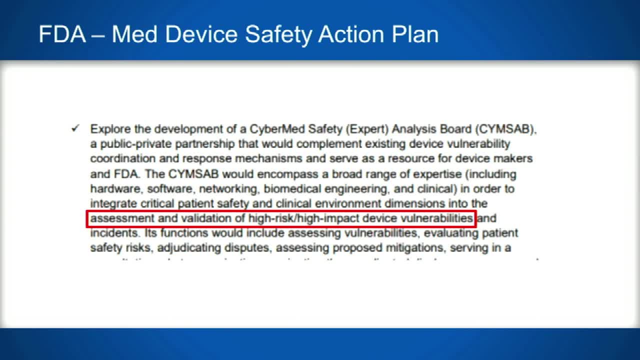 concerns with it. uh, so that's that's really our motivation. that's why we're here today is, um? they've issued this statements that they're not going to fix these vulnerabilities. they have said they're not patching it. um, let's see what happens after our black hat talk right when the 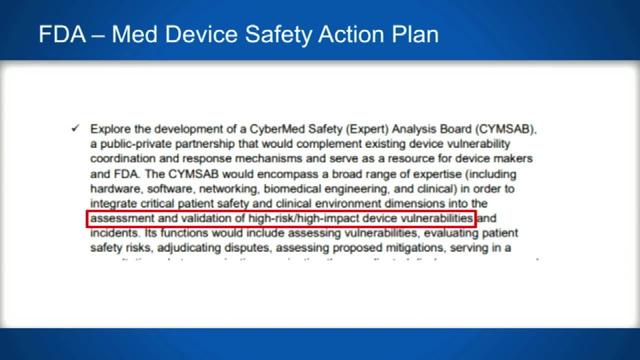 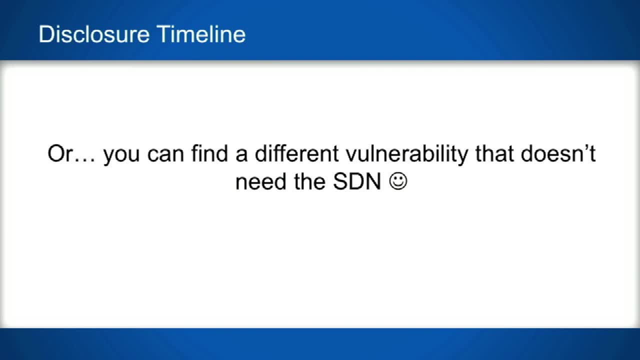 pressure comes on them, that's i have a feeling they're going to be fixing this thing. i hope so. i hope so because it's it's. it's unfortunate, all right. so, um, i wish we could, on stage, exploit their software delivery network and show how you could take over someone's pacemaker remotely. uh, obviously we can't do. 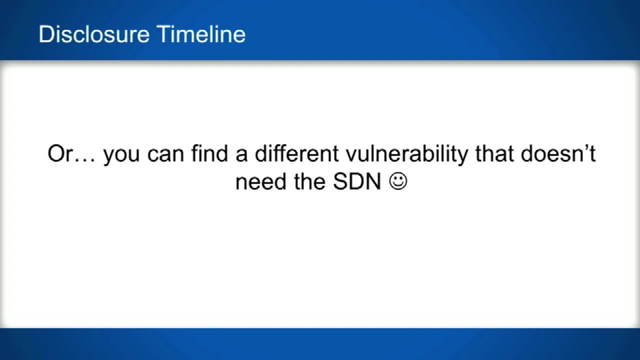 that. so, uh, but what we can do is find a different vulnerability that leverages the same weakness, or different exploit that leverages the same weakness, and show that, and so that's what we're going to show, right? so, because we already mentioned to you how the delivery mechanism works, there's vpn. 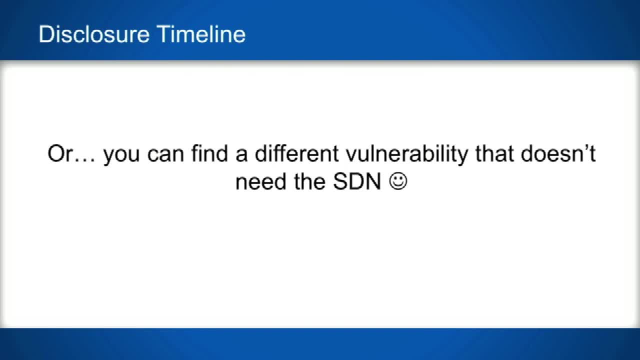 the vpn joins. once you're joined onto the vpn, it authenticates, indicates in some specific ways and then it downloads the update over what HTTP right And then it does what Runs it because the software is not signed, So anyone can literally serve. 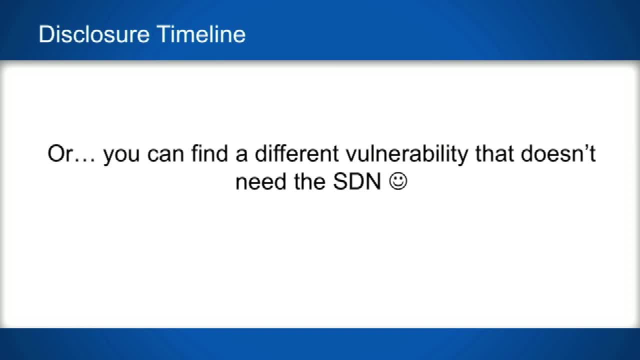 back. if they can get the right timing and exploit or whatever, they can actually just serve back an executable and the program is going to run it right. So that's what we're going to show you. We're going to show you how that works. There's already advisory for this. 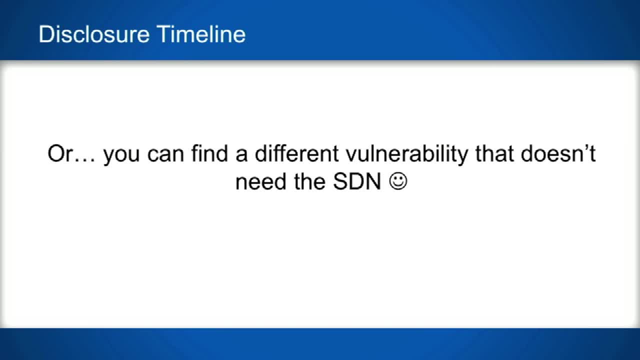 Essentially, I'm going to kind of describe to you how it works and then we're going to show you how it works. Essentially, what happens is because the actual retrieval mechanism is very insecure over HTTP and unsigned code. they're just strictly relying on that VPN right to 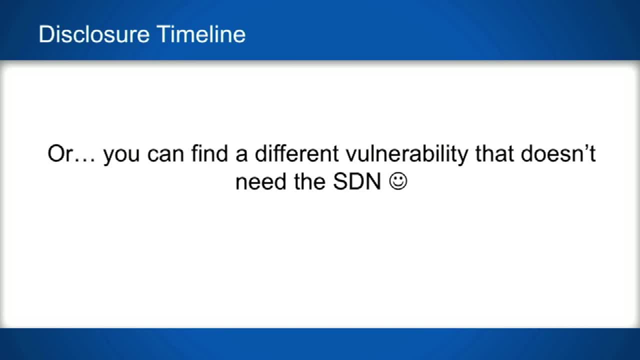 provide all the security for them. And so if you can convince the programmer that it's actually on the VPN, when it's not what happens, It sends an HTTP request to a random server on the internet. basically, And if you can position yourself to say, hey, I'm that server, you should. 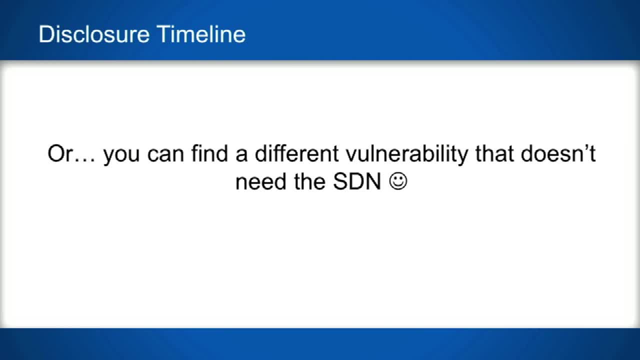 run this executable. that's what the programmer is going to do, right? So we'll show you how to do this, if you're on a local network, what it would look like when this thing gets exploited, And so I don't know if you've heard of that. I don't know if you've heard of that. 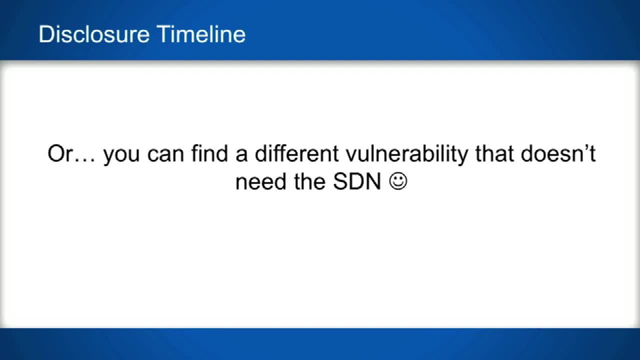 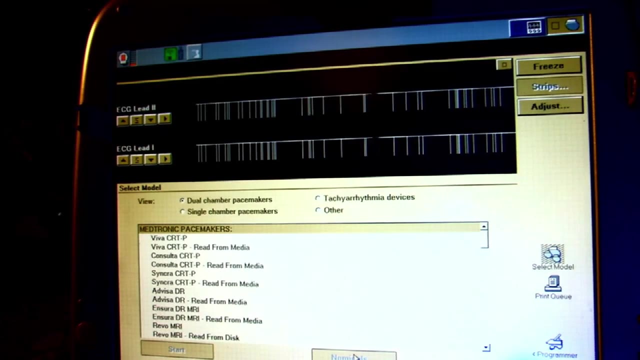 You can switch the screen back to here. Let's see if we can get this thing set up here. Can you switch to this little camera here? Perfect, All right. So this is the pacemaker programmer interface And so you can see at the top if this were actually implanted in someone. 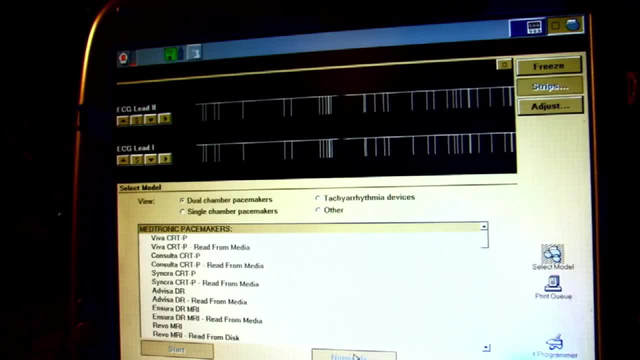 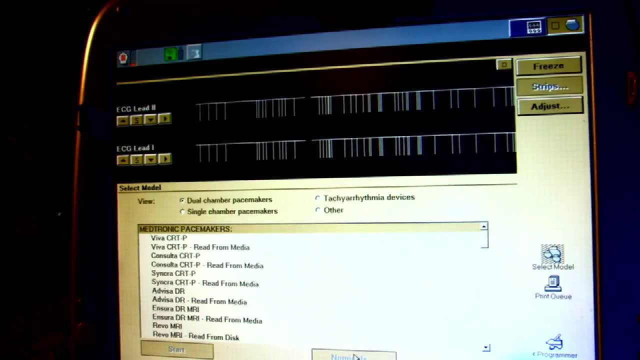 you would actually see the pacing occurring up there, right? It would be feedback from the actual device itself, And so this programmer was going to try to like: join the network, join a VPN and download software, right. So but this thing is already exploited And we want to. 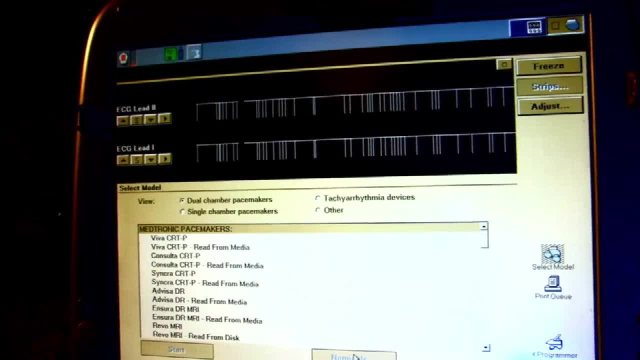 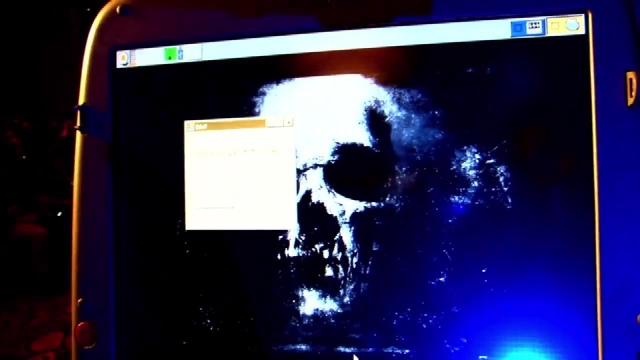 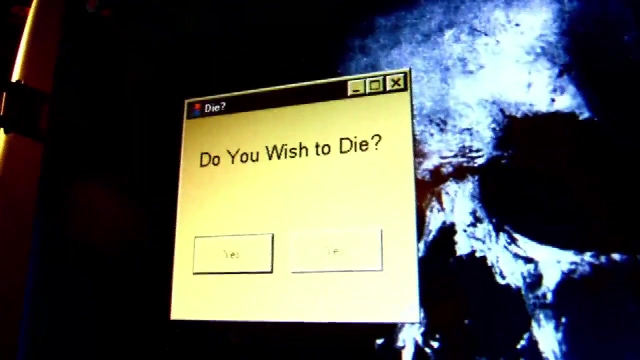 show you what an exploited programmer looks like, right? So one of the things we talked about. well, we'll let you, Okay, a second here, All right? So I mean you're going to ask a really simple question here, So like: 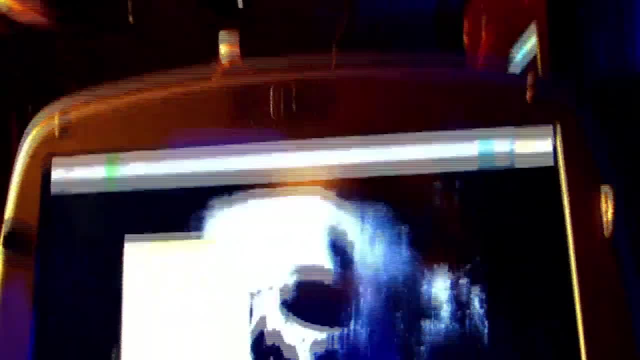 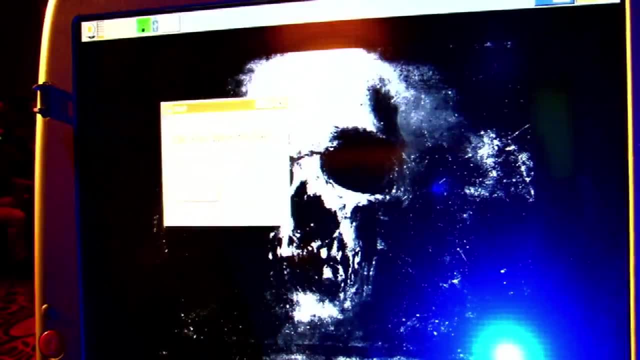 And then, if you look at the answers, right, So we've been asked some questions like Billy Jonathan, why would you do that? right? And it's like when you read that advisory- and I recommend everyone go read the advisory for this- When you read the advisory, we'll show you. 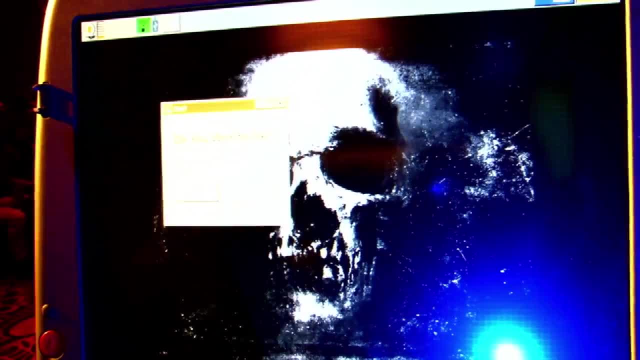 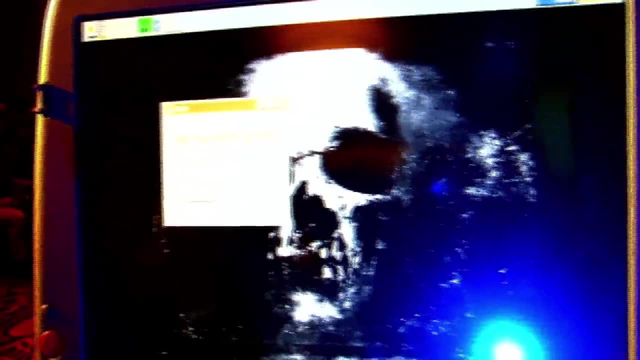 some language from the advisory It's almost impossible to understand what the real risks are right. But I think when you see this you start to understand what the risks are right And if you realize that this thing programs these things, maybe it makes a little bit more sense. 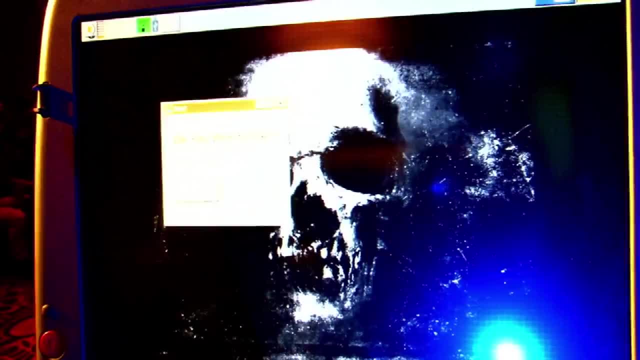 Right. So that's why we did this. We had another thing that we were going to do, but, Yeah, we got talked out. One of the problems is with the pacemaking. it's difficult to see our code running on this right, Because we can hold it up and say our code's on here. This gives a 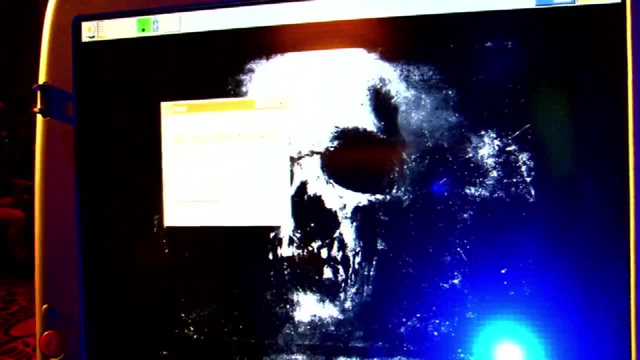 better display of that We had. actually we're coordinating with Black Hat. we were going to bring a pig on stage and shock the pig, but we kind of cooler heads, smarter heads prevailed. Primarily, we didn't know what we were going to do with the carcass afterwards, the livestock carcass. 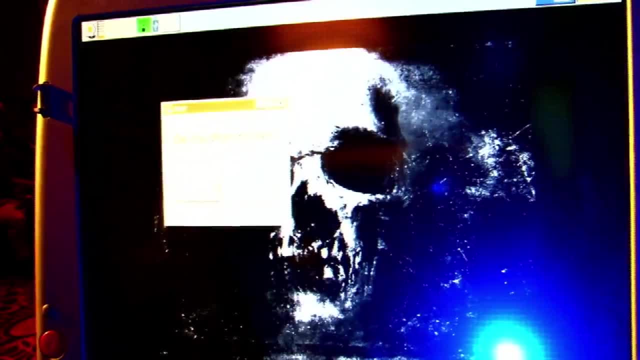 here, So we decided to go this route instead, But we have demonstrated the ability to actually just change the code to initiate shock when we want, And there's two pieces of this. One is the sensationalism of we can just shock it when we want. That's concerning right, But actually. 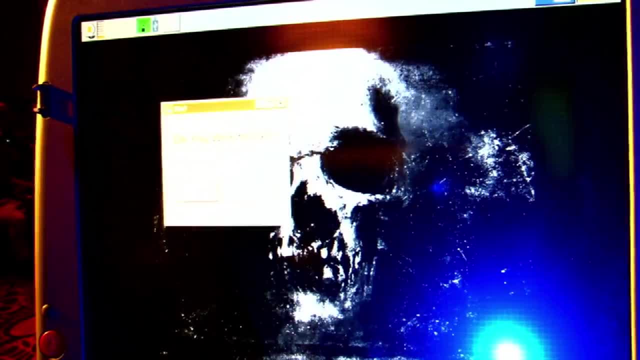 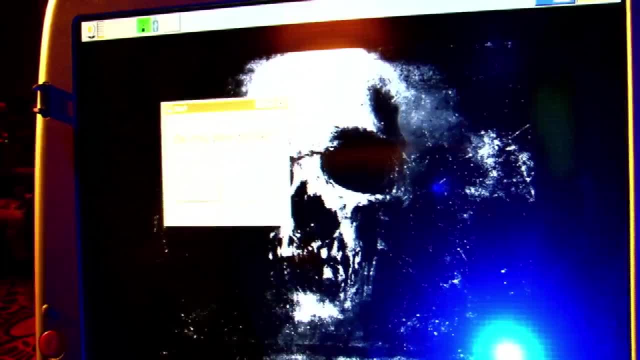 exploit there. Uh, we want to make. We did a live demo work. they worked. right Yeah, They worked, Thanks. Measuring risk: right Yeah, A Google drive, Measuring risk of a Google drive. Alright, Can we go back three slides if we could? Alright, So um a couple. 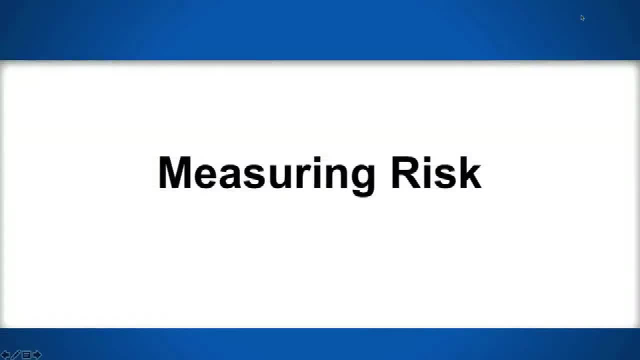 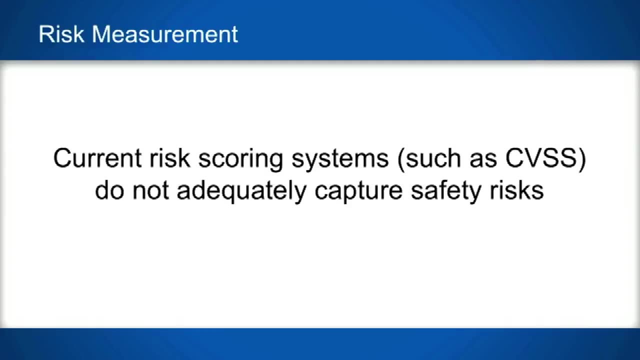 different things here, right, And we go to click in, Alright. So, uh, if you're going to use something like CVSS- which for some reason the defender was like, Oh, this CVSS was really low, right? So, uh, we want to make sure that's not a test. that's really low, right. So, uh, we. 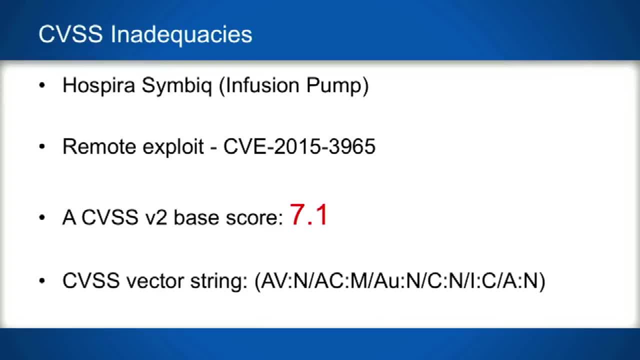 want to make sure that that's not a permite that you been watching dogs on TV once or three appropriate way to measure patient safety risk, right. So example: CVE 2015-3965, that's research that we're involved with. That was a HOSPERA Cymbic Infusion Pump. If you look at the advisory 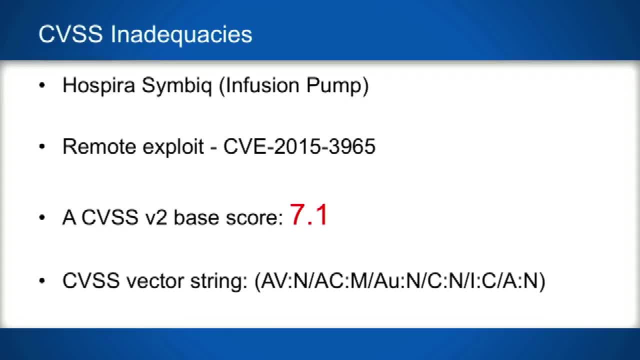 for that that has a CVSS score of 7.1. Pretty respectable score, right. So we also did some other research on something called a PIXIS Supply Cabinet. The PIXIS Supply Cabinet essentially holds supplies right, And so that actually has a score of 9.7.. If you look at the technical 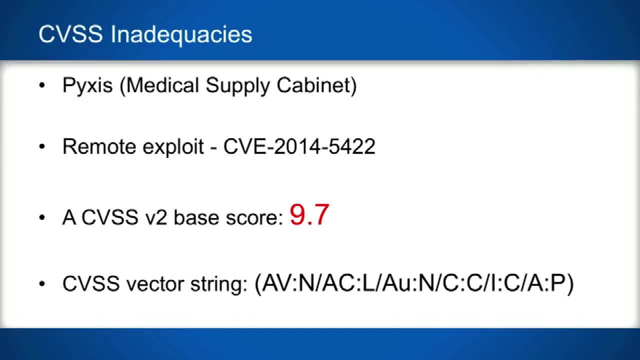 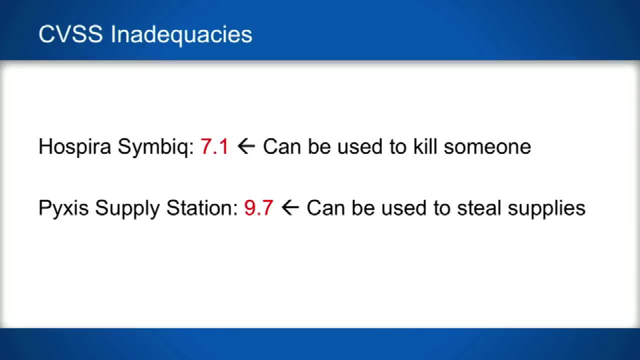 details. vulnerability is actually really really similar. So, but that one score that has a 7.1, that could be used to kill someone And the one that's a 9.7 could be used to steal supplies, right. So CVSS really falls down when you're trying to understand patient safety implications. 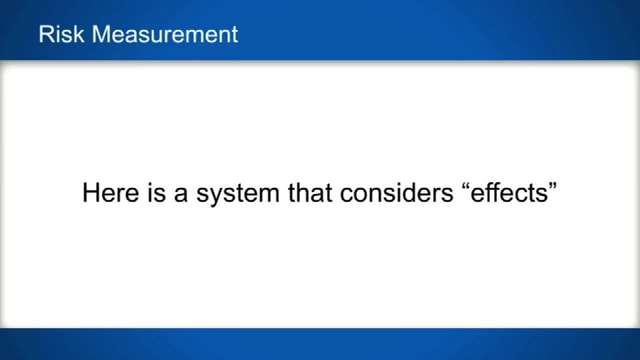 and things like that. So here's a system that considers effects. Want to go over this? Yeah. So we actually working with some vendors. this was their frustration too, because they want to measure actual risk and they have to report that up in certain situations, And so we kind of 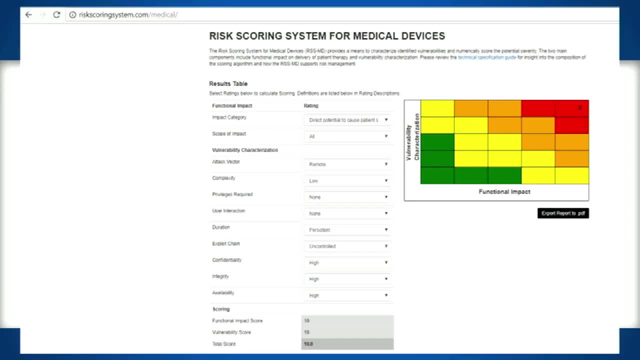 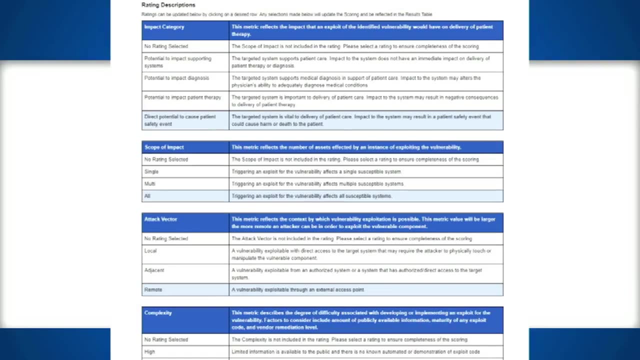 came up with this Just a risk scoring system. You can go check it out and punch in things as you want, And it actually considers the impact to patient health, And so you're actually putting it in the context of what does this have an impact to patient therapy, the delivery of patient therapy, Is it? 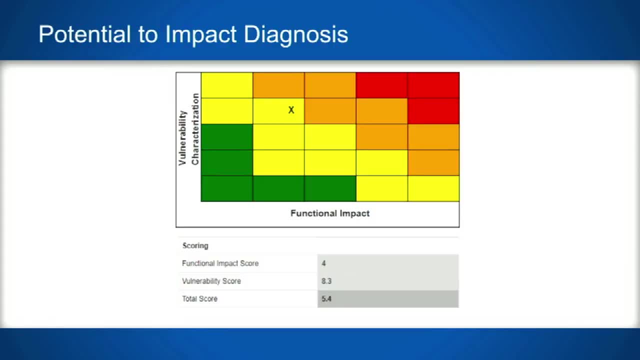 a diagnosis impact, And so it actually puts those into context. And so when you run these down, you know the similar implications you can actually see. it'll actually put that into context, And so we like to just kind of point that out. as it's, I don't know if we had the website there. 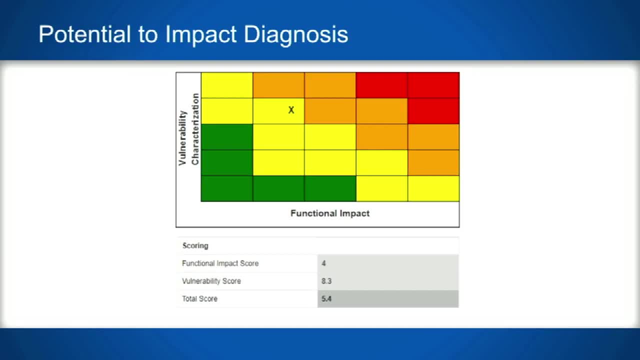 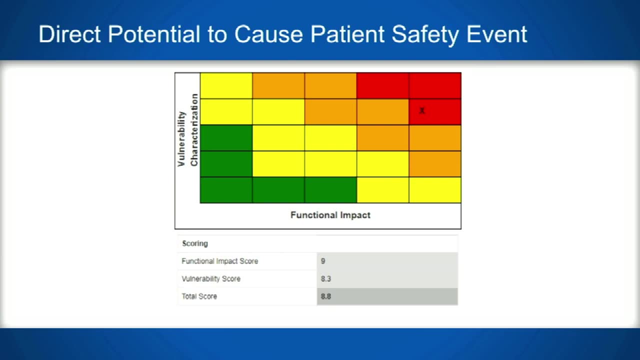 for that or not. So here's the one, the same two. we saw Potential impact diagnosis versus potential to cause patient safety event and how it impacts on the severity of that. There it is, Yeah, So that's up and running. Feel free to give us feedback. 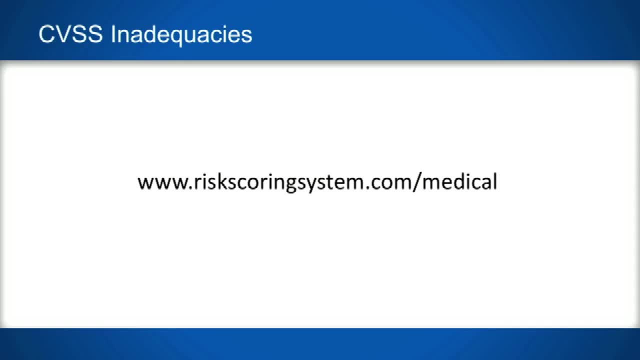 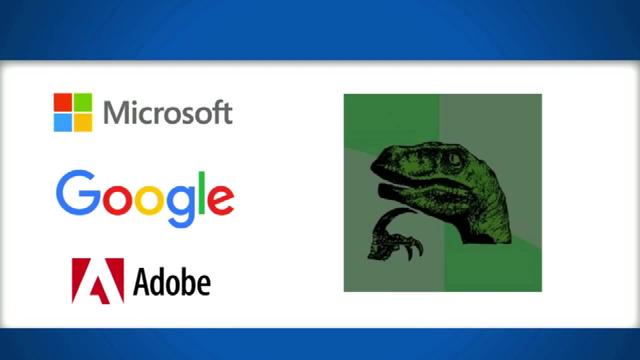 Yeah, It's all client side, So if you want to take a look at exactly how that calculation is being done, definitely take a look. All right, So kind of on a closing note, one of the things that we find interesting is Microsoft. 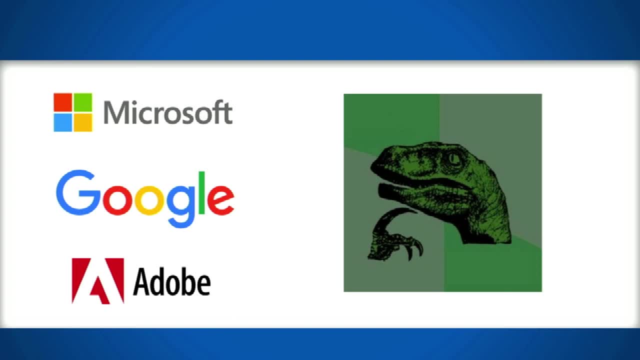 there's a vulnerability in their software delivery network for pushing updates. You think it's going to take 18 months for them to push a patch or to repro or patch it. That's probably a couple. well, you used to work at Microsoft. I mean, you used to work at Google. 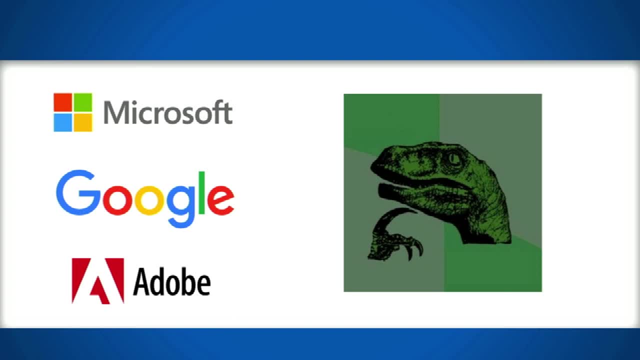 So it's frustrating. It's interesting- frustrating how we want to position it- that from our general IT systems- boy, the patch systems, they've got it down. The varying analysis. if you're, as a researcher, if you report something to one of these organizations. 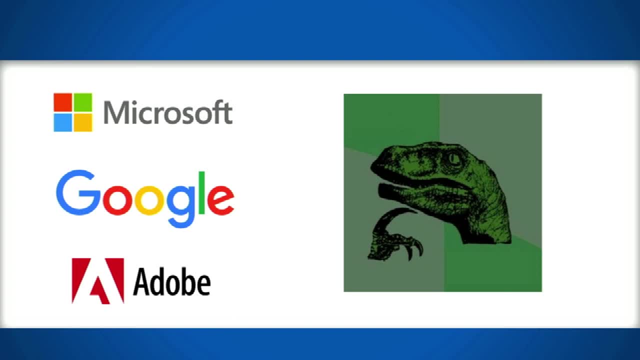 they're going to put a team on it and do varying analysis that says, okay, what else in our code similar to that is exposed? Or is there other products that we're presenting that have similar vulnerabilities that we need to take a care and look at? But when it comes to a device that actually 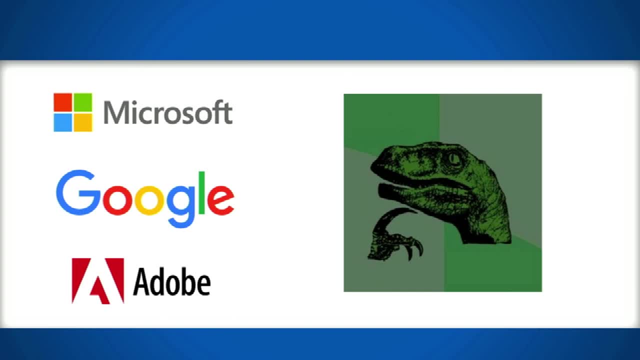 administers patient care. it's 18 months. They just released a memo saying they're not going to fix it. They're actually going to rely on the hospitals. Boy, could you imagine Microsoft saying: well, we've got a bug, but just put a firewall in? 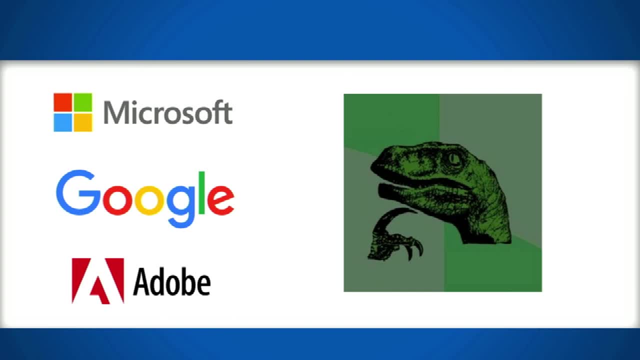 Yeah, there's a bug. There's a bug in Exchange, but, man, you know, it's not remote, It's just over the network. Yeah, So we want the culture to change on that. I think it is moving that way And again. 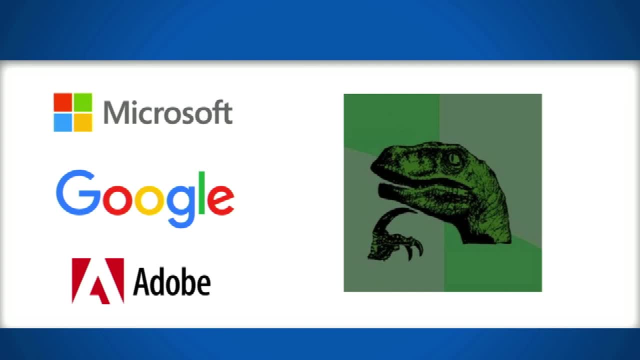 we work with a lot of vendors, and there are most vendors out there who are trying to do the right thing, And so we don't want to paint a broad brush on that. But it's frustrating and I think the industry has a long ways to go, especially when we're sitting here. 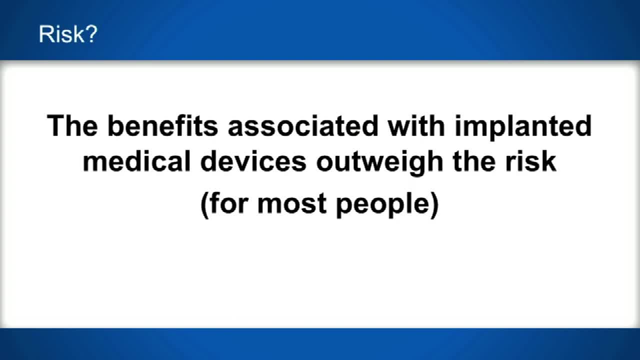 Definitely. Yeah, I think that's about it Once again. hey look, the benefits probably in most cases, for most people probably outweigh it, Right? So if I go to the craps table and I slip and fall and hit my head and I have to go to the 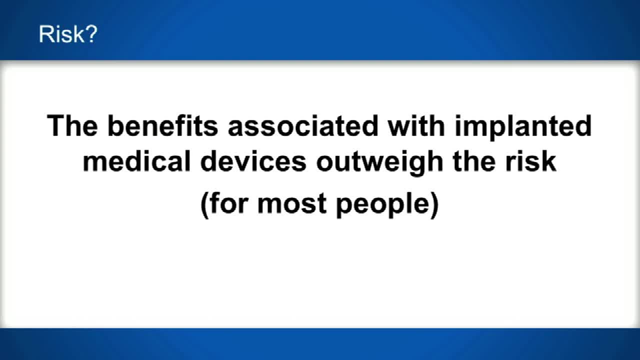 emergency room. I probably want to be connected to a medical device And I'm a researcher, right. And the bugs? obviously things are going to have bugs, right So. but what we can't control is the way that we react and respond to those. All right, So I think we've got time for a couple. 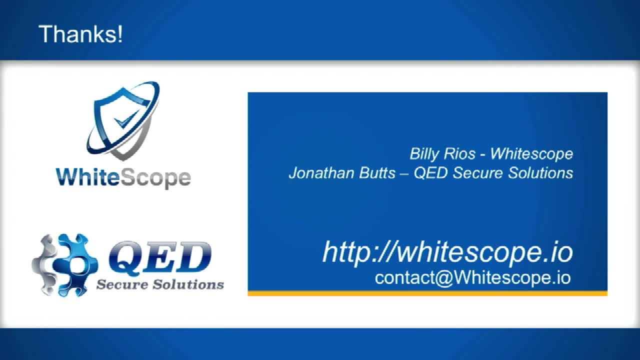 questions. Yeah, I think someone from the FDA is here. if there's questions for the FDA- So like we're not going to answer regulatory questions or anything like that- but they're here to talk about it, And if there's any questions about the technical pieces, we'll be happy to answer that. 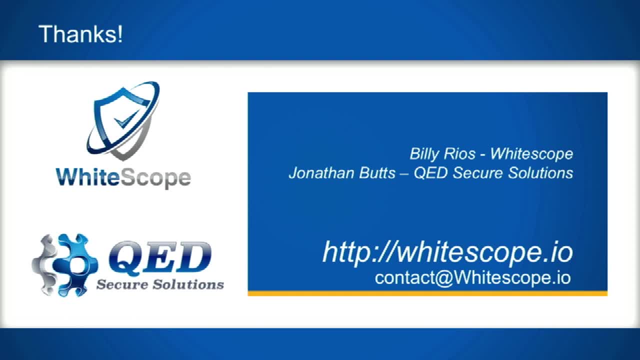 Thanks for coming. everyone Appreciate it. Thank you. We have one question here, So I'm Suzanne Schwartz from the FDA and I first of all want to applaud the work that you've done, Billy and Jonathan. you've been really extraordinary partners for the FDA. 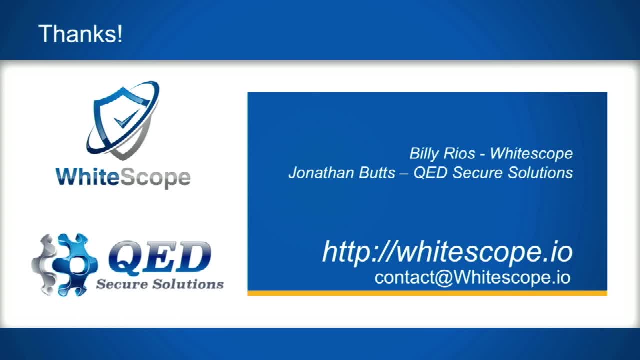 In moving and advancing the state of cybersecurity. I think that this case is illustrative of the need for greater partnership and greater work across the independent security research community and the medical device community and government as well. So we want to encourage that kind of. 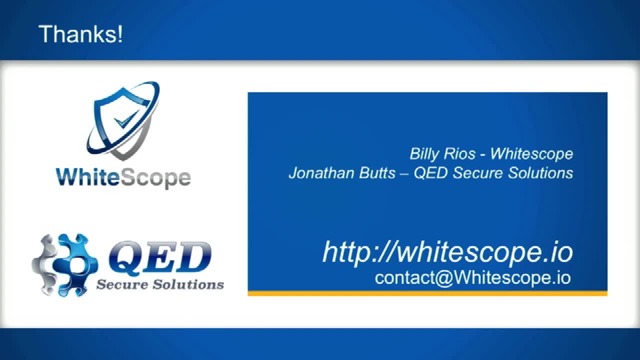 partnership, and we also are very excited about the future of cybersecurity, So I think that's going to be something that we need to be talking about for some time. Thank you, Thank you, So I've got a little bit more time left to talk about the prospects of standing up the 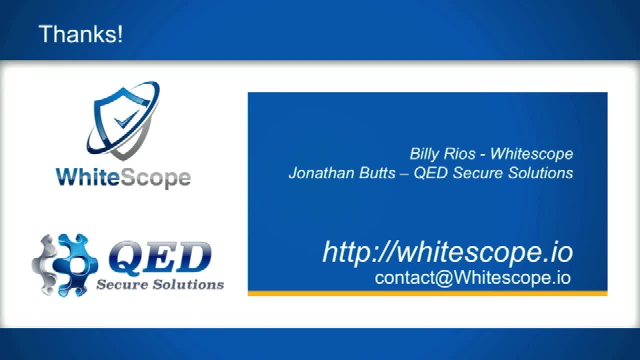 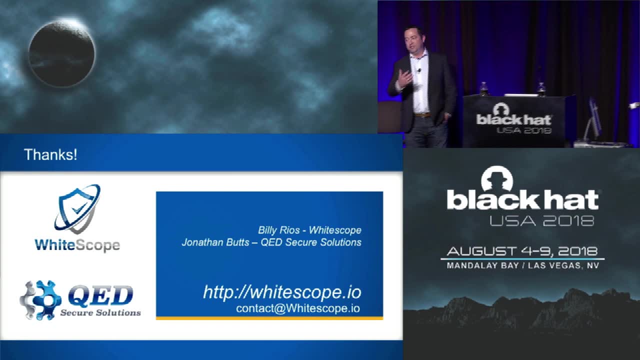 SIMSAAB that you highlighted in this live presentation. So thank you, Yeah, Thanks, Suzanne. Thank you, Suzanne. Yeah, Appreciate that And, as we mentioned, we know, as researchers, sometimes working with regulatory bodies isn't always easy but, to FDA's credit, they've got a lot of challenges but they will, you know. 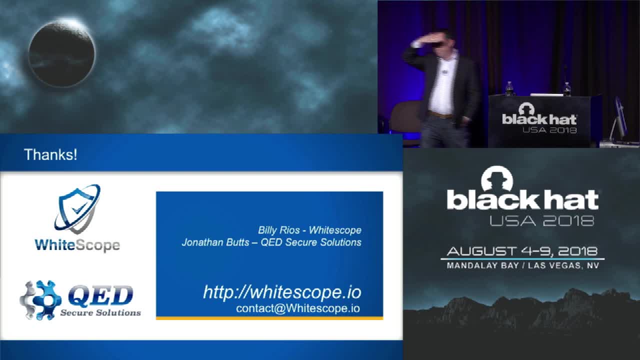 I appreciate that they're working with us. Any other questions? I don't know. Yes, Yes, ma'am, I'm actually here as a mom. Hi, Hi, Hi Hi. I saw in your abstract that one of the devices you were looking at was a. 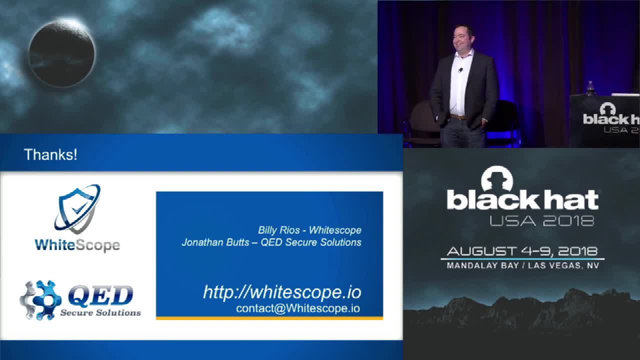 neurostimulator? Yes, And I know you didn't have time to get to that because you were irritated with Medtronics and I understand that. Can you reassure me that Nuvectra is responsive? Yeah, so we don't have enough time to cover everything that we looked at. 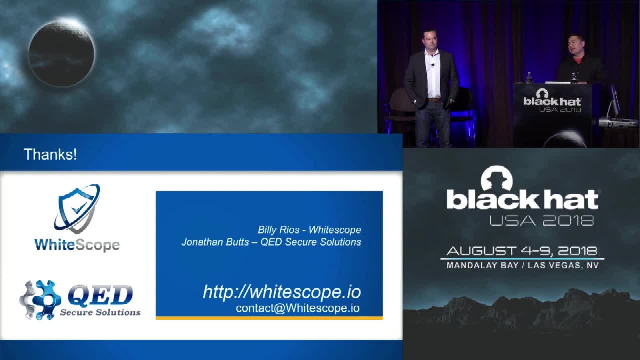 There's actually a DHS advisory on some of the issues that we discovered in a neurostimulator programmer, And we also have a deep brain stimulator programmer as well And we have an Activa PC. So I'm sure if you're interested in specifically that stuff we can. 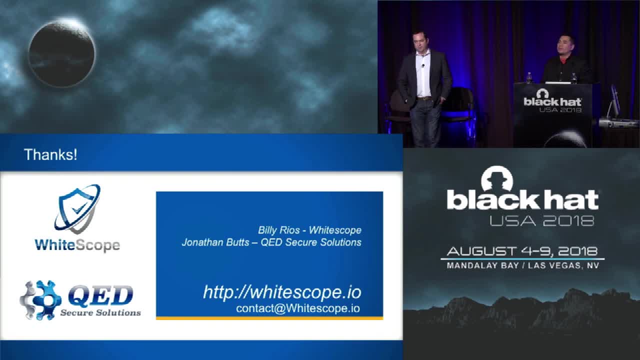 maybe chat with you afterwards about what we've seen in the neurostimulator world. For those that don't know, the neurostimulators work very closely like a pacemaker. It's an implanted device but instead of connecting to your heart, it connects to your brain or your spine.